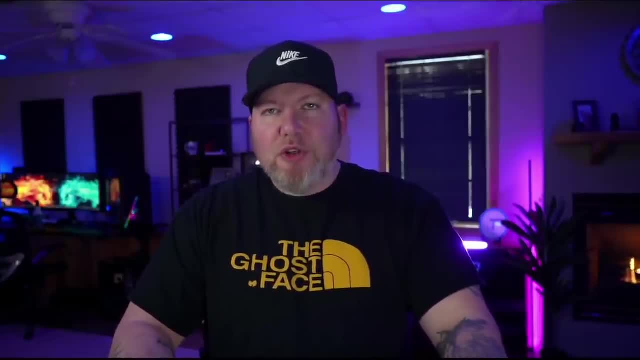 Hey, what's going on guys? So in my opinion, every web developer should learn CSS Grid, at least if you're working in the front end. And in this CSS Grid crash course, we're going to break it into a couple different parts, So first we're going to look at some 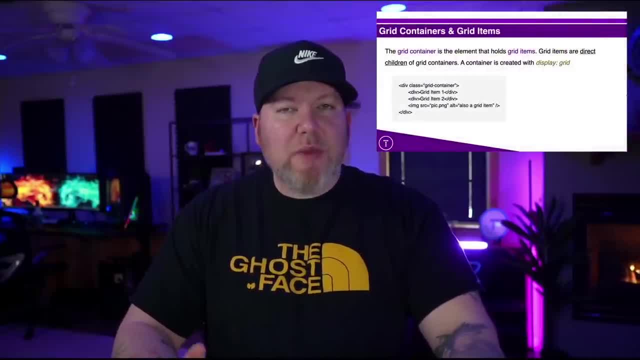 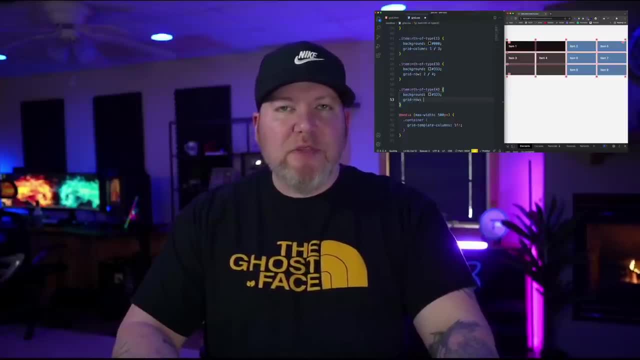 slides just talk about what CSS Grid is. We'll compare it a little bit to Flexbox. Then we're going to jump into a sandbox where we look at all the different CSS properties that we can use on grid containers and grid items. learn how to span rows and columns and 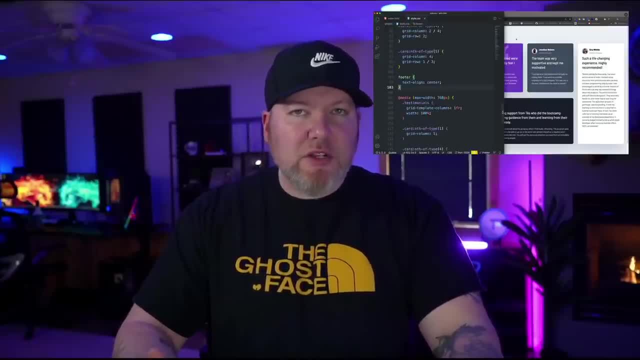 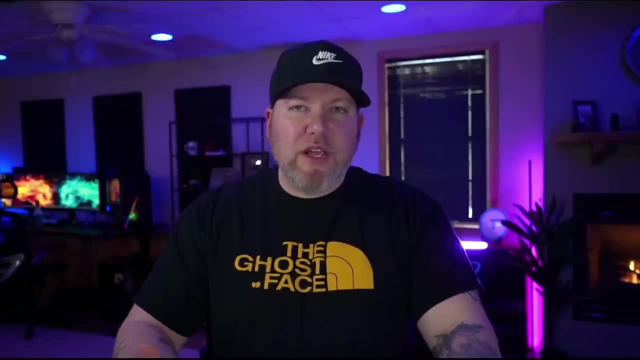 things like that. And then, finally, we're going to build a small project which is going to be a testimonial landing page. All right, so I think that this will give you a lot of foundational knowledge in creating layouts with the grid, So hopefully you enjoy it and let's get into it. 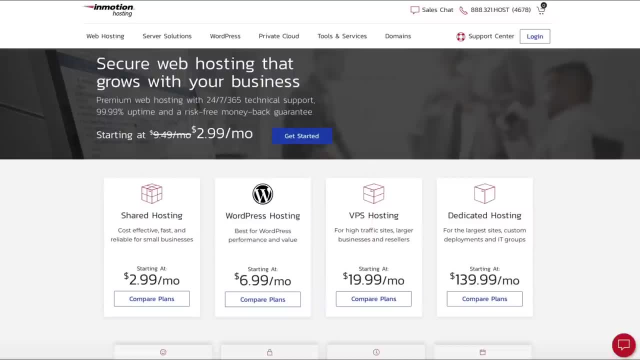 This Grid Crash Course is sponsored by InMotion Hosting, and I've used InMotion personally for years. In fact, my TraverseyMediacom website is hosted on one of their VPSs, So they offer everything from shared hosting and WordPress. hosting for small businesses to VPSs and dedicated servers, And I can speak from experience that their service is fast, secure and reliable and great for just about any project. So you have accounts starting from just $2.99 per month, and that includes not only web hosting but email. 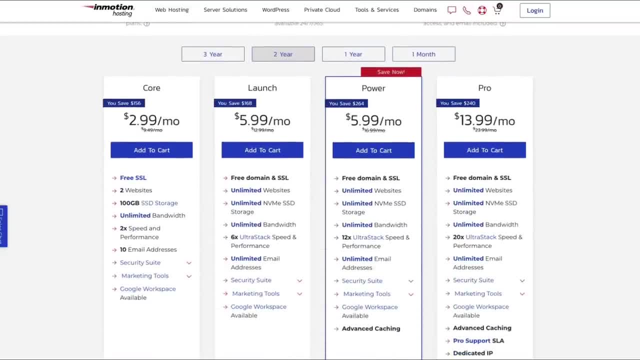 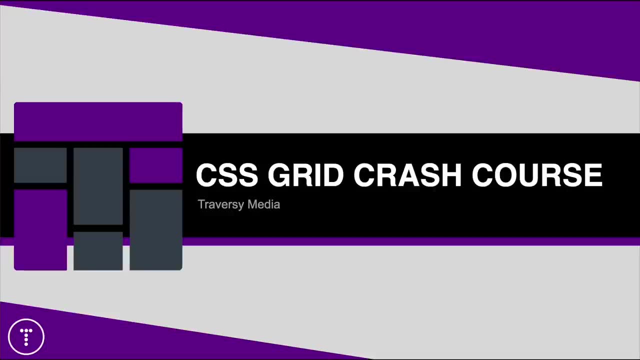 accounts, marketing tools, free SSLs and more So. to learn more, visit InMotionHostingcom or click the link in the description below. All right guys. so I just want to jump into some slides real quick to talk a little bit about what 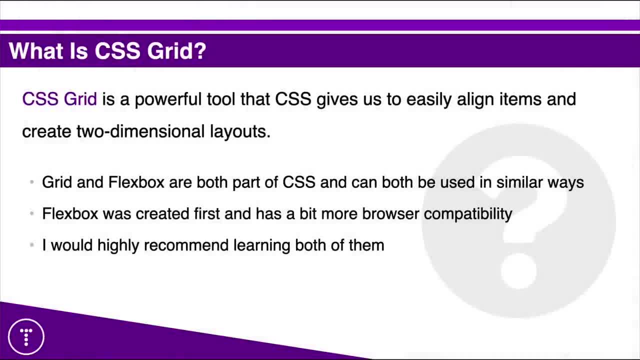 CSS Grid is. So the Grid is a powerful tool. that CSS gives us to easily align elements or items on the page, create two-dimensional layouts with rows and columns- And I do want to mention Flexbox here, because they can be similar. They are used a lot in similar ways And a lot of people ask me which. 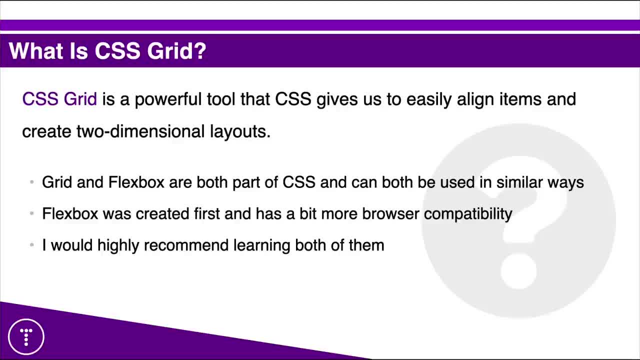 one they should learn, or if they should learn both, And my answer is always to learn both. Now, Flexbox was created first. It has a bit more browser compatibility, But if you're using modern browsers, you're not going to have any issues with either of these. Now it's going. 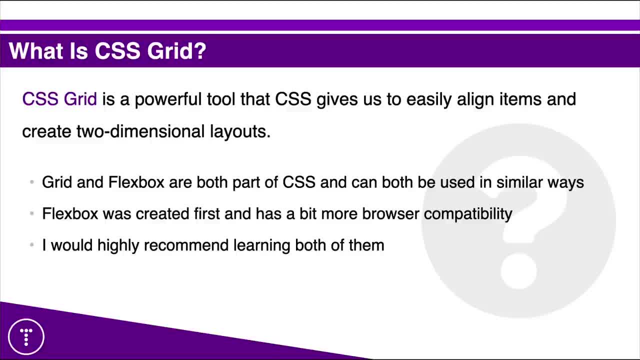 to come down to preference on where and when you use Grid or Flexbox. So I can just tell you what I do. So what I do is I use CSS Grid for the overall layout of a website or a user interface, So laying out headers and cards and all that stuff. 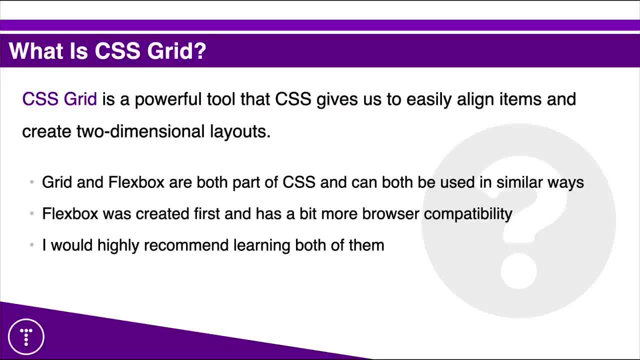 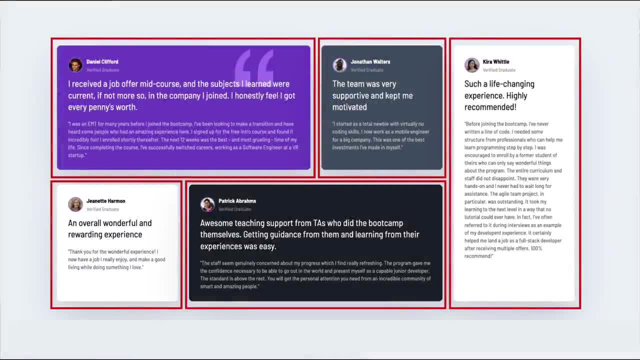 And then if there's inner elements that need to be aligned, that's where I'll use Flexbox, So I may have a layout of cards that I use with. you know, I'll use CSS Grid And then if there is maybe a header in the card, 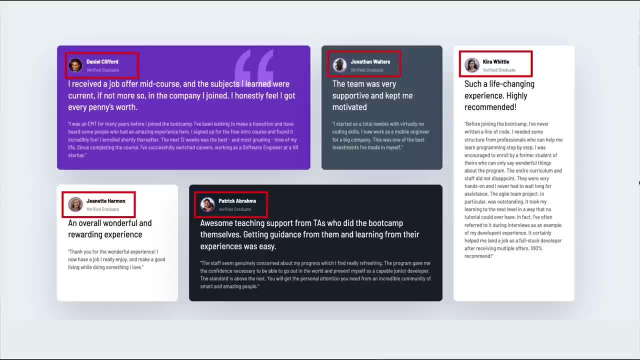 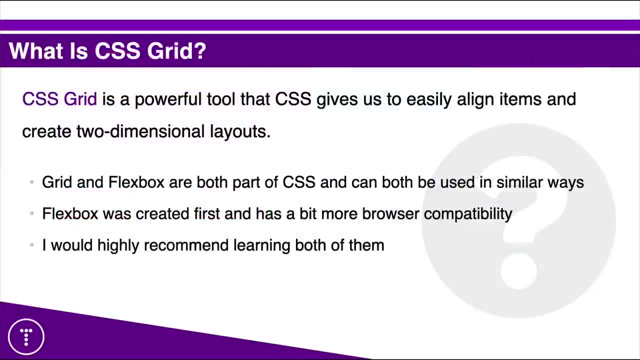 with the title of a blog post or a testimonial or something, And then maybe a picture of the person. the date- That's where I'll use Flexbox is to align those inner elements, All right. So that's just what I do, But again, it's going to be preference. I do know some developers that only use 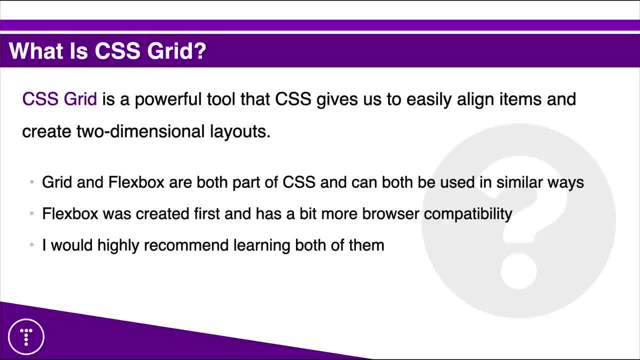 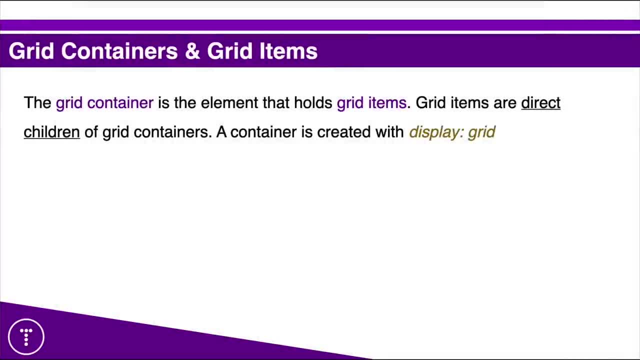 Flexbox. They don't even use CSS Grid, unless you know they have to for an existing project. But again, it's going to. it's going to come down to breakfast, It's going to come down to preference. So, with the grid we have, just like with Flex, we have containers and items. 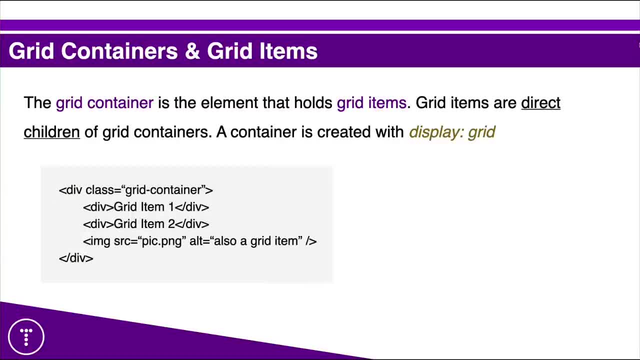 So we have, you know, an element that's going to be your container, And then any direct children of that element will be your items, And we create a grid, just like we create a Flexbox And that's using the display. So we have an element on the grid. 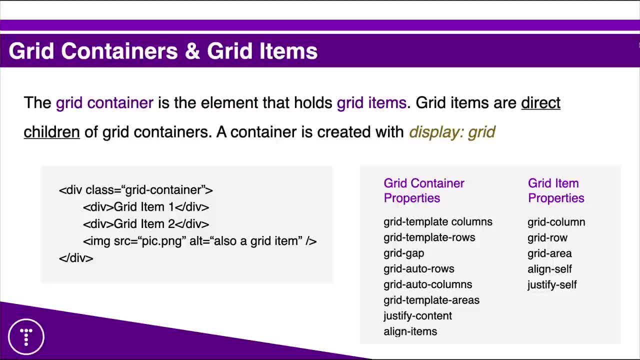 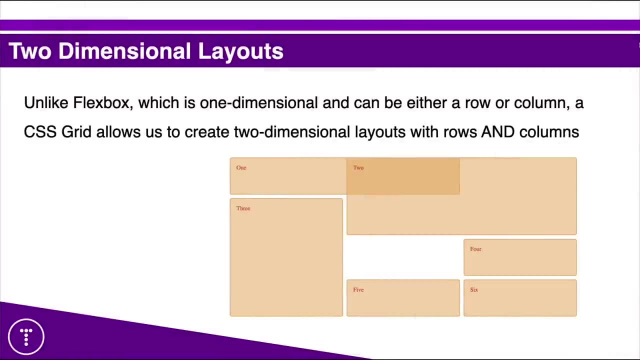 And then we have this specific property, And then we have specific properties that are available on the grid container, and then specific properties on the on the grid items, And we're going to get into all of these within our, in our sandbox, part of the of this crash course. 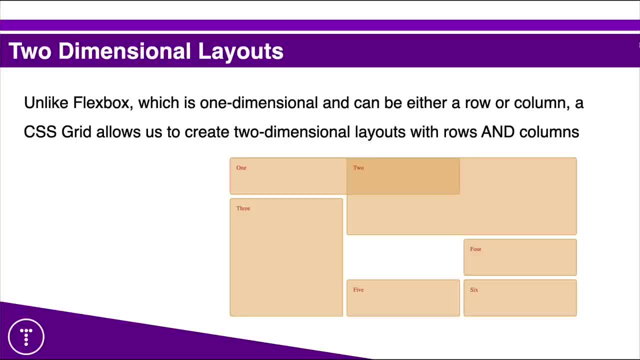 All right. So with Flexbox, you have the ability to create one dimensional layouts with either a row or a column. So you know, use flex direction, Set it to row or column. little more powerful where we can create two-dimensional layouts and we can use. 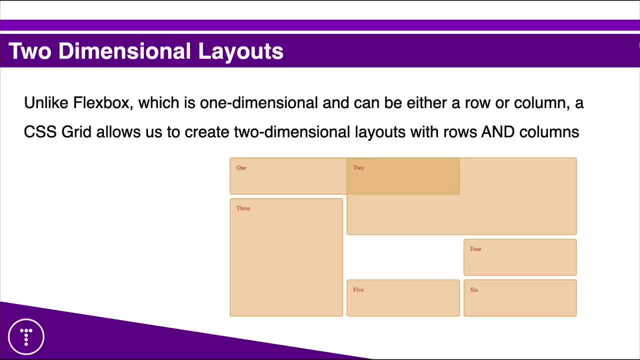 rows and columns in the same grid, and then we also have the ability to span certain rows or certain number of rows and columns, and it's just it. to me, it's a better option to, especially for more sophisticated website layouts and user interfaces, but we'll get into all that later on. alright, so enough with the. 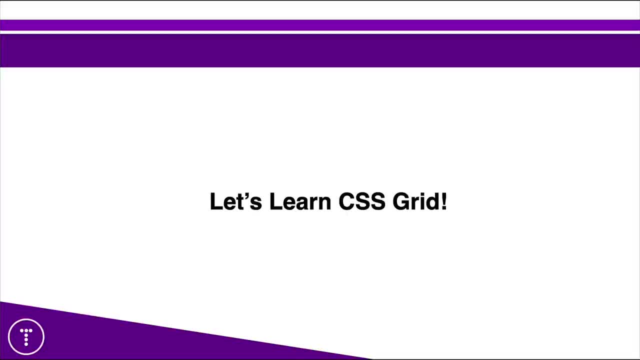 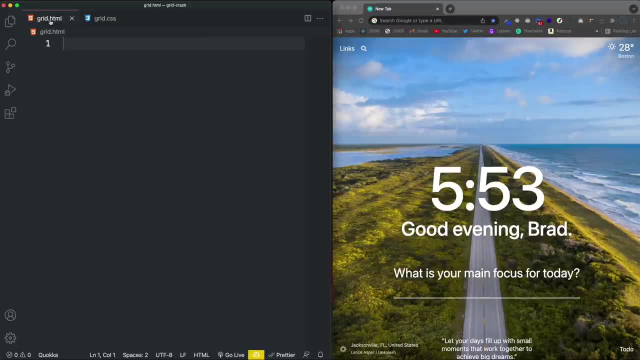 slides. let's go ahead and jump into vs code and let's start to learn CSS grid. okay, so I have vs code open. of course, you can use whatever text editor you want, and I have a grid dot HTML and a grid dot CSS file. that's it and they're. 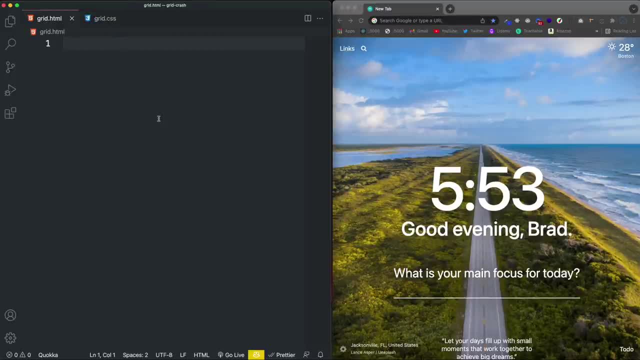 both completely blank. so we're gonna basically go through and learn all the different properties that the grid gives us and how to size things, how to create columns and rows and span items across multiple columns and rows and so on. so we'll start off with the HTML, which is gonna be really simple, so just. 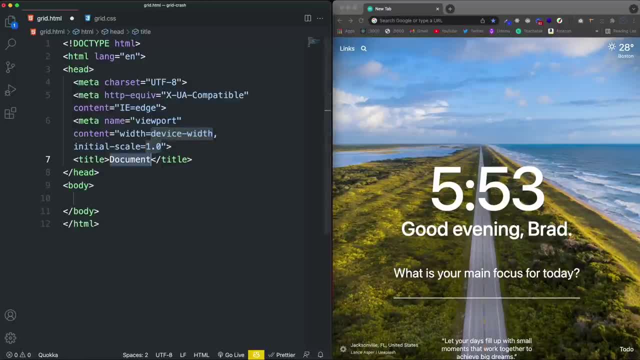 exclamation and there will give us a template in with using vs code and Emmet and title. I'll just say CSS grid, crash course, and then we want to bring in the CSS file, so that's called grid dot CSS and then the body is actually going to. 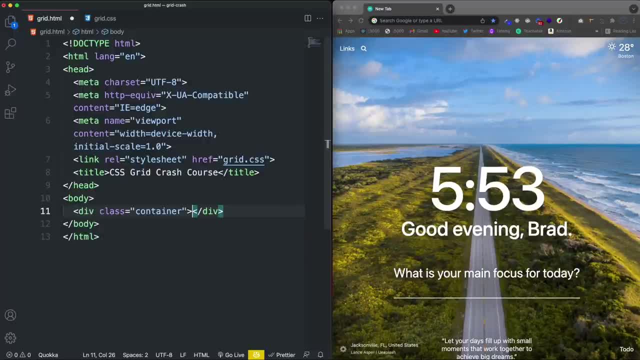 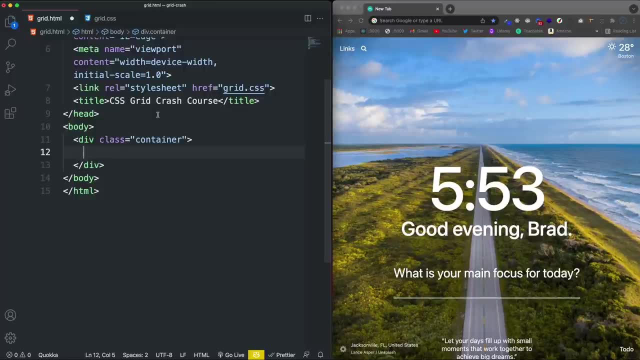 be really, really simple. so we're gonna have a container that's gonna be our grid container and if you're familiar with flexbox, it's kind of the same thing. you have your container that you have specific properties that you can use with the grid, and then you have your grid items inside and you have specific 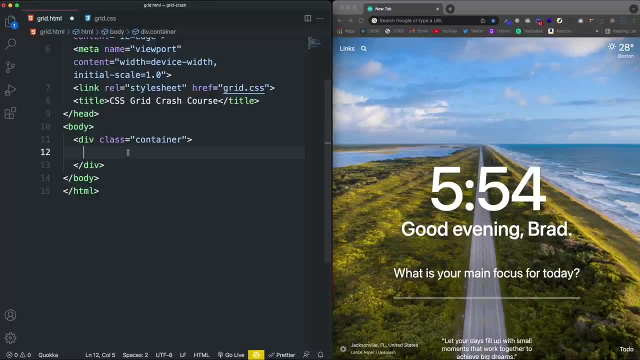 properties on those as well. alright, so in this container I want to have nine divs. they can be anything can be divs, images, headings, anything at all could be a grid item. but we're gonna do nine divs with the class of items. so I'm gonna say: 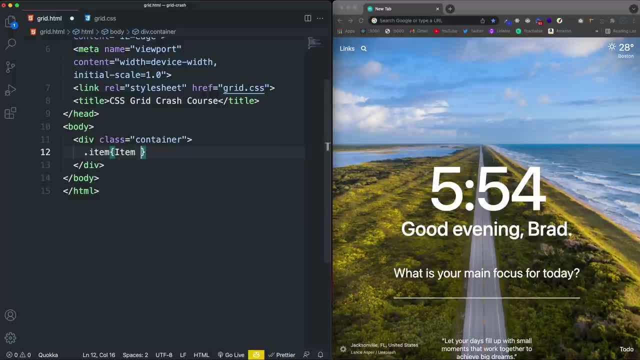 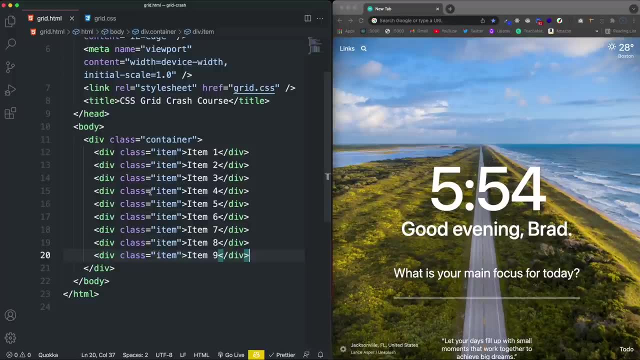 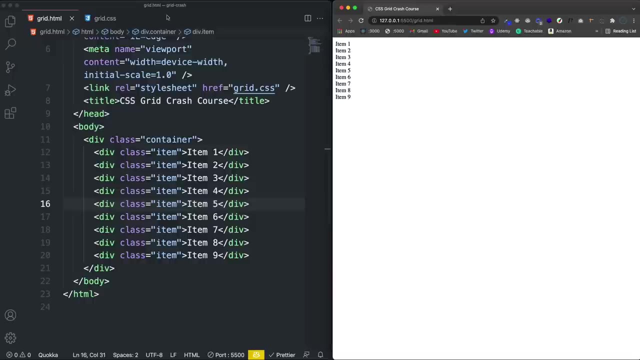 dot item and then I'll add some text, I'll say item and then whatever the current number is, and let's times that by nine and we get nine divs with the class of items. so i'm going to save that and then open that up with live server. of course you don't have to use live server, but i i am. 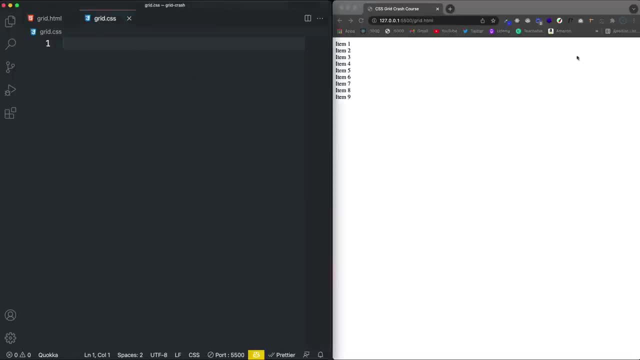 all right, so now we just see item one through nine so we can go over to our css, and i just have some some base css that i want to add. okay, so basically here we just have a reset. we have some body styling, font and so on. um the container. i put a max width of 960. of course you could make that. 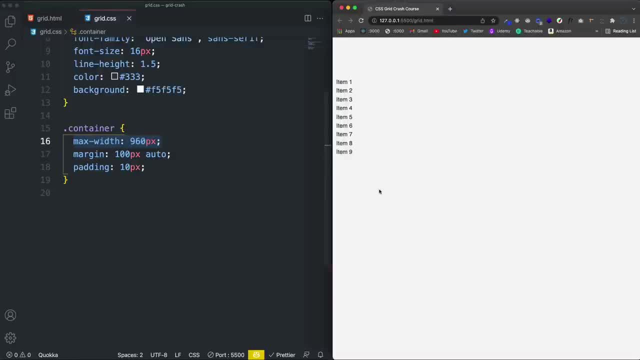 whatever you want. margin: 100 pixels on the top and bottom and auto on the left and right, so you can see there's a 960 pixel container here and that's going to be our grid container and then just some padding. so these items i don't want to just use text, so i'm going to basically 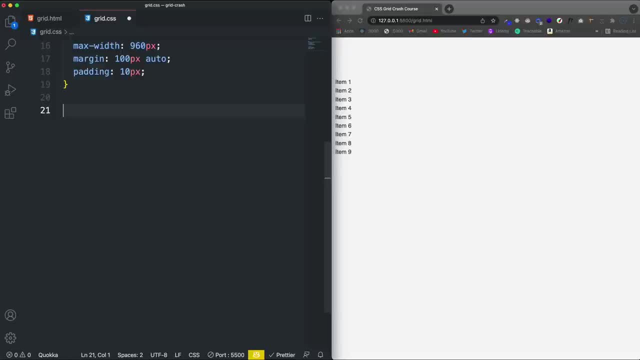 turn them into just blue boxes so we can clearly see our items. so let's say dot item and let's set the background. of course you can use whatever color you want. i'm going to use steel blue and then let's do color of white for the text and let's do a font size of 20 pixels and let's 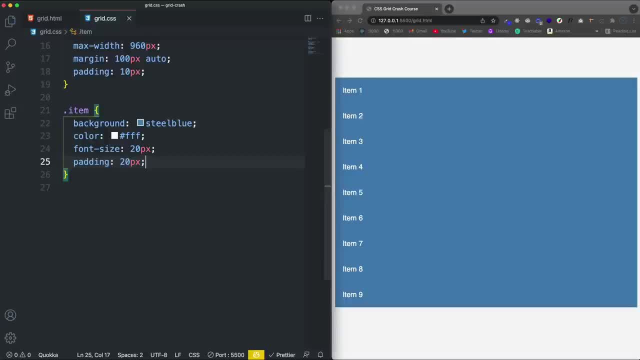 say padding, we'll do 20 pixels. okay, let's actually add a border as well. so we'll say border, let's do sky blue and one pixel solid, just so we can see where these end and begin. so we just have three, uh three, we have nine blocks or nine items now to make this container a. 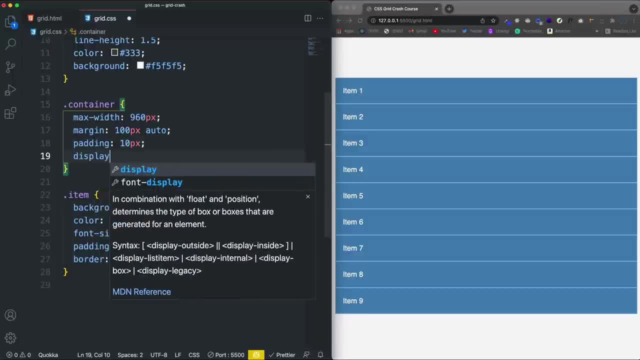 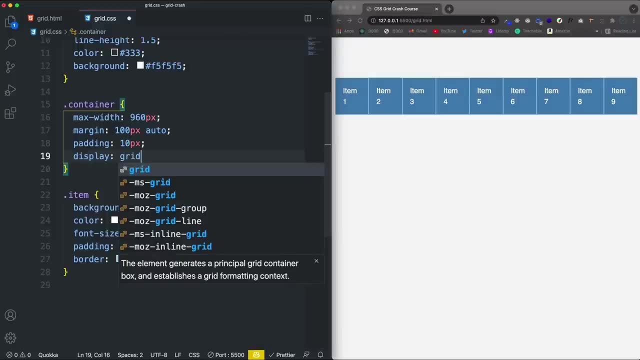 grid container. just like with flexbox, we use the display property right. so if we said display flex, it would put it into a flex row. we can see that immediately now. if we say display grid, it doesn't do anything. we can't see anything happen just yet because we need to specify. 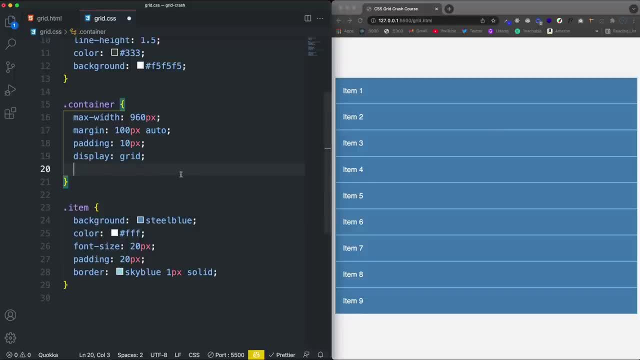 how many columns we want and how, how big we want those columns to be. property we're going to look at is grid template columns. so the way this works is we set some sizes so i can say, for instance, the first column 100 pixels, second 200 pixels. if i save that, i'm going. 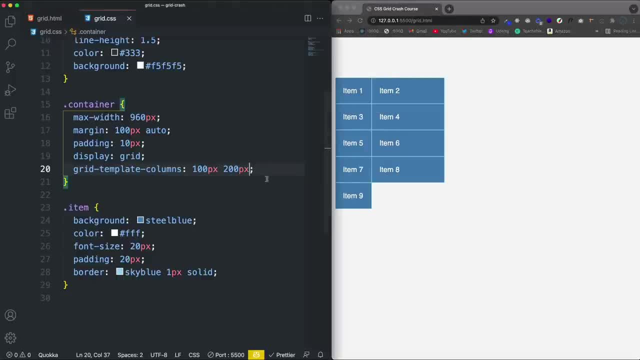 to get two columns, first 100, second 200. if i wanted a third column of 300 pixels, i could go ahead and do that as well now, and it doesn't have to be just pixels, i could use percentages. so if i do 30, 40, 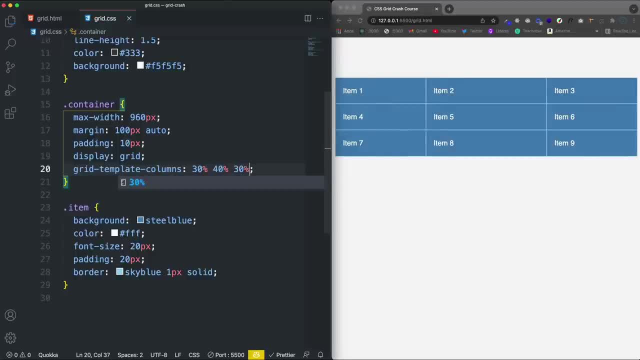 30 and save that. you can see. now we have percentages, but most commonly you're going to be using fractions. so if i do one fr and one fr, these are fractional units and this is just going to give me two columns that are the exact same width, if i make this browser. 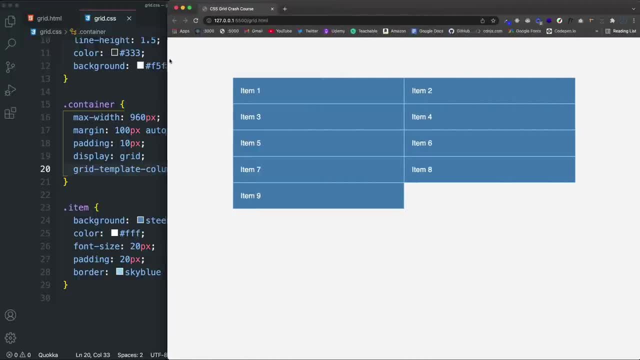 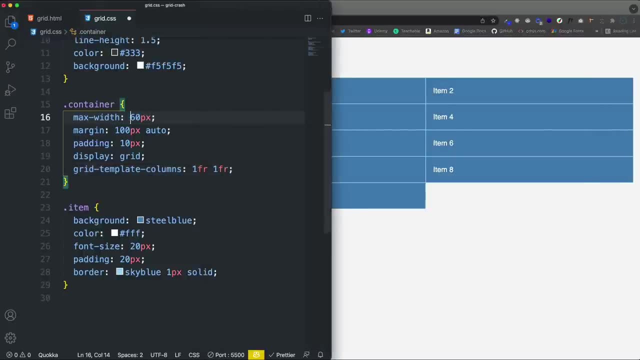 wider. you'll see, it's going to. it's just going to take up the entire width of whatever the container is, which in this case is 960, but of course i could change that to 1160 and make it bigger. i could change it to 660 and make it smaller. so, whatever the, whatever the width of. 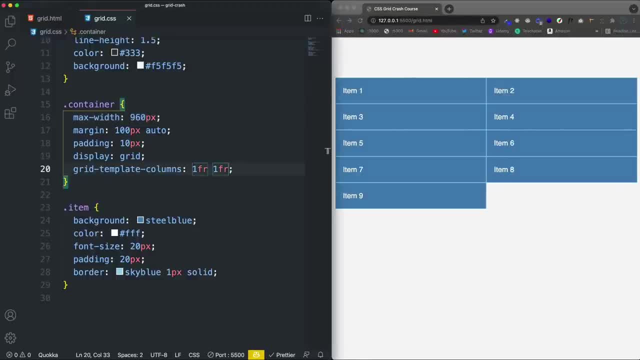 that container is all right now. i could of course add more here and i can make. i can make certain columns bigger. so if i want to do 2fr here now, you'll see that the third column is bigger than the first two. if i want to make the middle one three fr, then that one's going to be bigger all. 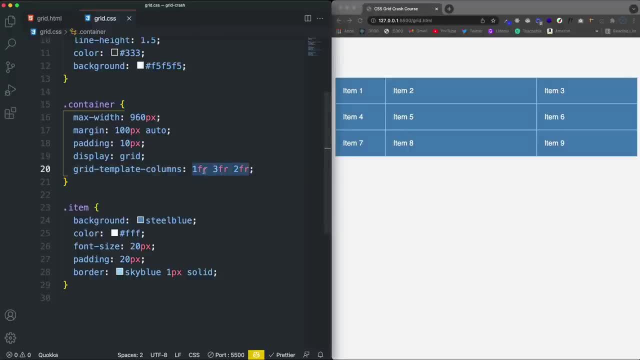 right now i actually want to have three of the same, so i could do one fr three times, or i could use the repeat function and just say repeat three times one fr, and if i save that, you'll see it'll give me the same result as if i did one fr three times. now, when it comes to spacing, 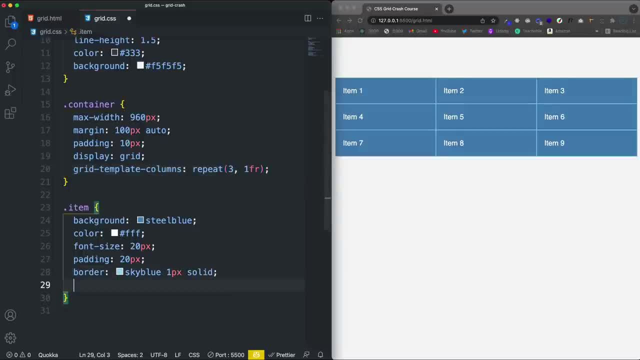 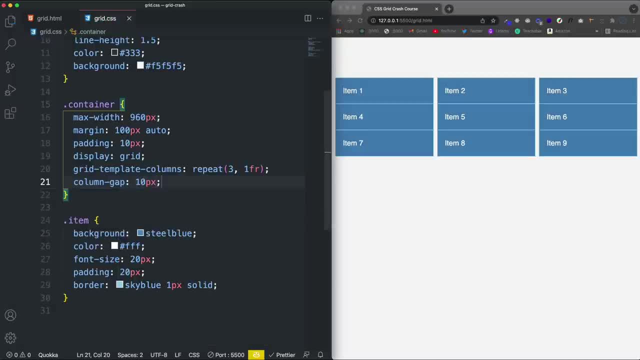 so i'll say column gap 10 pixels, and you'll see that will add space going vertically between the columns. and then we also have row gap, which you can probably guess what that does: it adds a space between rows. now if you want to use both of these instead of using two properties, we could just go. 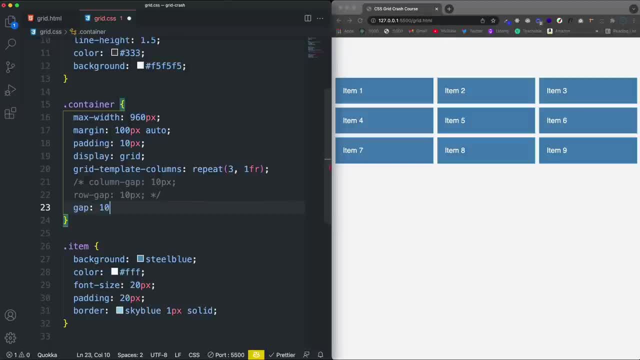 ahead and do gap and we'll set that. we'll do 10 pixels and you'll see that it gives us the- the same exact result, all right. so we know how to divide the- the same exact result, all right. so we know how to divide the items up into columns and we know how to make columns certain widths. 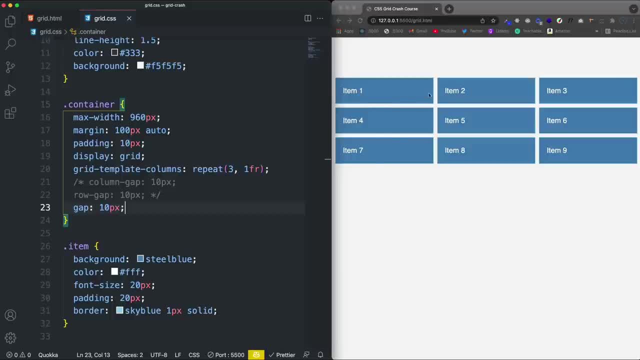 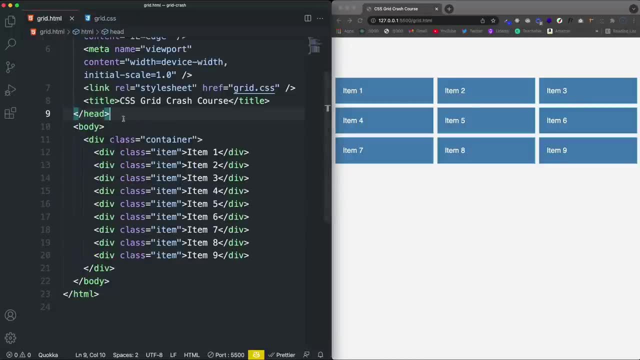 so now let's talk about height. so the height right now is going by the content that's in each, each grid item, and it's all basically the same content. so they're all the same size. so i'm just going to go ahead and replace this with, let's say, larm 30. 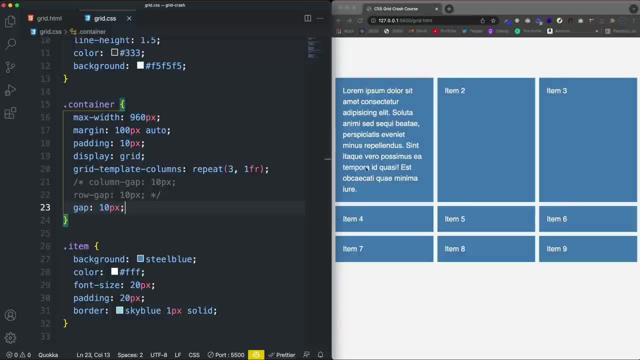 and save that, and now notice that the height expands to fit the content by default, and then all of the columns that are in that grid are all the same size. so i'm just going to go ahead and and save that, and then we can also look at this, and then i'll show you the options we can use. 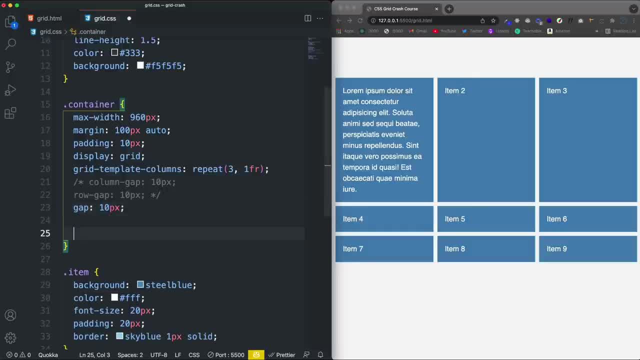 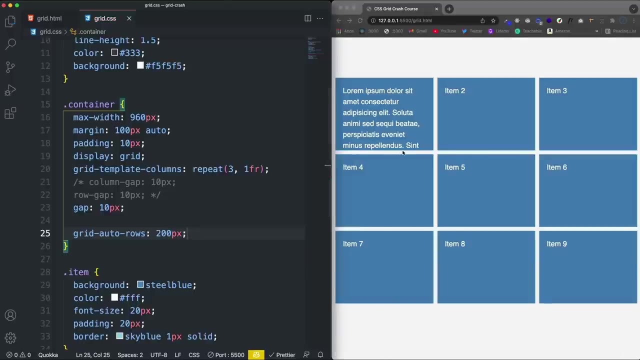 on this tab here in the首 up here, so that when i'm doing that row also expand on height by default. so there's a couple properties that i want to show you that have to do with with rows and height. so the first one is grid dash, auto dash rows. so with this we could set 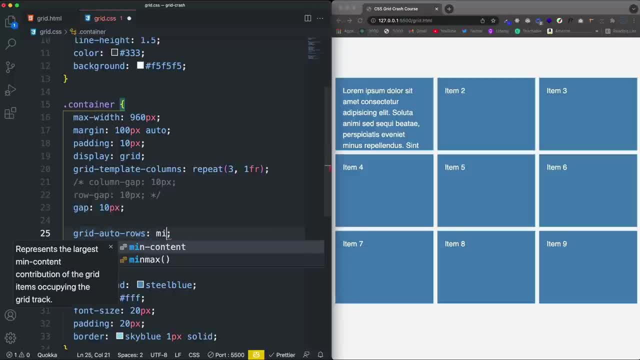 all of them to 200 pixels, regardless of the content. you can see it actually gets cut off here. as you can see, it defines a size range greater than or equal to min and less than or equal to max. so basically it takes in a minimum- we'll do 100 pixels- and then max- we'll just do auto. 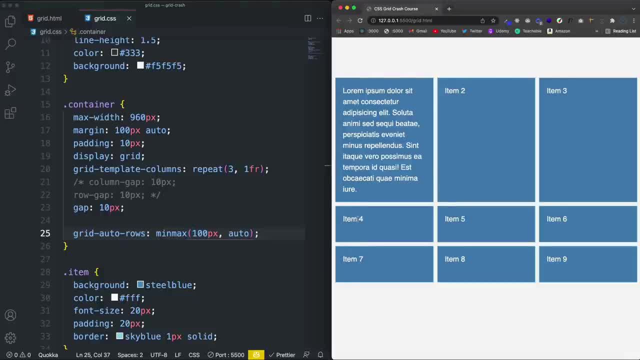 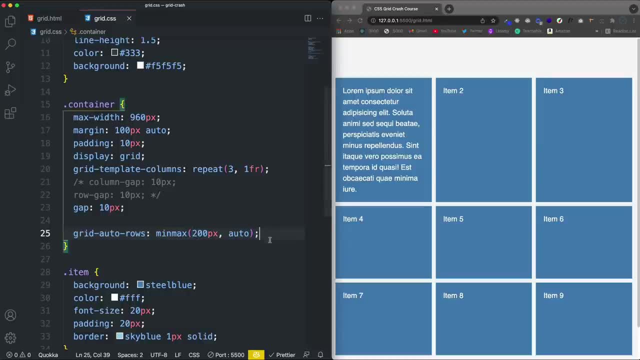 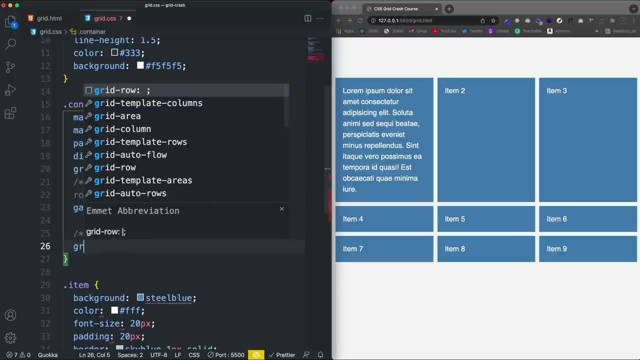 so now we can see all of the content that's set to auto, and then these other ones are going to be set to 100.. if we want those set to 200, then we could do that all right now. just like we have this grid template columns, we also have grid template rows, so that's what i want to look at next. so 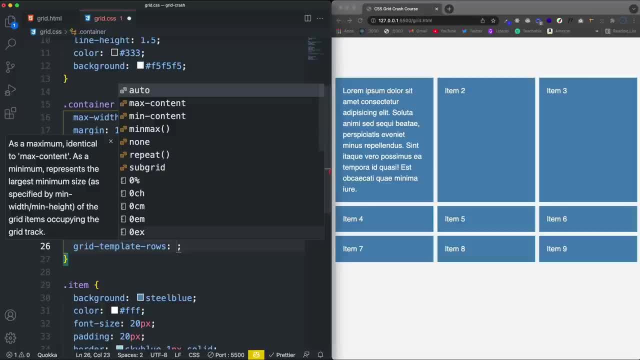 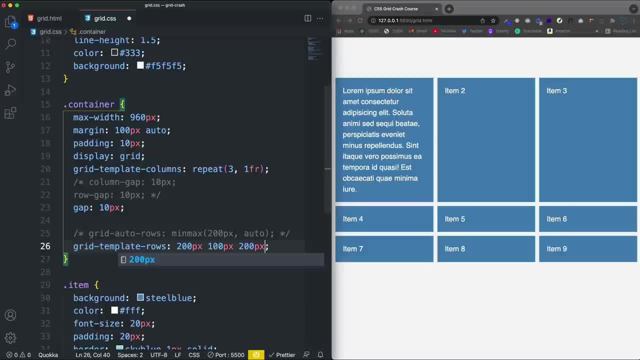 let's say grid template rows, and we could use pixels or percentages or fractions. for now let's just say like 200 pixels, 100 pixel, 200 pixels, and it's just like grid template columns, except instead of going this way, it goes this way. so we have 200 pixels, 100 and 200, all right, and you can. 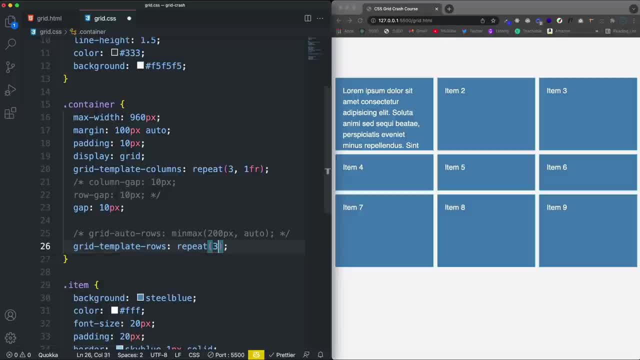 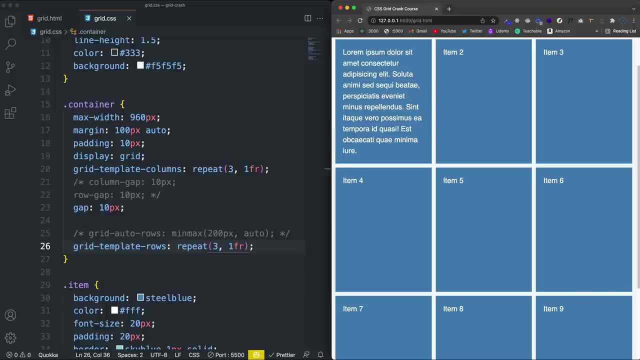 also use, like we could say repeat. we could say repeat three times: one fr, save. and now by default, the height is going to be of whichever the the most content. so if i were to come over here and slash this in half and save, then that's going to. 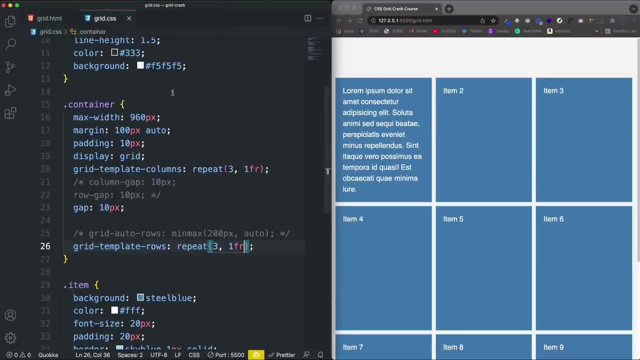 resize the height of all of these. so i i don't find myself using grid template rows that much, because most of the layouts that i build just the the content determines the height, and then i'll align things with the alignment properties that i'll show you in a minute. but it's good to know how these work, so i'm just going. 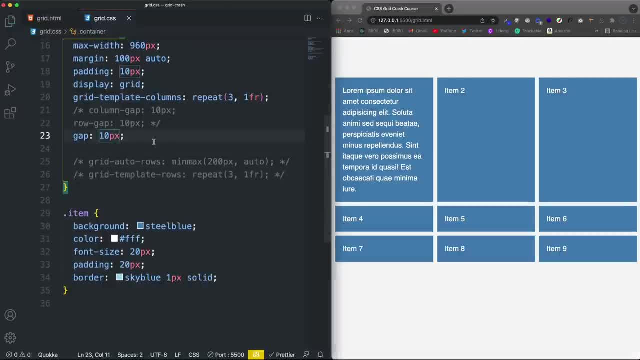 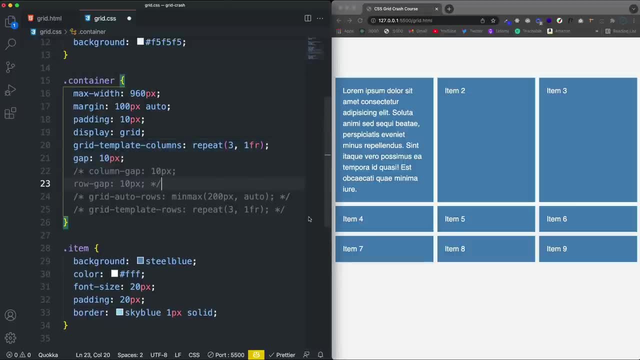 to comment all that out and let's- uh, let's move this up here. i just, i just want to have this. i'll probably create a repository so you guys can have this as kind of a reference. so let's see, what do we want to look at next? let's look at, let's look at, some of the alignment properties which, if you 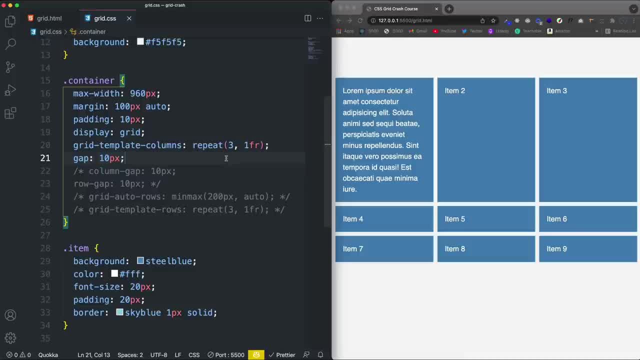 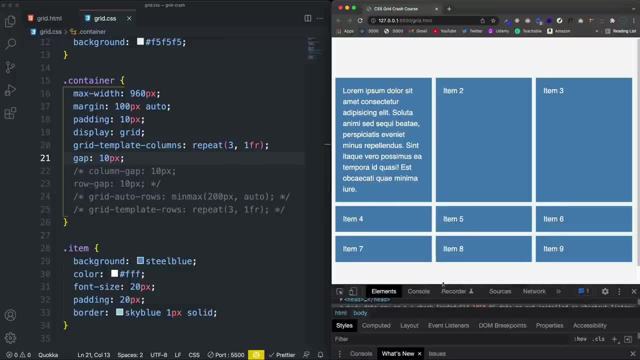 know flexbox, you probably already know, so align items, justify content and so on. now, before we do that, i do want to show you that in the google chrome dev tools and firefox dev tools- i'm not sure about the other browsers- i don't use anything else. if you have a, 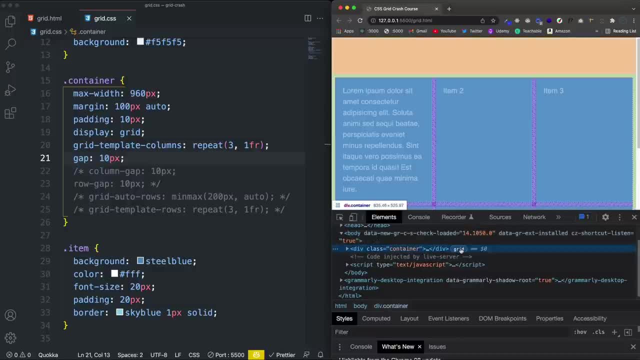 grid container, as we have here. you have this little grid button and if i click that, you'll see we get this highlighting and you can also get these numbers. now, if you don't see the numbers, you can just go down to layout and under grid just choose show line numbers. you can also show the 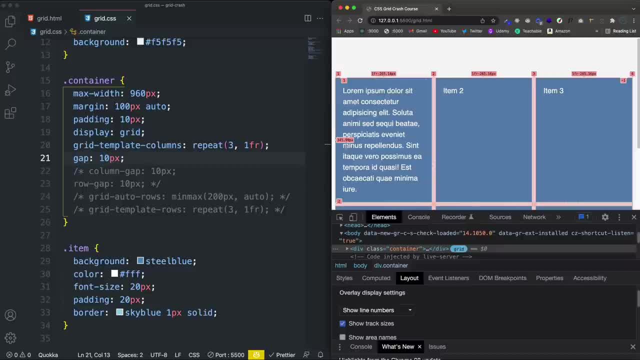 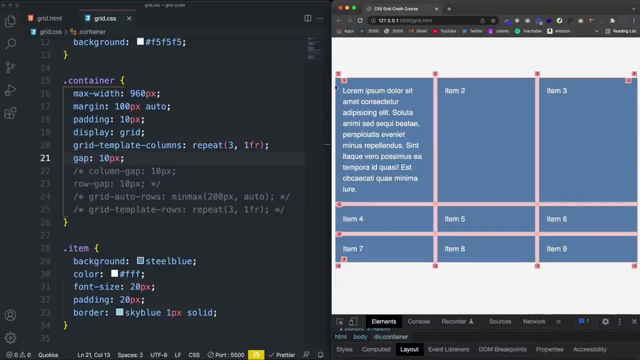 here you'll see like one fr and the number of pixels, and here as well, but i don't want to keep those displayed. so i'm going to uncheck that. but i do want to keep the numbers because when i show you how to span across rows and columns, these numbers really come in handy. so let's see, i want. 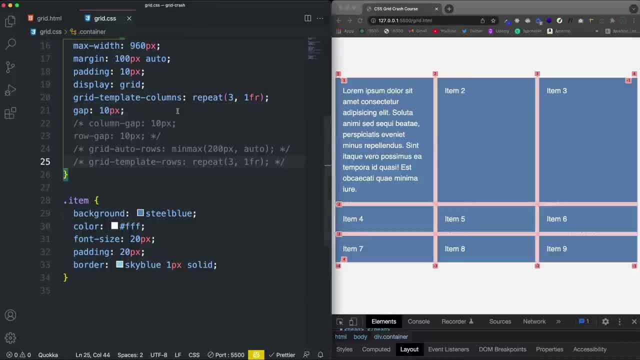 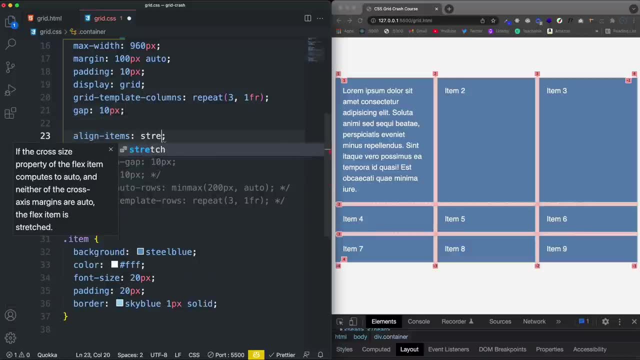 to start off with align items. so let's go. we'll just go here and let's say: align items. now the default for this is stretch. okay, if i save that, i'm just going to go ahead and go ahead and go. we're not going to see any difference. and what that does is: is this right? here it stretches. 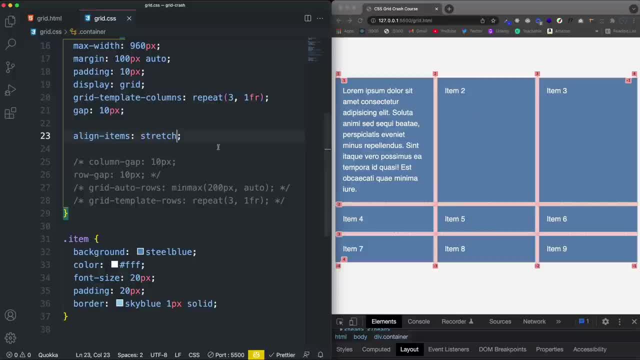 uh, go according to whichever one has the most content. now, you might not want that, so we could set this to, let's say, start. all right, so what that's going to do is align it to the top here. okay, if i want to align it to the center, i could do that. if i want to align it to the end, 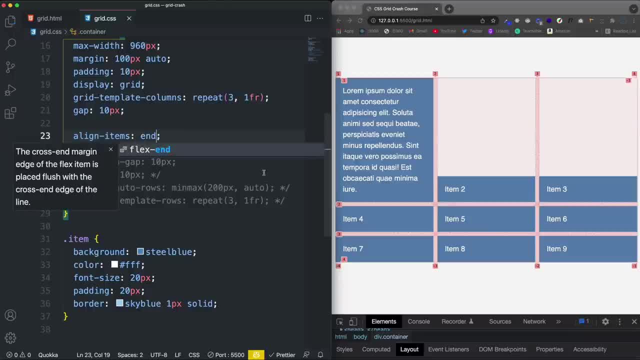 i could do that as well. all right, and- and this will take effect if any of these are have have height to them, like if i. if i go ahead and uncomment this grid, auto rows, you'll see. now they're all aligned to the bottom, but i'm going to just make sure i comment that back. so as far as justify content, in order for 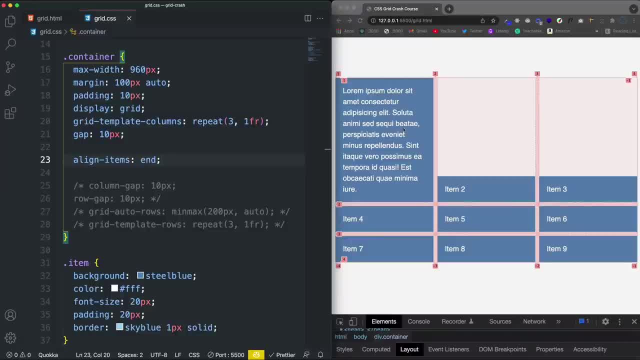 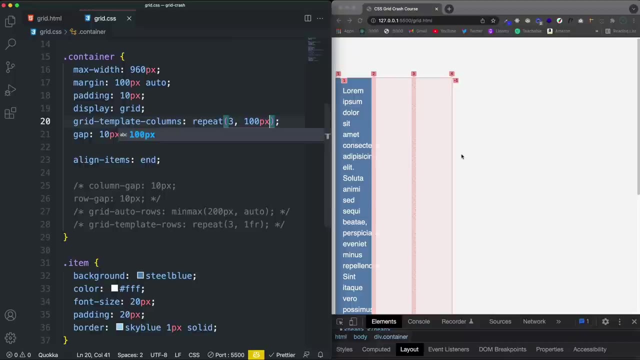 us to really see how that works. we can't have the, the content, taking up this whole space. so just temporarily, i'm going to set, let's say, repeat, 3 100 pixels. all right, so now we have three 100 pixel rows, or sorry, columns, and if i wanted to align all of these, let's say, to the end, i could use justify content and set that. 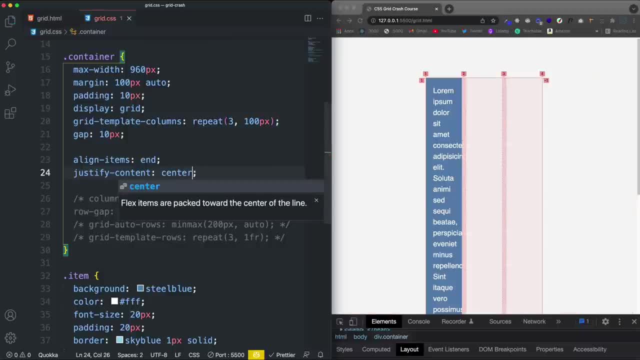 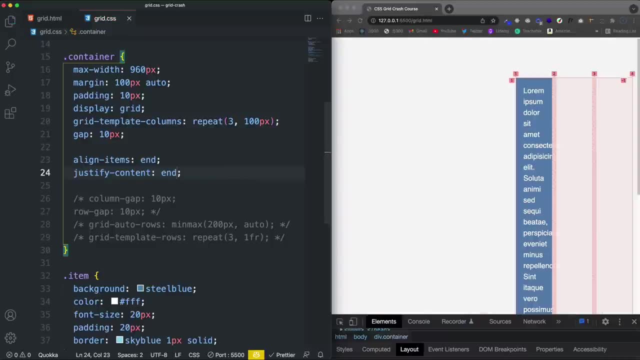 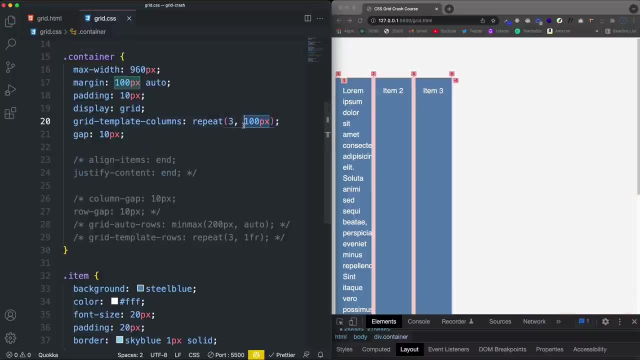 to end and it would move them over to the end. i could do center, move them to the center, and so on. we could do also like space around. you know so all those different values, and if you're familiar with flexbox, then you already know those. so let's set this back to one fr, and now you can also align. 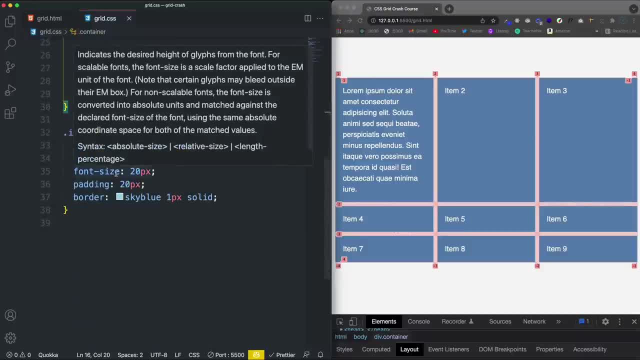 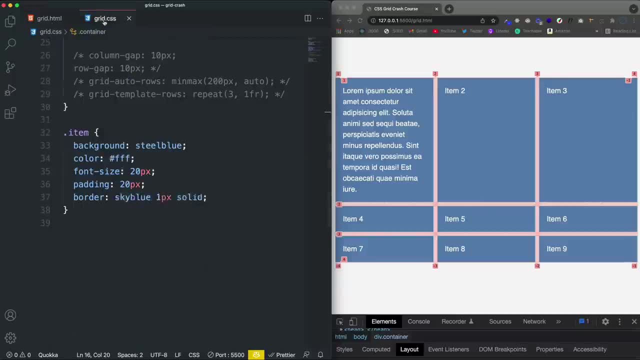 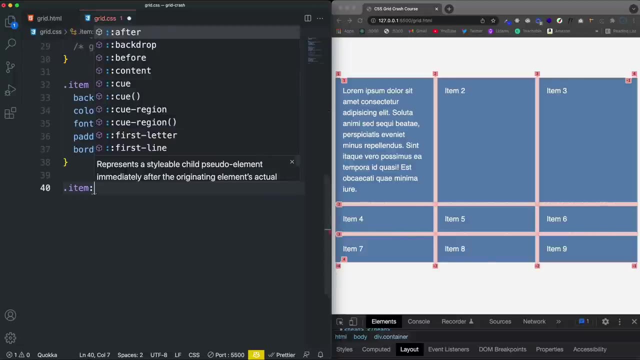 self meaning on the item itself. so i don't have specific classes like item one, item two, item three, to to grab these. but of course we could use pseudo selectors. so i want to grab the second item. so what i would do is item colon and then we could use nth of type and then i'm gonna pass in two. so 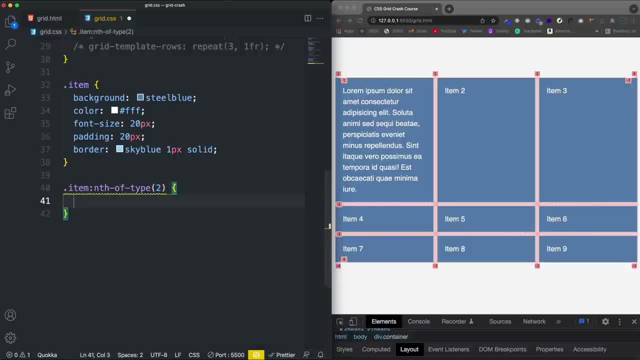 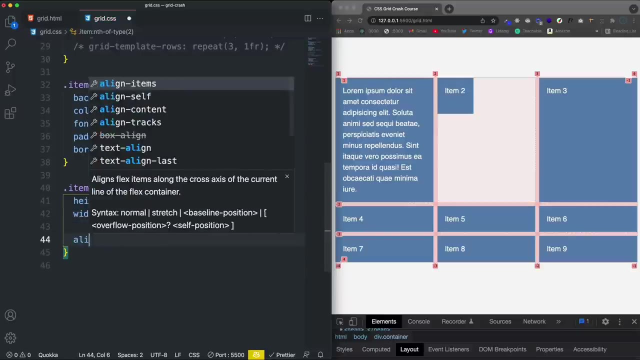 that will select the second one, and i'm just going to change the height just temporarily, just to show you how this works- the height and weight, the height and width to 100 pixels. okay, and now if i want to align this, let's say a line item, i'm sorry, not align items. align items is for the container. 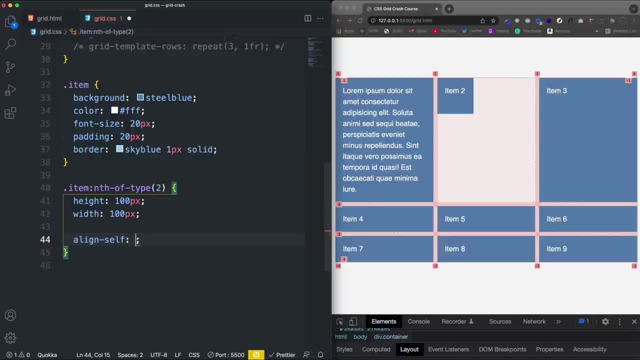 align self is for the actual item. So I want to align that to, let's say, end, And you'll see that it gets moved to the bottom. So I want to move it to center. I could do that And then, if I want to, 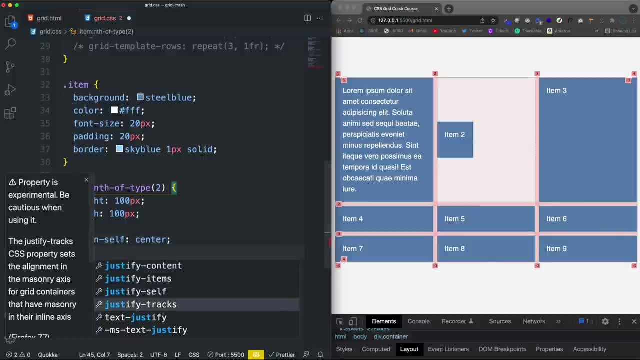 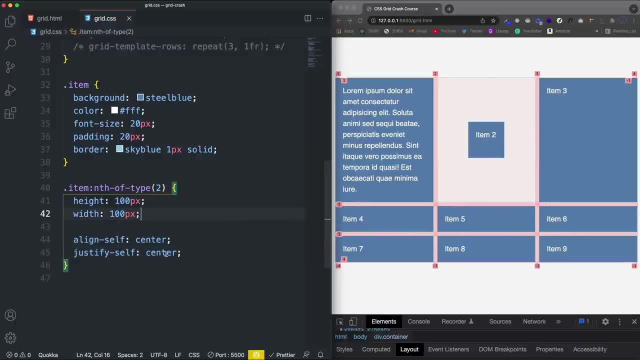 move it along the x-axis, I could do justify self, And let's say we want that to be center, All right, So I'm not going to keep this. I just wanted to show you that those properties are available. So the next thing I want to move to is spanning items across a number of rows, or 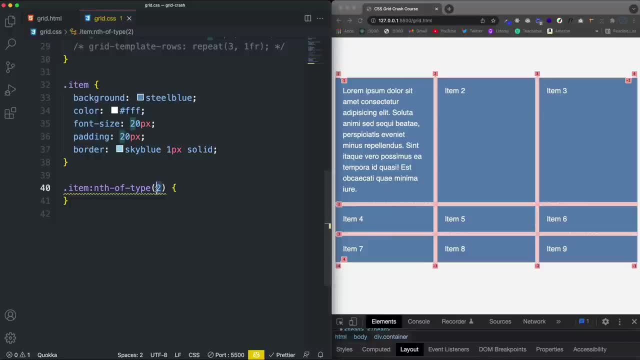 columns. So I'm going to start with the first one here. So I'm going to change this 2 to a 1.. That's going to select this first one And we'll just go ahead and change the color. I'll change. 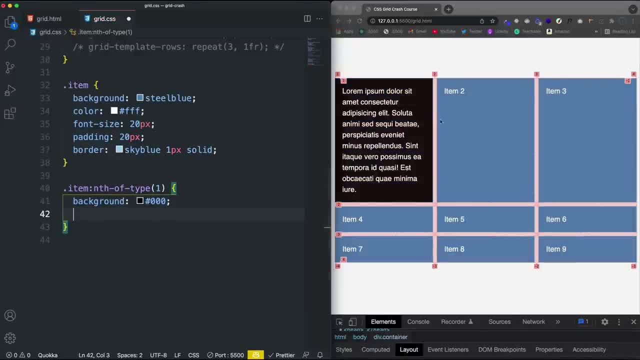 it to black, And let's say that I want this to span from line 1.. So these are grid line numbers from 1 to 3 instead of just 1 to 2, which is the default. So I could do grid-column-start and set that to 1,, which is where it is currently, But then I want. 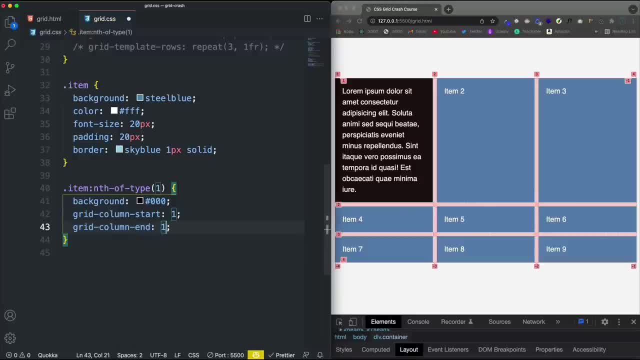 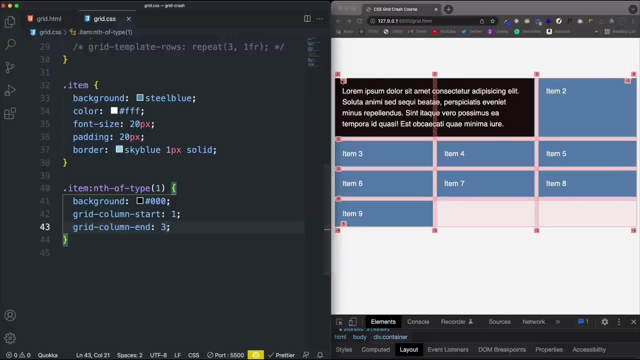 grid-column-end. I want that to be 3 instead of 2.. If I put it to 2 and save, it's the same thing, But if I put it to 3, it's now going to stretch over to column 3.. All right, So I should say: 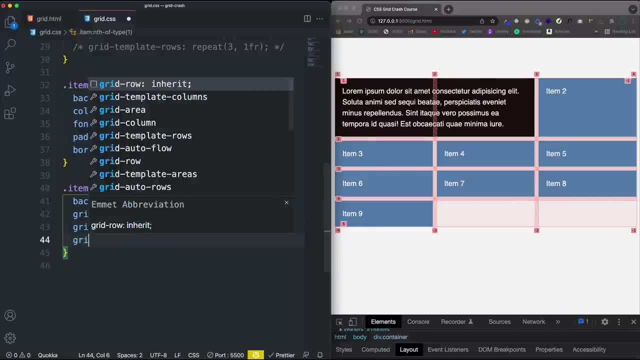 line 3.. Now there's a quicker way to do this. Instead of doing start and end, you can simply say grid-column, And then we can just do 1 and then slash 3 like that, And then we can actually get rid of this, And that will do the same thing. Another way we could do it is we could 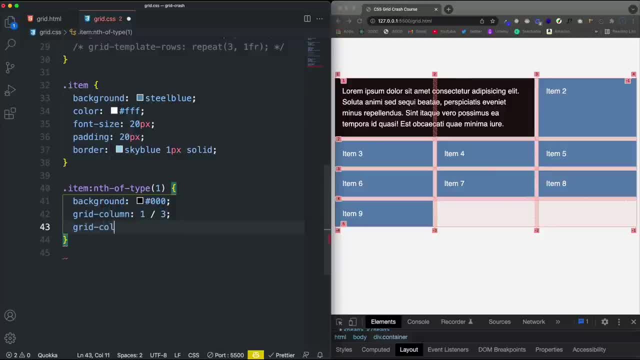 say grid-column, And we could say 1 and then do slash, span 2.. So instead of just specifically saying we want it to go from 1 to 3, we could say start at 1 and then span 2.. If I comment that out and save, we should see the same result, But I prefer to do it this way. 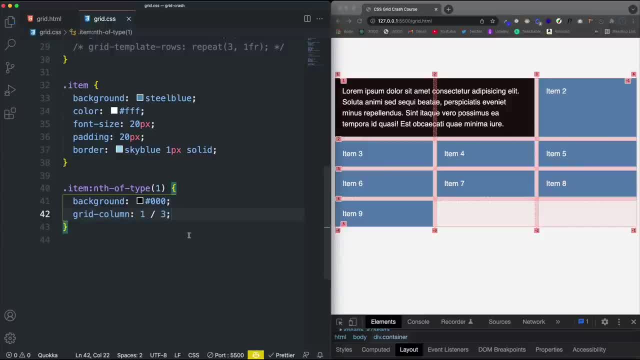 and explicitly say where it starts and ends. Now we can also span rows or span down. So let's say item 3 here, which right now goes from 2 to 3. Let's say we want it to go from 2 to 4.. So I'll just go ahead and grab this And let's select item 3. And we'll change the color. 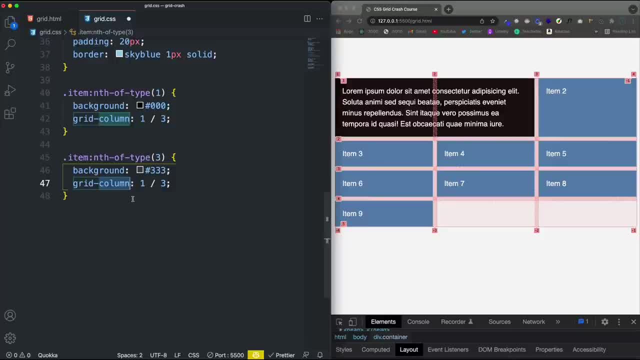 Lighten it up a little bit. And then instead of grid-column we're going to do grid-row, And it starts at 2.. So we're going to say 2. And we want that to go now to 4.. So it's going to go from here. 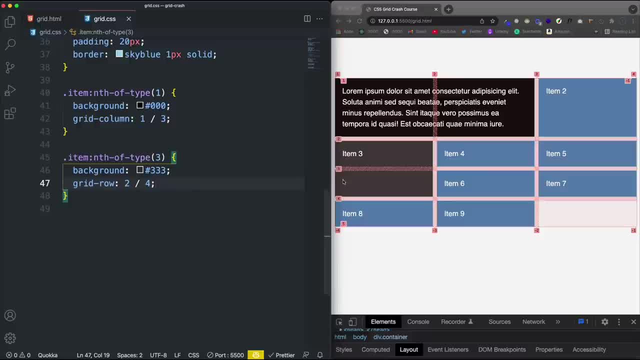 2 to 4.. All right, So we'll save that, And now you can see that that spans from 2 to 4.. Now let's do the same thing with item 4.. So I'm just going to grab that And then we'll say: this is: 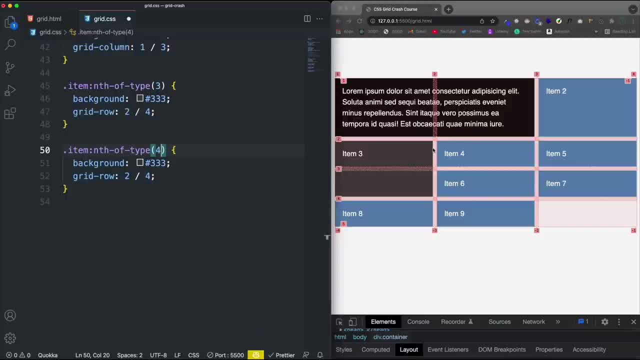 grid-column And we'll just keep the same color And then grid-row is going to do the same thing. We want it to go from 2 to 4.. So we'll save that. So you can see that CSS grid. it is more powerful. 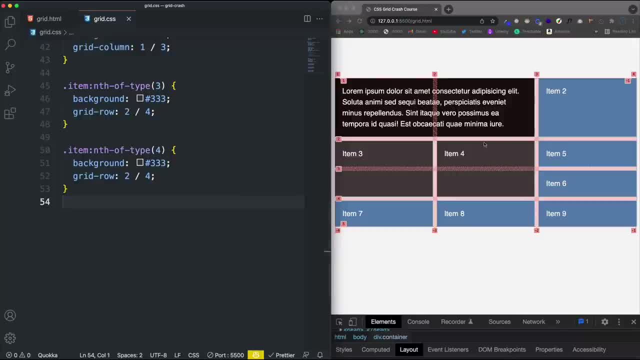 than Flexbox. It's two-dimensional. There's no way to do something like this in Flexbox, have these two here and this, unless you use multiple Flexboxes. This is all one grid. So now what I'm going to do is turn off the grid lines here. 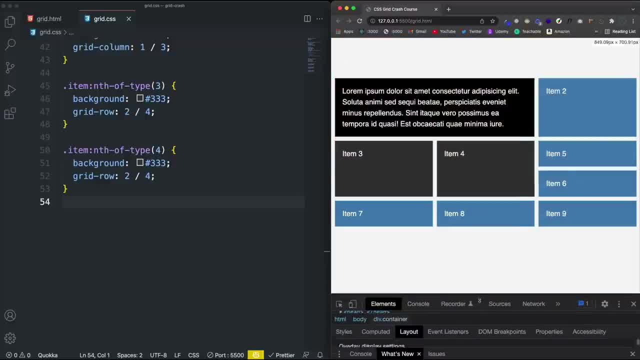 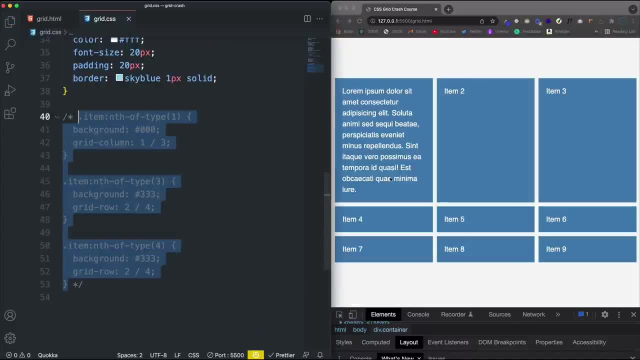 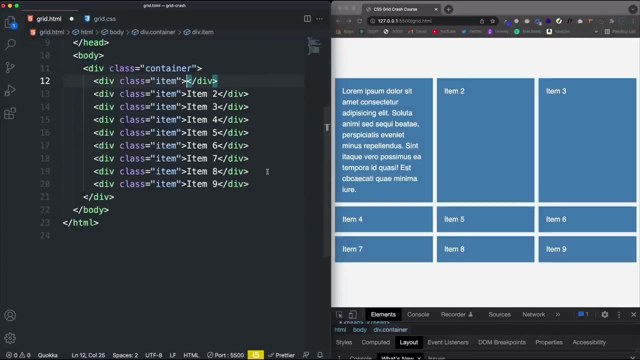 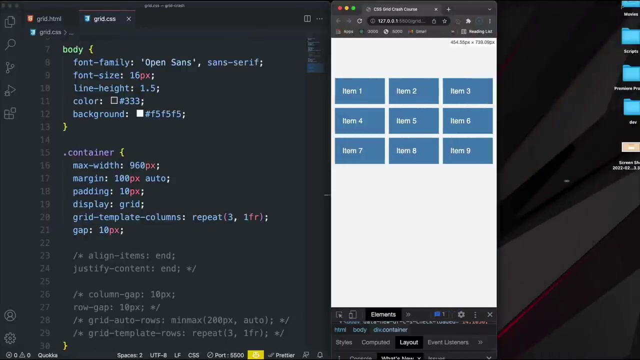 Let's shut those off And then let's comment out this stuff here where we did all the spans. So we just have three columns across And I'm actually going to just change this back to item 1.. All right, Because now I want to talk about responsiveness. So right now, no matter how, 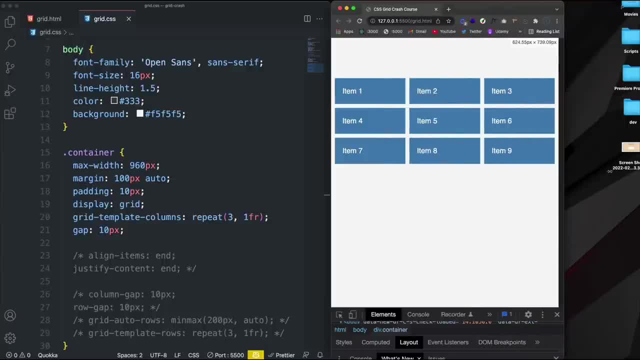 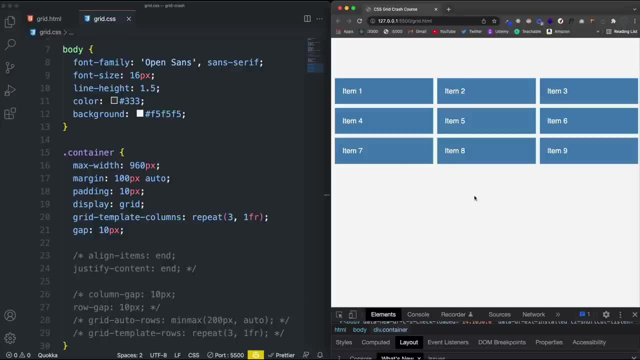 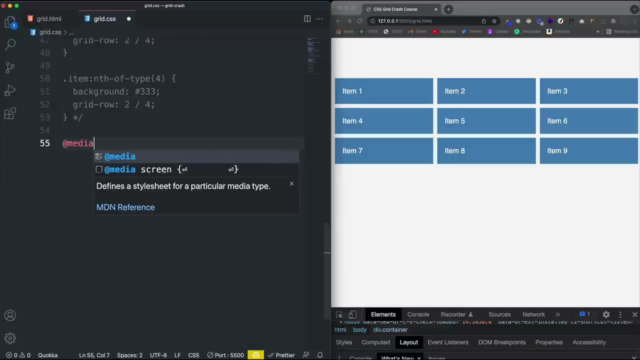 the browser is sized. we have three columns right And that's probably not what you want. So what I usually do is just create media queries and just have them stack on smaller screens. So, for example, I'd come down here and say: at media, And we can do max, We'll say max. 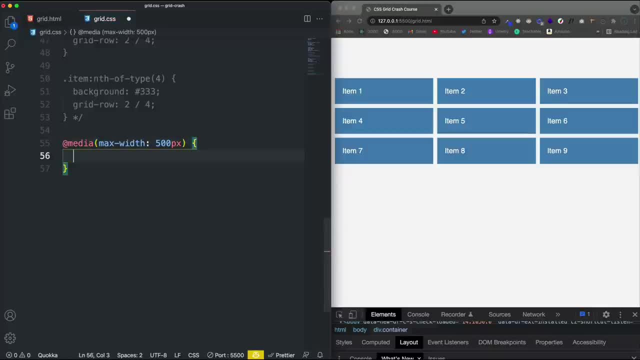 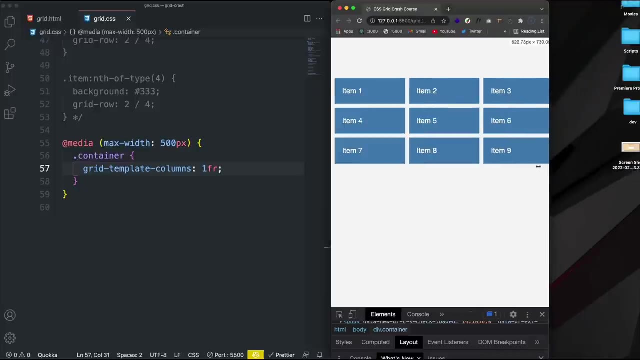 with 500 pixels And then we can set the. let's take the container And let's set the grid template columns to just simply 1fr. So now, if we take the browser and we resize it down to 500 pixels, then you can see they all. 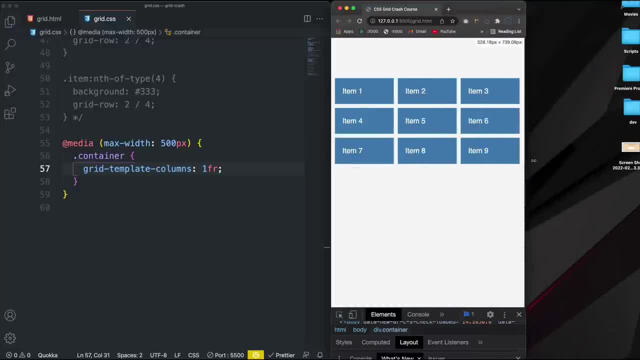 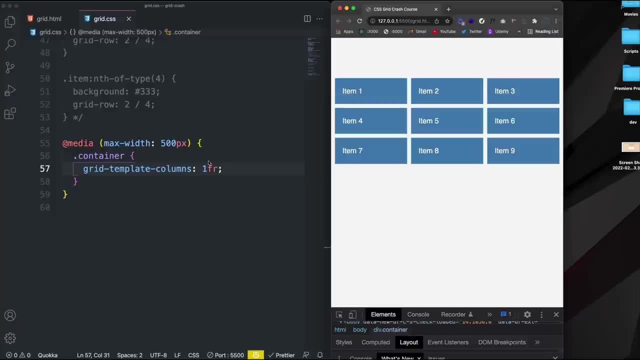 stack All right, So we can do that Now if you want these two. and of course, you can set other media queries and you might set it to 1fr, 1fr, or use repeat to 1fr for maybe 768 or something. 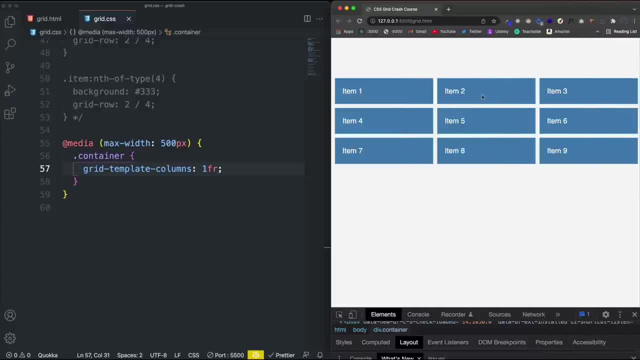 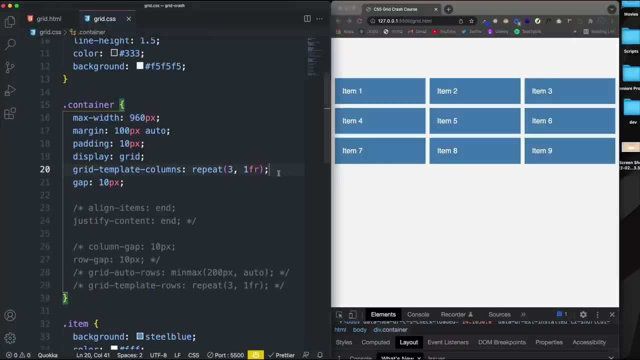 like that, But you can also make these, make these wrap, like with Flexbox. you have flex wrap. So to give you an example of that, we'll go up here and let's copy this grid template columns down and then comment it out. 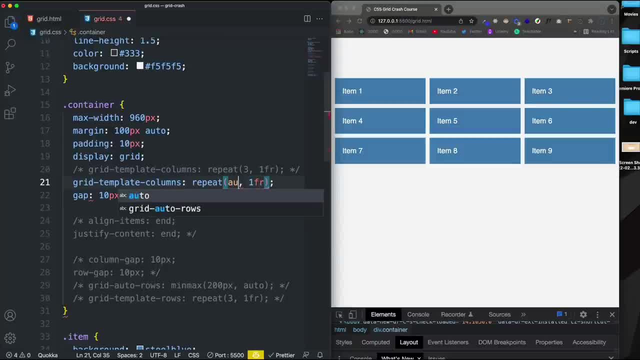 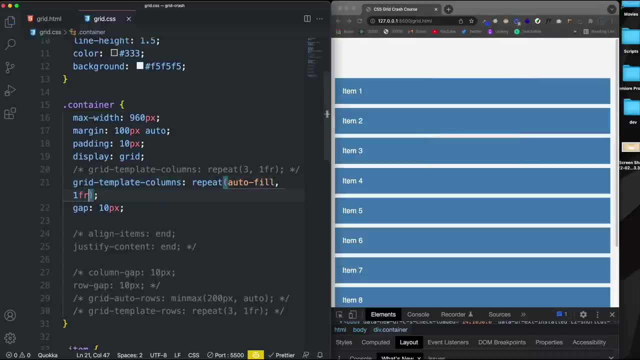 So what we could do is pass in here, let's say, auto-fill, And then instead of just 1fr, because if we do it like that we're just going to get that result. So instead of that we can do: we can use min-max here And we want to pass in here whatever the minimum. 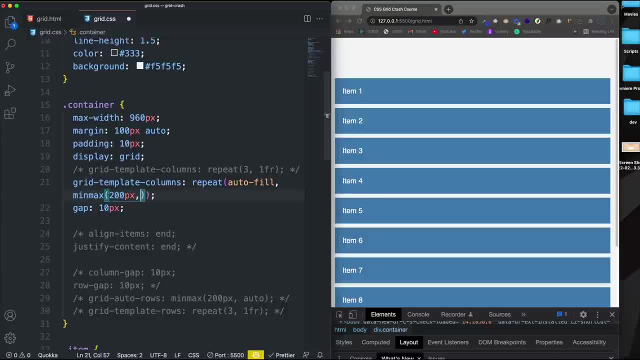 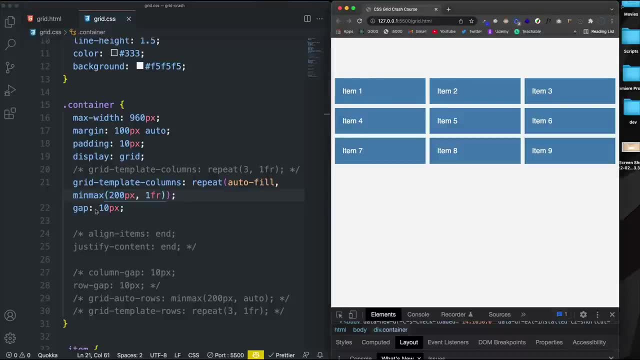 width you want. So let's say 200 pixels, for example, and then we could do 1fr here. So now what happens is we get three across, because we're saying if it's 200 pixels, then put it in, But if 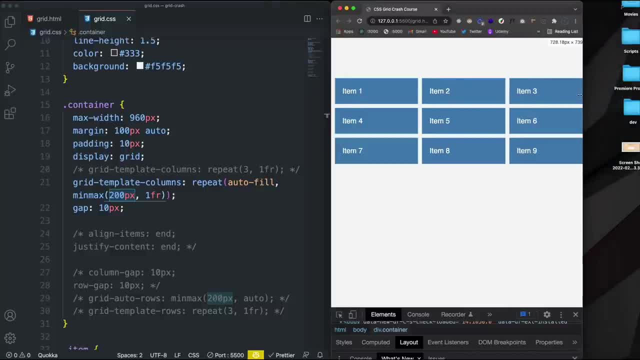 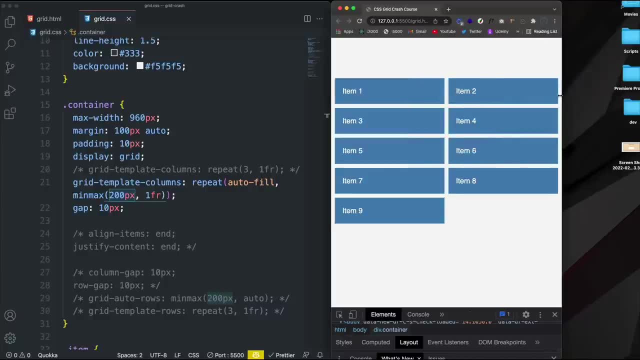 we go below that. so let's see, we're going to go, keep going, And as soon as one of these goes below 200 pixels, then it wraps, And now we have two columns, Okay, And then we still have our media query. 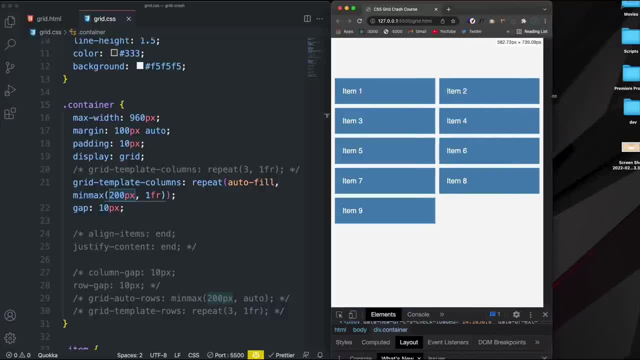 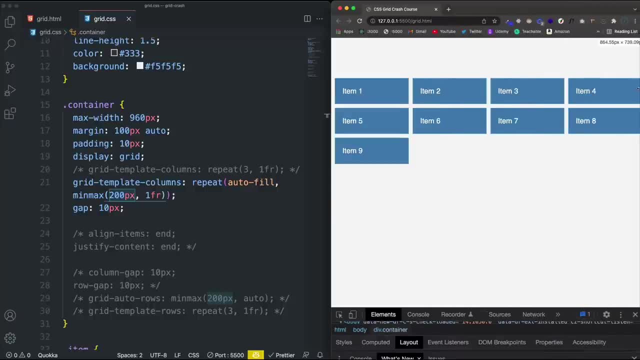 So if I keep going and I hit 500,, then they're going to stack. If I stretch it out long enough, we should see four columns as well. All right, So that's how you can make your grids responsive. Now, obviously, if you're. 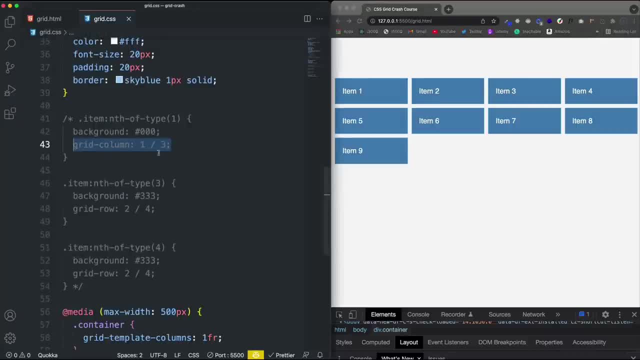 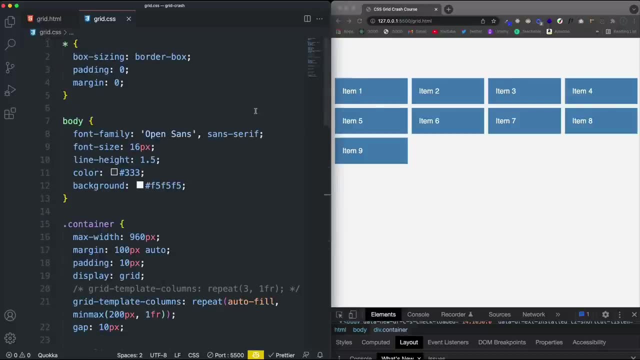 going to keep like the grid, the spans, like this, then you have to account for those in your, in your media queries as well. All right, So that's pretty much it for for the basics and how to use the grid. Now there's one more thing I want to show you before we move. 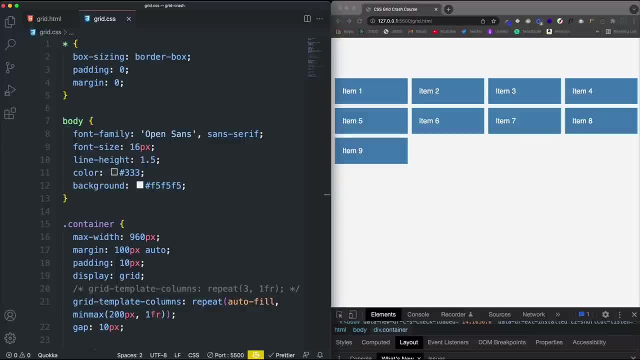 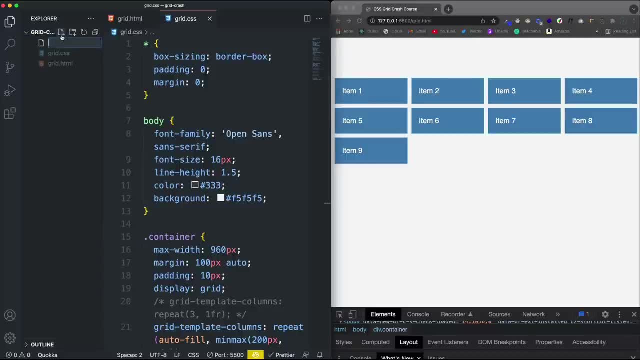 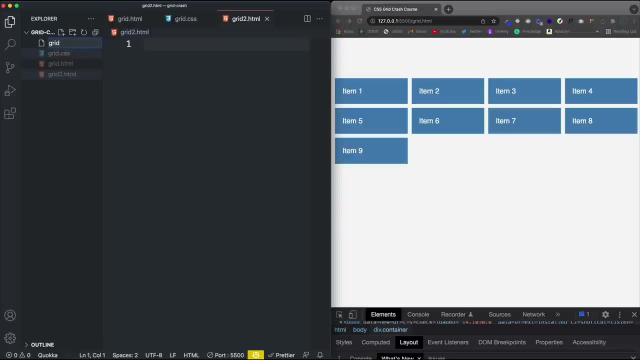 on to the little project they have and that is a grid template areas, which is kind of a different way of of doing things. So I think what I'll do is just create two more files, say grid, two dot. HTML. Uh, and then we'll say: we'll do grid. say grid, two dot. 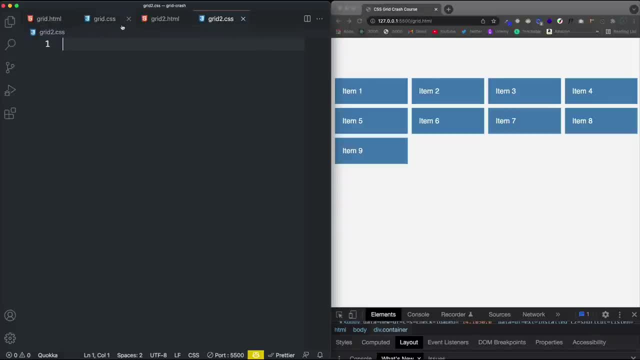 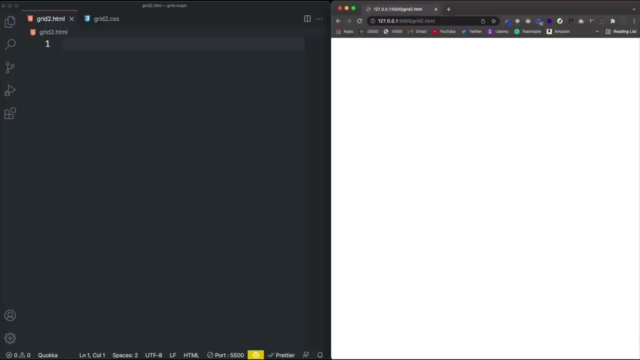 CSS. All right, And I'm going to just close up grid HTML and grid CSS. So we have the two new files And then let's go to grid two, dot HTML, which is completely blank right now. So I just want to show you a picture of what I'm. whoops. I don't want to open it in Photoshop. Let's. 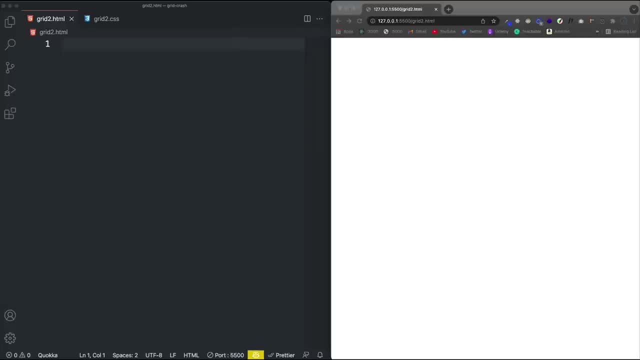 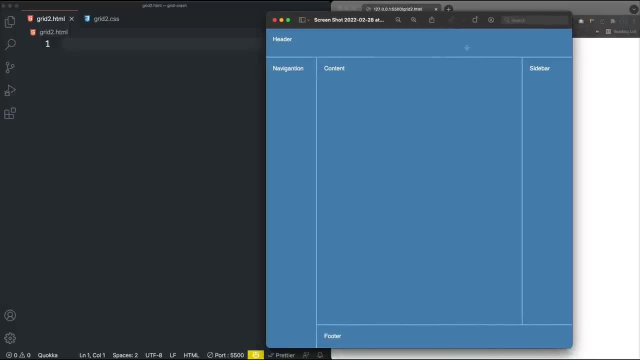 open it with preview. So this is the layout that I want to create, which is a pretty common type of layout. So we have a header at the top that goes all the way across, have some navigation on the side that goes all the way down under the header. 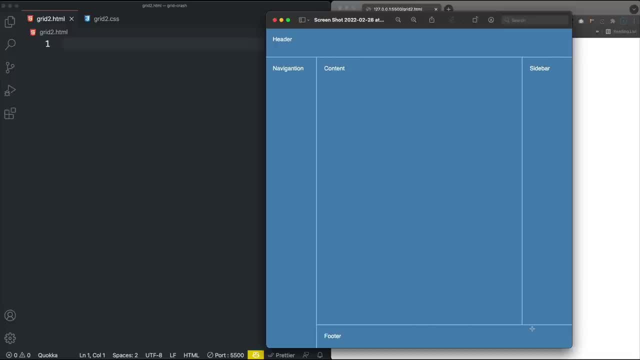 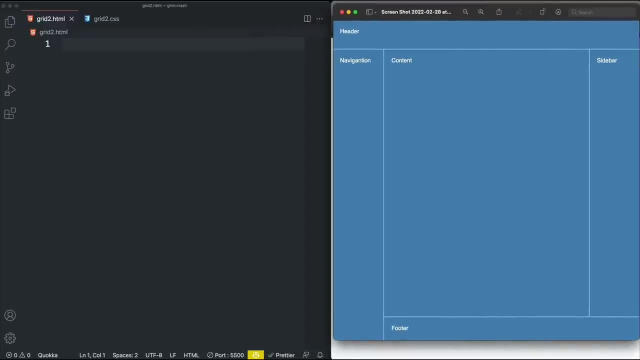 chau: The content, and then the sidebar, and then the footer. that goes under the sidebar and the content. So I'm going to show you how to do this with grid templates or grid template areas. So, first thing, let's add our HTML, which is going to be really simple. We'll just throw. 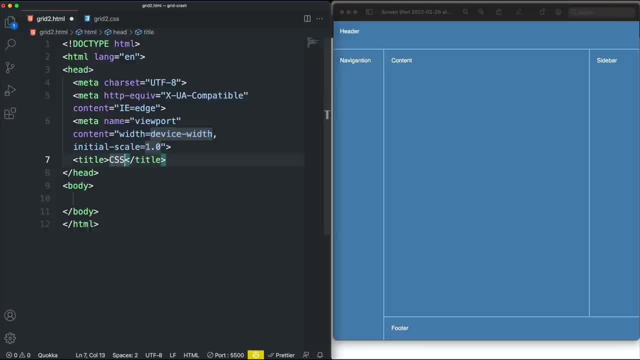 in a template here and let's say CSS, CSS, grid template areas, and let's add in a link here And this is going to go: Uh uh, olhaор Th stata are gonna��고 họperem. 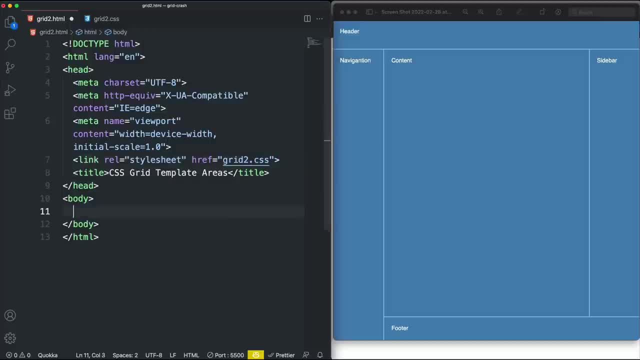 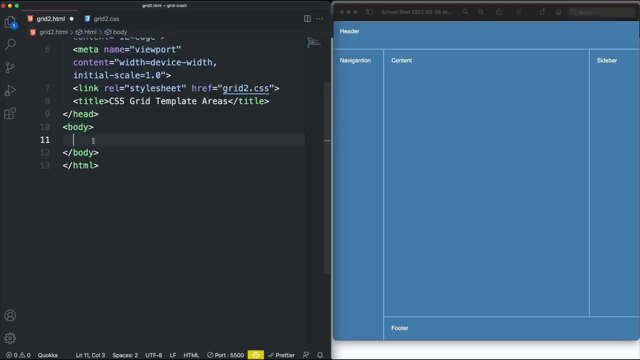 go to grid2.css now. in this case i'm going to use the body as our, as our grid, as our grid container, and then any direct elements are going to be grid items. so first we'll have a header and i'm just going to put some text in here. so you have header, we'll have a main tag and here we'll say content. 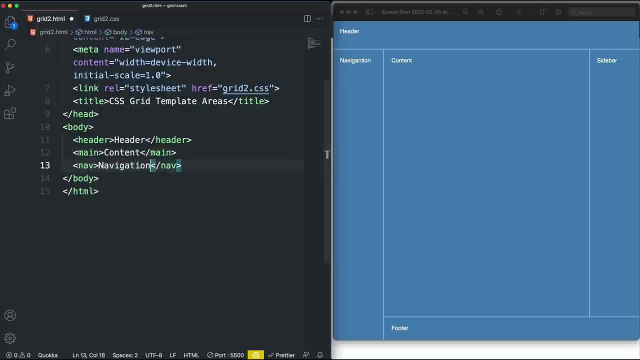 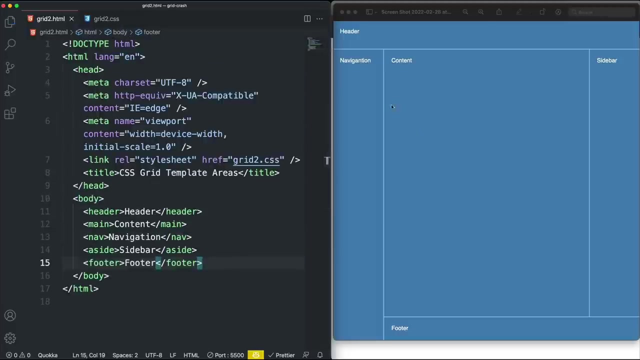 then we'll have our nav, say navigation, and oops, let's do an aside, so that'll be our sidebar. and then what else? our footer, which will be footer. all right, so that's all i want to have, and i want to turn this into this using grid template areas. so let's go into our. i'll get this out of. 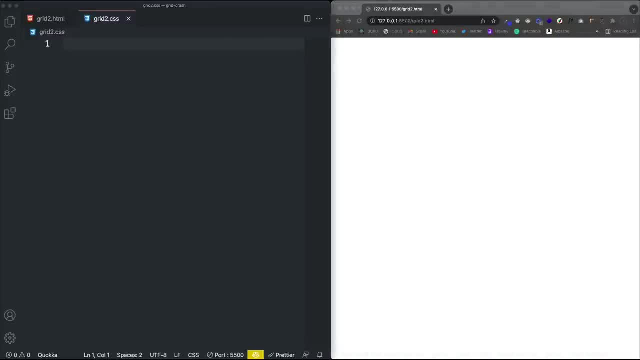 the way. now let's go into our css- and there's some just basic css i'm going to pass in here. so just a reset, some body sizing, and then let's make the wait a minute. there we go. so let's make the body, the grid. actually, before we do that, let's take all the elements and let's make, turn them into. 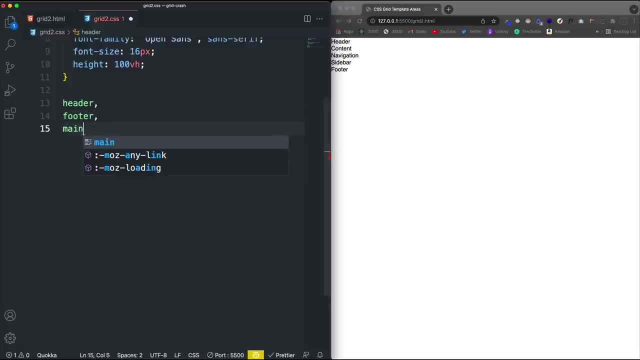 blue boxes. so we'll say header, footer, main side and nav, and let's do background color and we'll do steel blue, let's do color, we'll set that to white, and then padding 20 pixels and let's do border. we'll do sky blue, one pixel solid. all right. 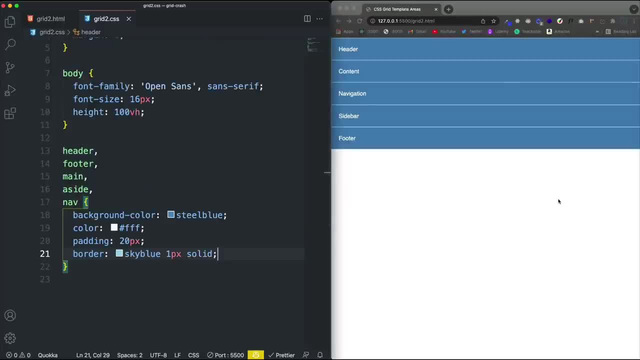 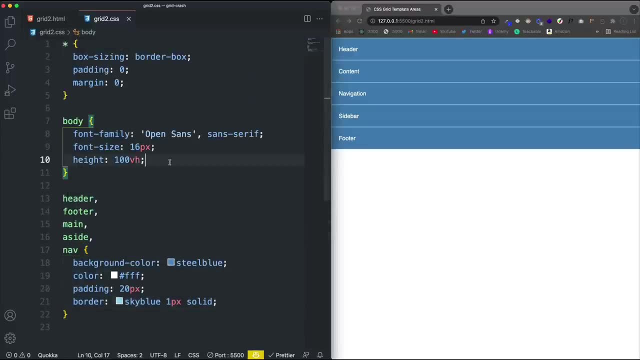 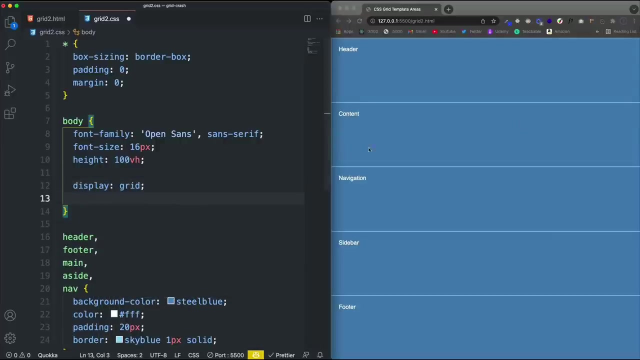 so we have no positioning or anything like that, we just have a bunch of blue blocks, just like we did, uh, in the last, you know, in the last file. so, like i said, the body is going to be the grid, so we'll say display grid, which does right now. it the reason that it. 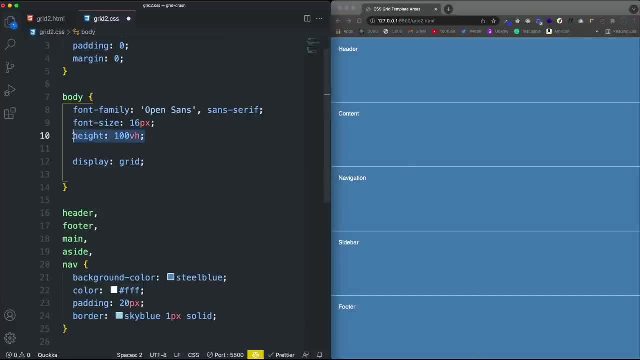 did this is because i set the height of the body to 100 vh. if i didn't do that, it wouldn't stretch. it wouldn't stretch like that, but i do want it to take up the entire viewport height. now for the grid areas. let's go ahead and say grid dash, template area. 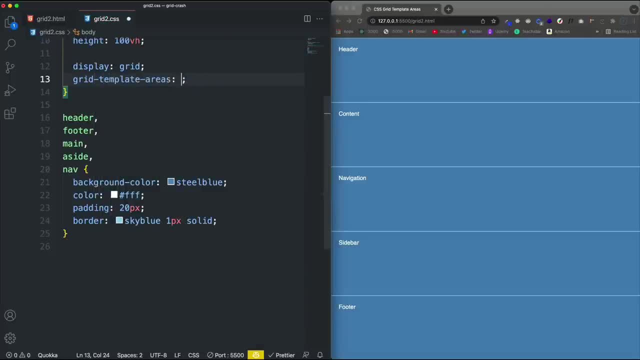 is the way we do. this is a little weird, but i think it's. it's cool because it's like a. it's like a physical representation of what we're trying to do. so the first row. let me bring back over our image so you can see exactly what we're doing. so the first row. 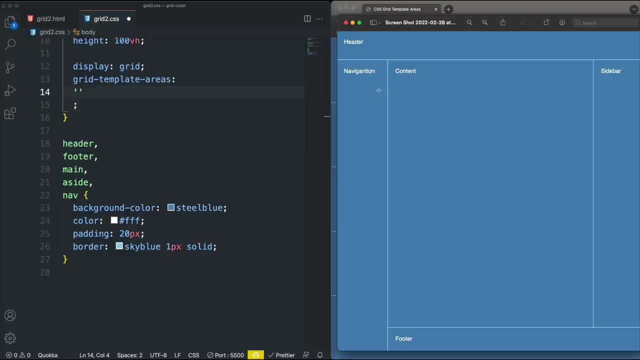 is going to be the header now. in total this: there's three columns right: one, two, three. the header we want to span all three. so the first row, let's say header, header, header. three times the second one, let's put in some quotes here: we want our nav, we want our content. now these words: 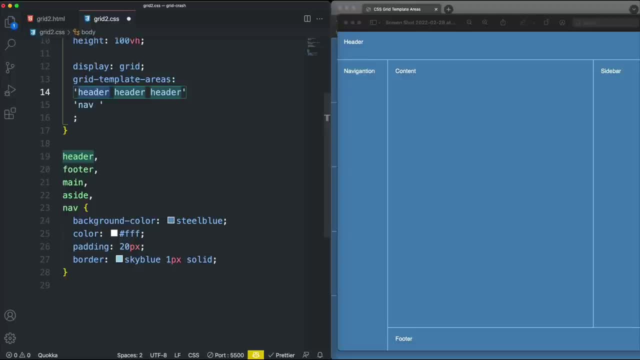 that i'm putting in here. these are going to be the grid areas. it doesn't have to be called header, we could call this anything, but i'm just being specific. so nav, then we'll do our content, and then let's say sidebar. okay, so that's the second, and then the third row is going to be. 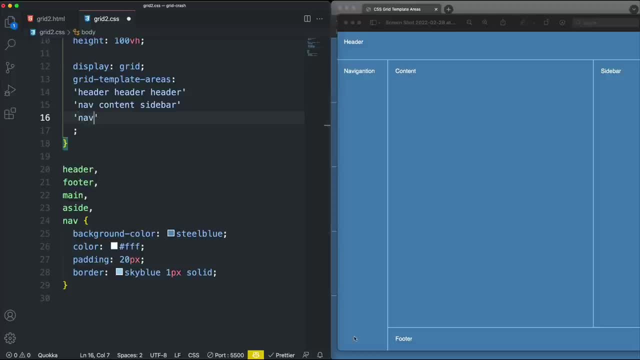 the nav again, because here the nav is going all the way down right, and then the footer i want under those two. so i would say footer and footer. so this is is like a text representation of how we want our layout. okay and hopefully that makes sense. header we. 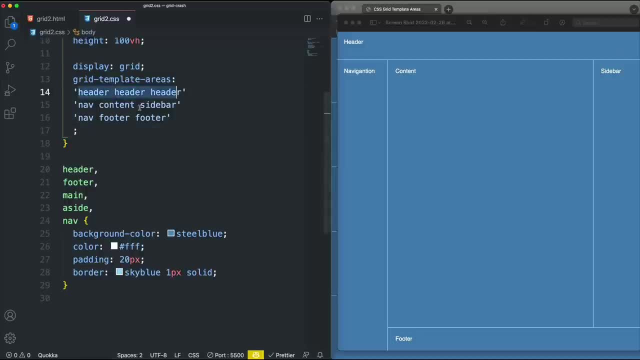 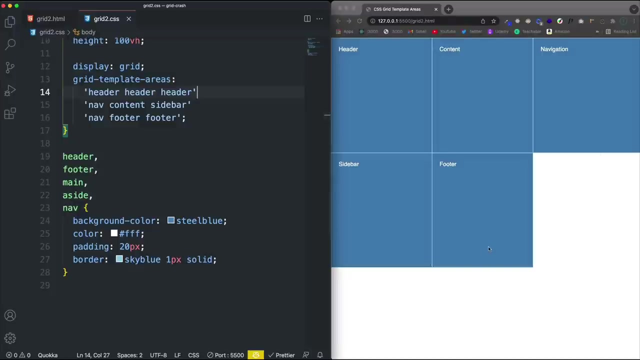 want to go all the way across the three columns, so we have it three times. we have the nav content sidebar, and then we have the nav footer, footer. all right, so let's get that out of there now, just saving this. it's not going to do anything except put them in side by side. what we need to do now is create. 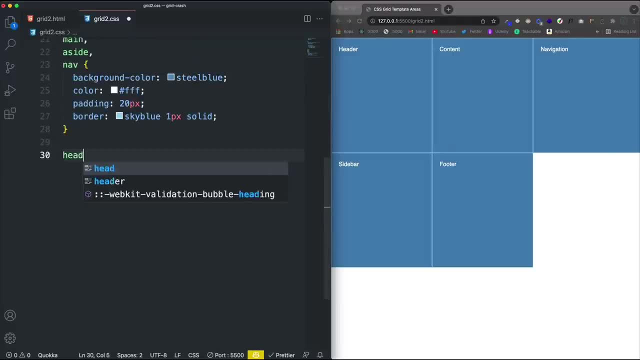 our grid areas, so we want to use our selectors, so we want the header tag and then we're going to set that grid area using the grid area property and we're going to set it to header. now, what i put here, this header pertains to this, okay, so this could be anything i could. 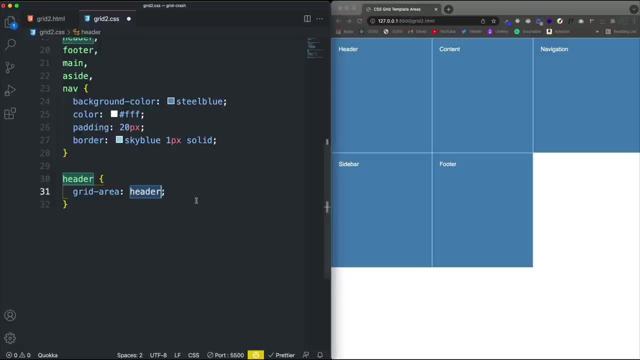 have brad three times here and then just have brad here. all right, as long as it's needed, per three. so this is something okay. i could have brad here and then just add brad here. i'm using the correct selector, so let's save that. and now you see, the header goes all the way across. 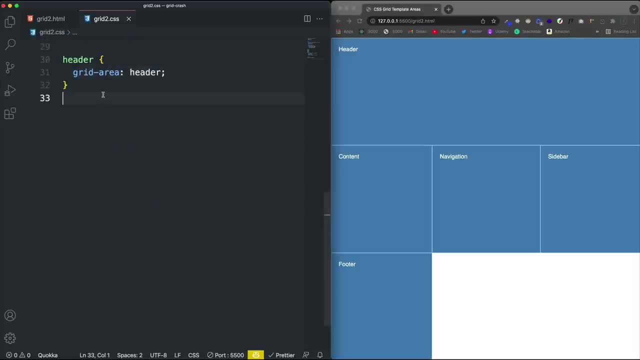 all right. so the next thing is, let's do the nav. so we'll say nav and set that to the grid area of nav, because that's what i called it. so now the navigation is going all the way down. so next we have what did i? we have the main tag and, i believe, the grid area i called content. 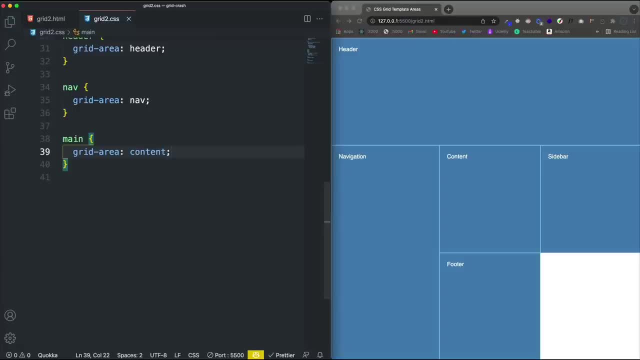 so let's say grid area content: not much difference there. and then the sidebar. so we'll grab that with a side and we'll say the grid dash area is going to be sidebar. and then finally the footer. and we want to set the grid area to footer. all right, so we'll save that. and now you can see. 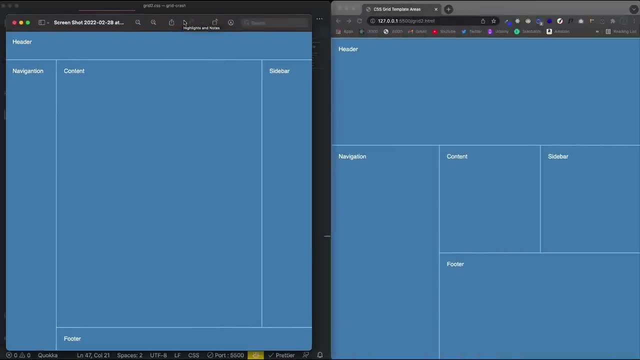 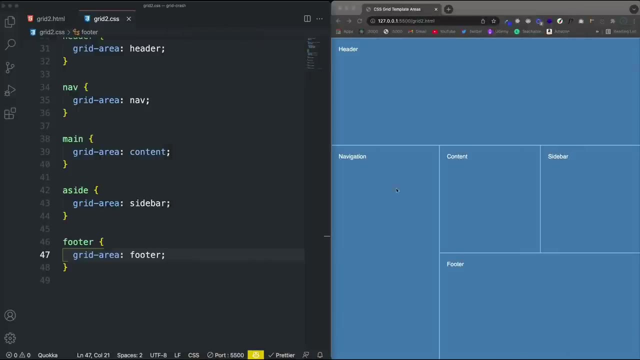 it's very similar to what i had have here, right, it's just the sizing. the positioning is all correct. now, if i wanted the footer to go all the way across here and have the navigation end here along with these content sidebar, i could just change this template area up here and instead of nav i could say footer and save, and now you can. 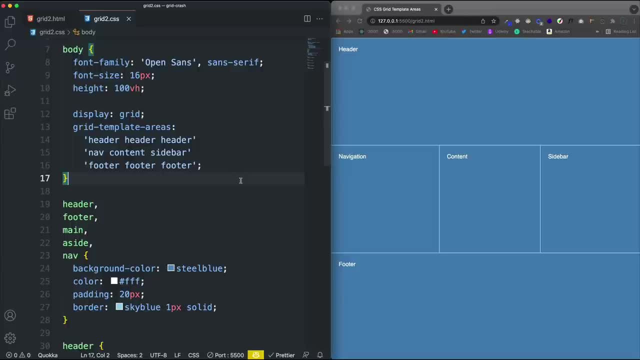 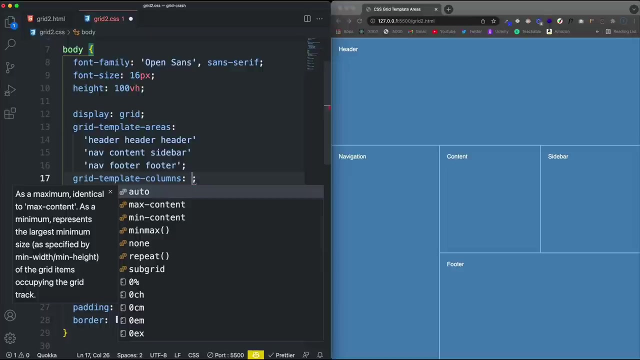 see the footer goes all the way across. all right, but i'm going to put that back to nav. now, as far as the the sizing, the width and the height, we can still use our grid template columns and grid template rows. so let's say grid dash template columns and i'm going to set it to one fr and 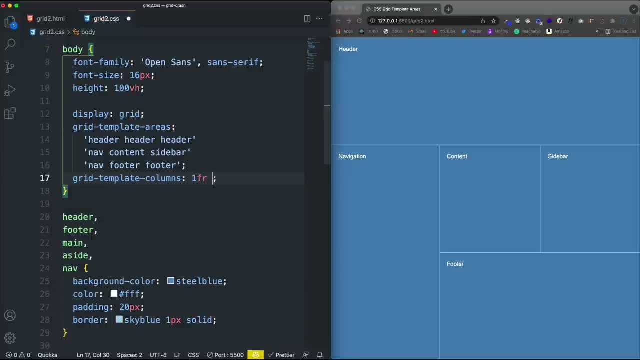 then the middle, the main content. that should probably be the widest right. so we'll do four fr and then the sidebar. we'll do one fr. okay, we'll save that. now you can see, the content is the biggest part. now. we also don't want the header and footer to be this. 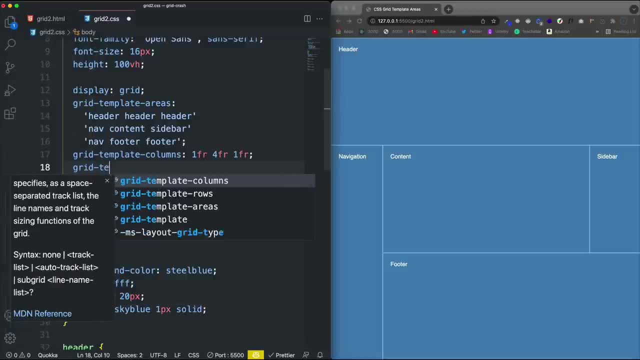 tall, and we're going to save that and set it to one fr, and then we're going to set it to one all. so let's use grid-template-rows here and let's set the header. we'll do 80 pixels and then let's just do 1fr, which is just basically the remaining area from the header. 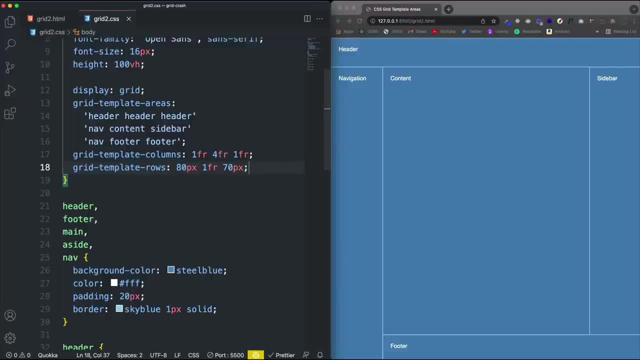 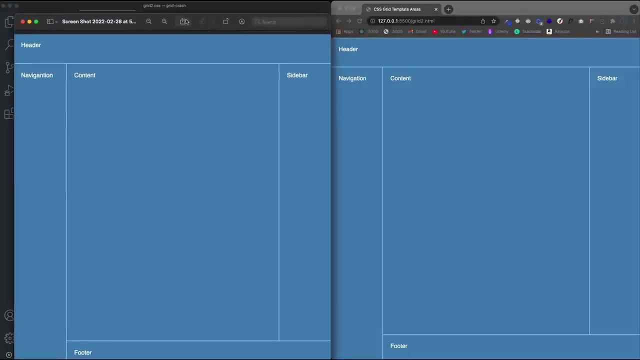 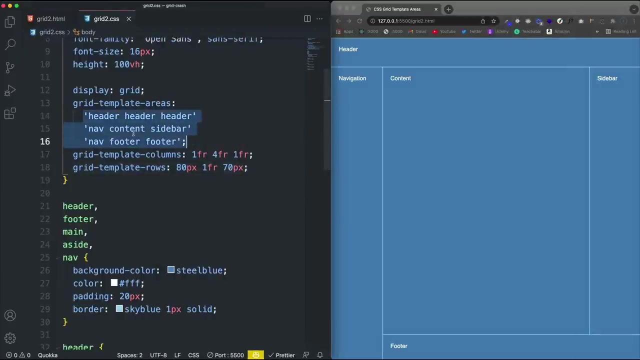 and then the footer, which I'll do 70 pixels. So now, if I bring my image over there, we go same exact thing. So I think it's really cool that we can lay things out like this. Now, you won't always use this, I don't use this a lot- but if I were to create something, 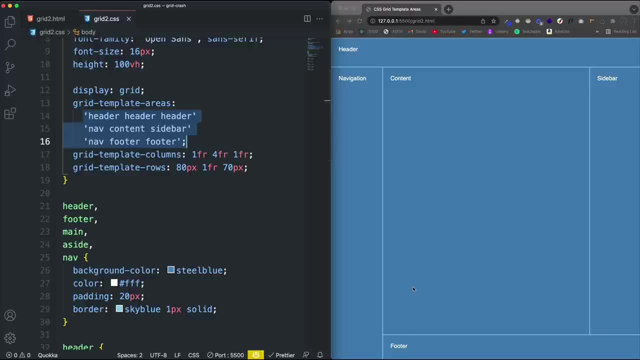 like this? I definitely would, And I've been doing web development for quite a while and those of you that have been too, you might remember when we did layouts like this with tables, like we would actually use HTML tables and style them to look like this and then doing it with floats and having the 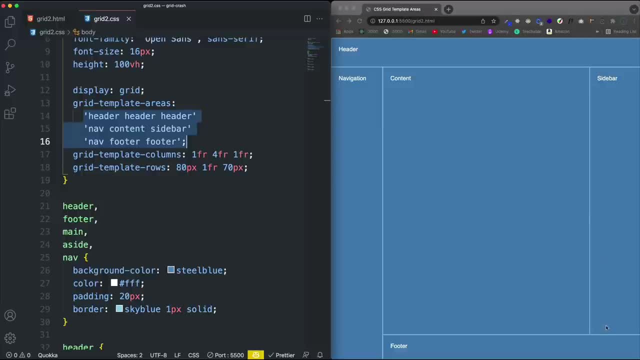 sidebar go up All the way like a color background color go all the way down. It was just a pain in the ass. So the fact that we have this kind of thing now, it's just. I mean newer people, just. 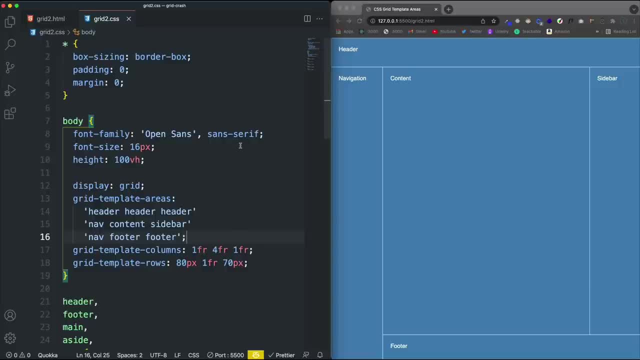 don't know how good you have it really when it comes to this kind of thing, But I think that's pretty much it as far as the properties that I wanted to show you. so now let's get into creating our little project. 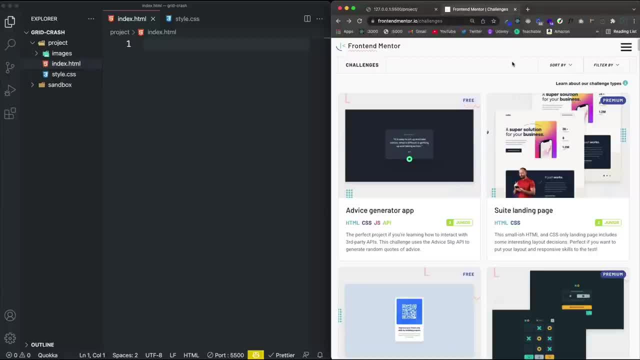 Okay, so we're going to get into our project now. The layout that we're going to build is: It comes from the frontendmentorio website, which is a really cool challenge website where you can build HTML, CSS and JavaScript projects, and there's some premium options, but there's 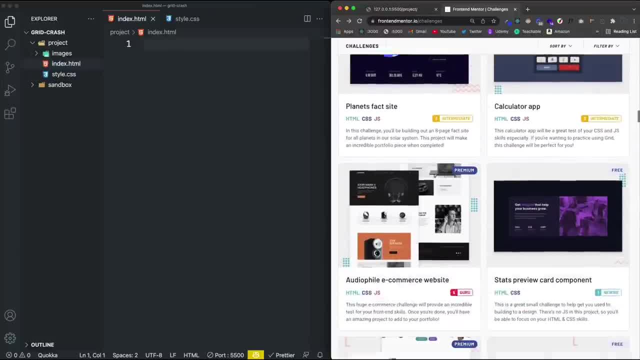 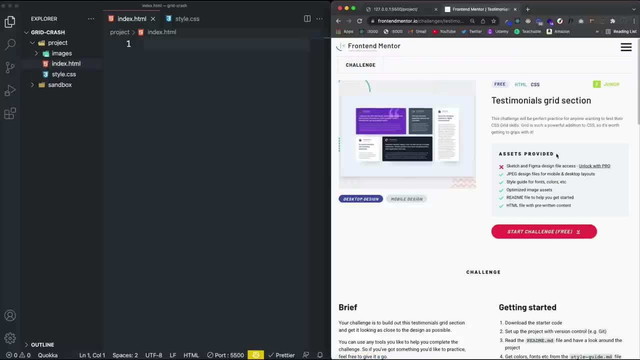 also a ton of free layouts here. So the one that we want to create is: let's see, it's the testimonials right here. So testimonials, grid section, and you can actually start the challenge and you can download all the images and design files and stuff. 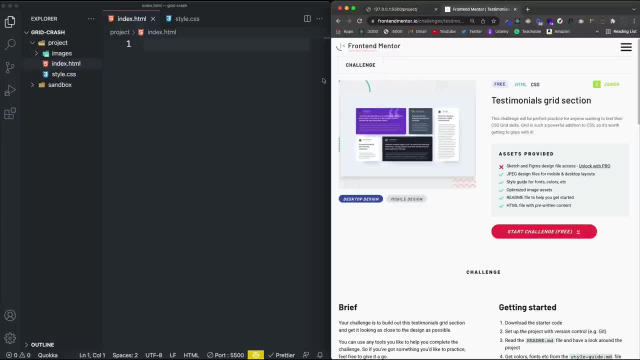 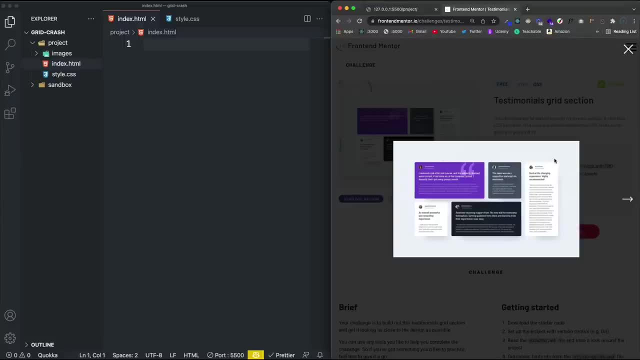 But I will have a repository in the description that will have the images and stuff that we need. All right, so it's going to look like this. I think this is a great example to use CSS Grid with, because we can use the 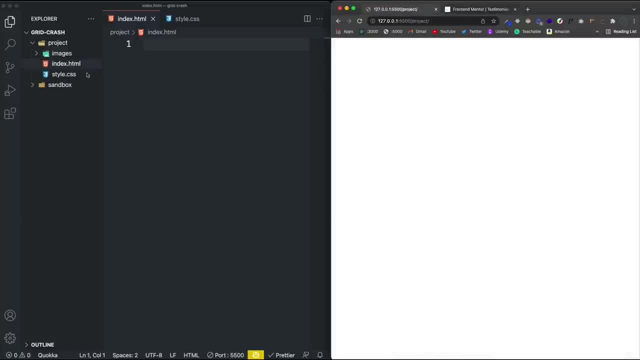 We can span columns and rows and all that, All right. so what I've done here is I've put all the other files that we've already created- the gridhtml, and all that- into a folder called sandbox, and then I have a. 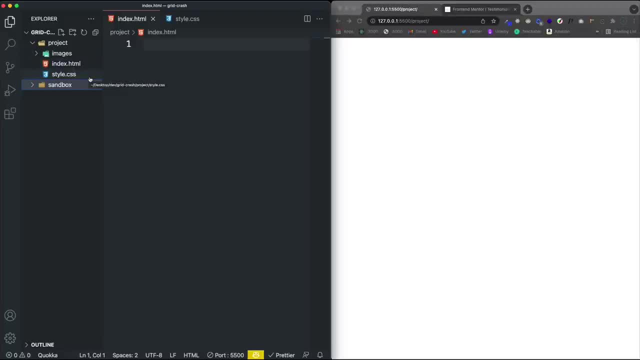 new folder called project, with an empty indexhtml and sandboxhtml. So I'm going to go ahead and do that. I'm going to go ahead and do that. I'm going to pay attention to my ability to filter these files, because I'm thinking. 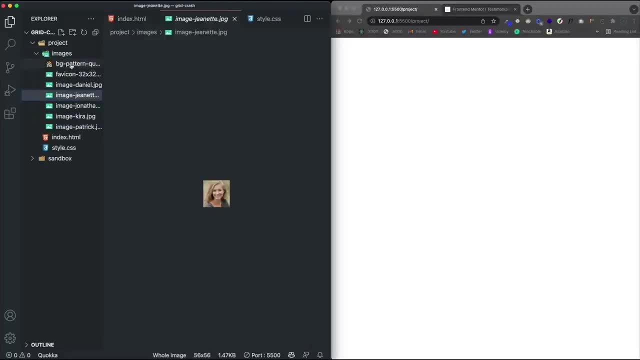 about how to do that And I'm just going to type this in here And I'm going to call this stylecss and then I just have the images of like the people and I have an SVG for this quote right here And you can get this again from the Frontend Mentor website or from my repository. 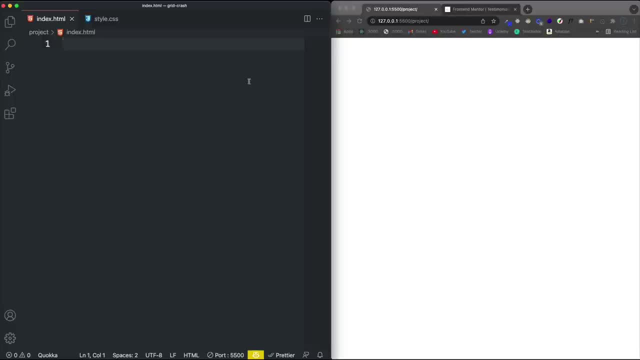 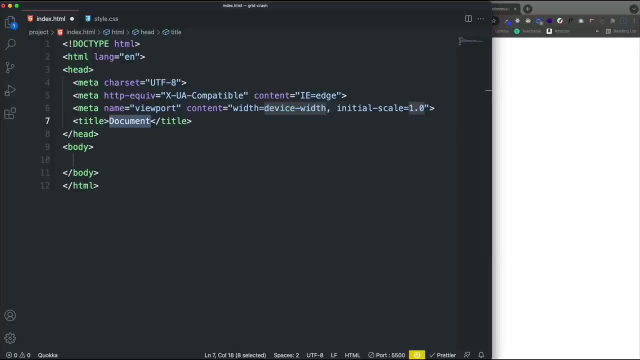 So let's go ahead and jump into our HTML first- And I'm just going to make this a little wider, since HTML takes up more room- And let's go ahead and add our boiler plate And we'll just say testimonials for the title. 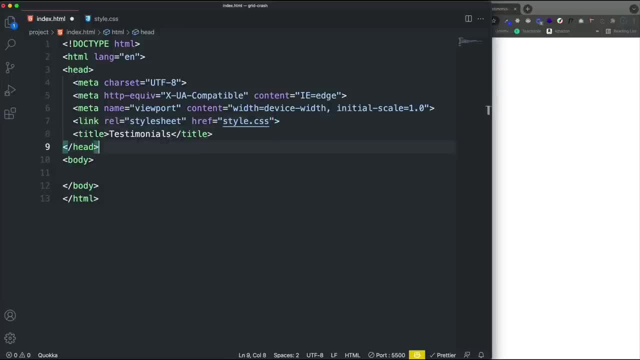 And let's link in our style sheet stylecss. And the way I'm going to do this is have a testimonials class And that's going to be our grid container And then inside that we're going to have a bunch of cards. 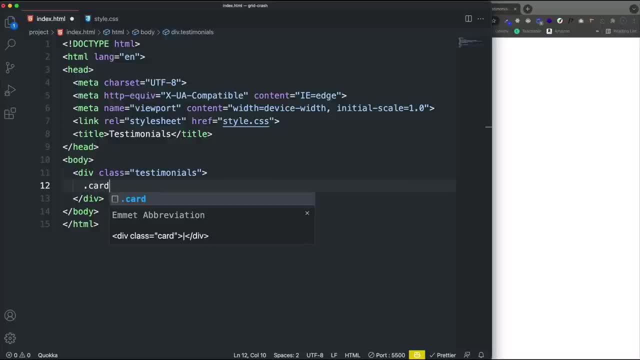 So first one will be a div. Let's give it a class of card And I'm also going to give it a class of card dash dash bg, oops, card dash dash bg dash purple. Because if you look at the project here, 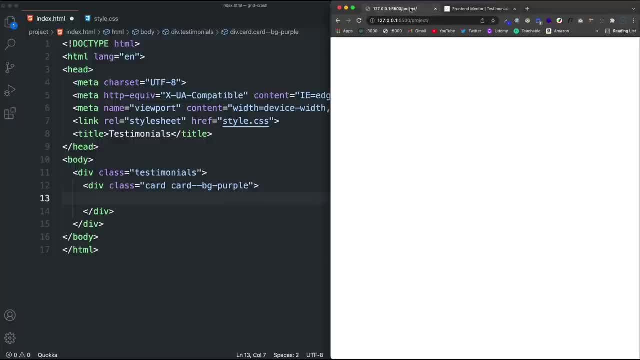 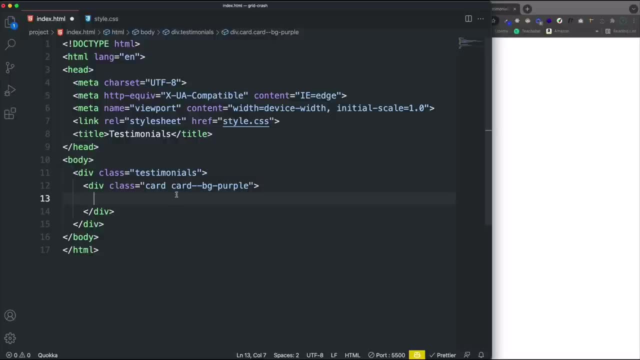 this one has the purple background, So we need to add a little bit of styling And I'm using the BEM CSS syntax or the B-E-M syntax, which I've been really liking lately. So inside the card we're going to have a header. 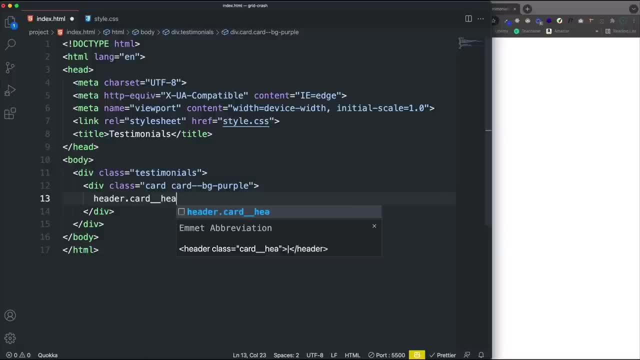 And let's give that a class of card, double underscore, header, And inside that we'll have the image, And we want images slash, and this one is Daniel. I'm probably just going to type this card out And then I'll paste the rest of the rest. 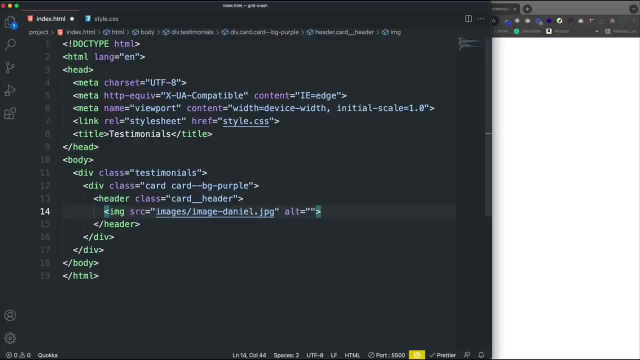 of them in and you can just grab it from the repo if you want. So let's add a class here of, let's say, card double underscore image And then underneath that we're going to have a div And that's going to have the H3 with the name. 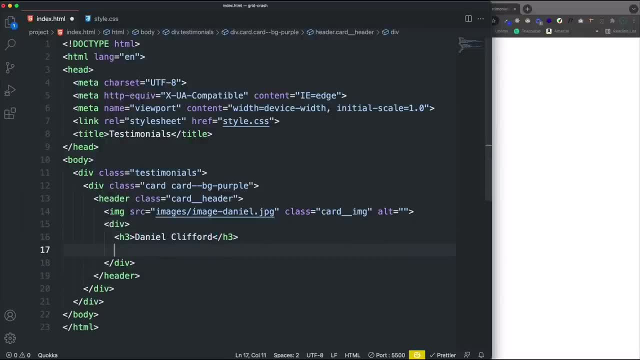 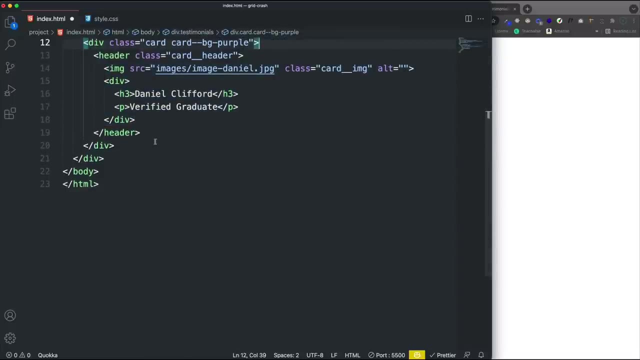 So Daniel Clifford, And then a paragraph with, say: verified graduate. And we'll use Flexbox to align like this here: This, This stuff here, All right. So underneath the header, let's see we have some more text. 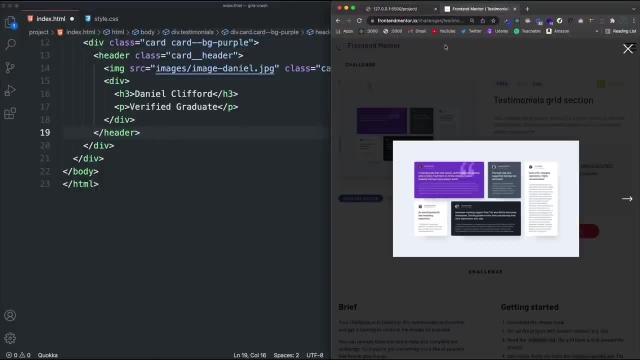 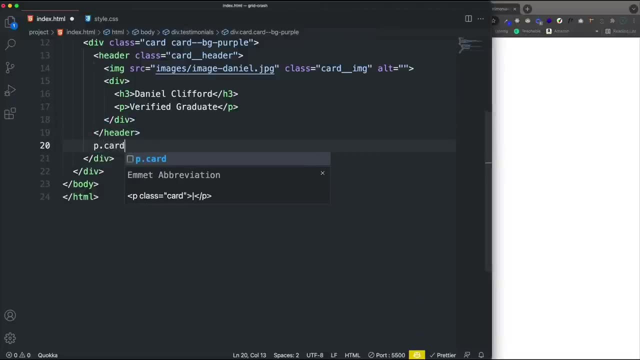 So basically, we have the large text, or the lead text, and then the quote, which is a smaller text. So under header we'll have, let's do a paragraph- class of card, underscore, double underscore, lead, And I'll get the actual text in a second. 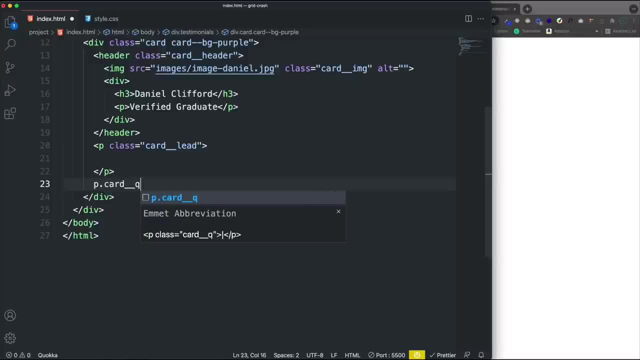 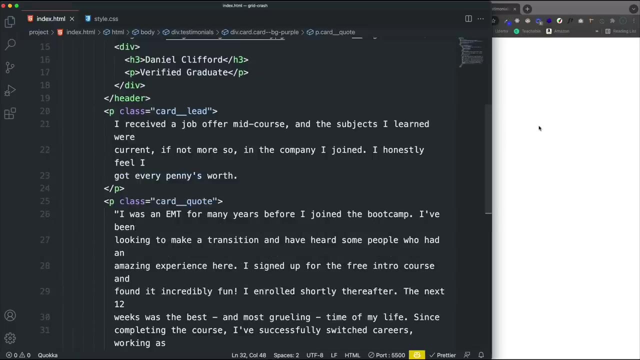 But then we're going to have a class of card quote, OK, And then I'm just going to grab those pieces of text, And if you just want to put dummy text, you can of course do that as well, And we'll save that. 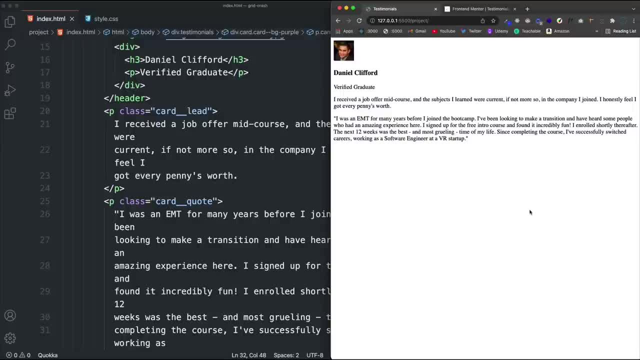 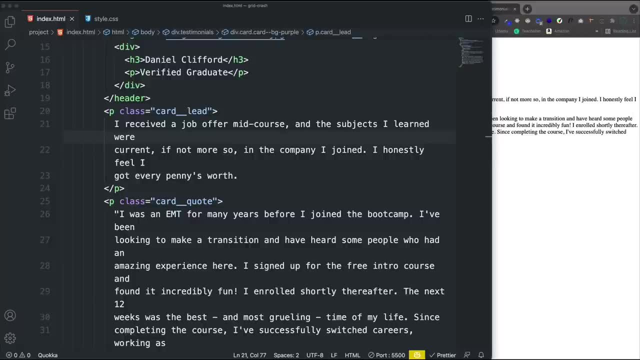 OK, so we have our first card, which looks absolutely horrendous, But we'll fix that in a little bit. So for the rest of this, let me just grab- I'm going to grab- the rest of the cards and just paste them in, because there's 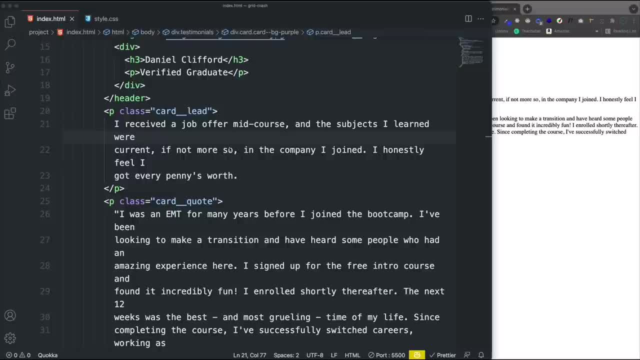 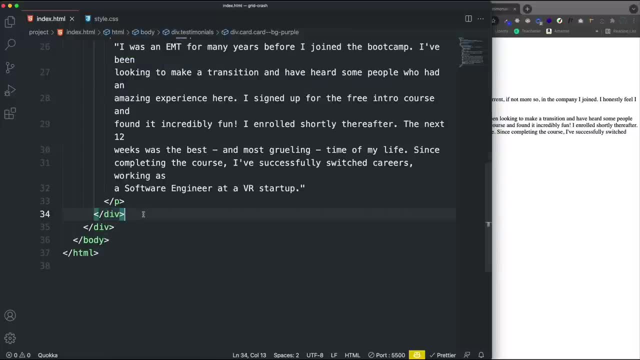 no sense in typing them out. They're all the exact same except for the content. All the classes and all that are all the same. So we want to go still within testimonials, But after this first div of the card we'll paste those in. 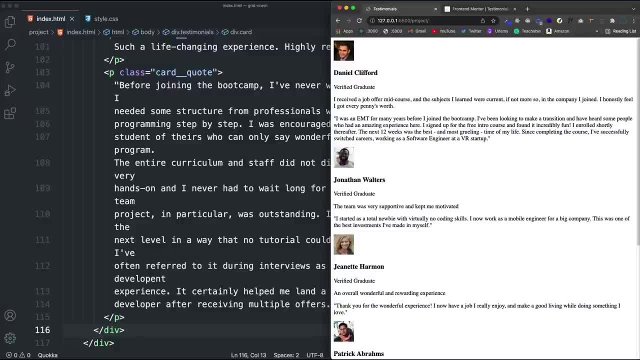 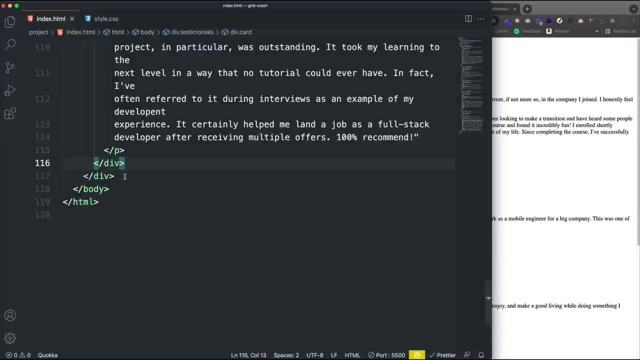 And now you can see we have all of the cards. And then I'm just going to add a footer just to give credit to Front End Mentor for this project. They're not sponsoring this video or anything, But let's say footer and say H3.. 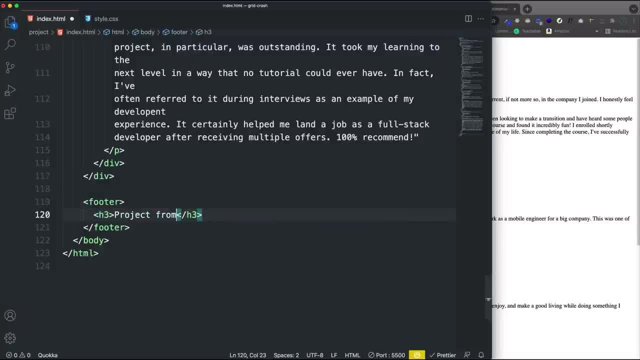 And we'll just say project. You don't have to do this, But I'm going to say project from, And then we'll put a link in here. Let me just grab the link. So this is the link to the actual challenge. 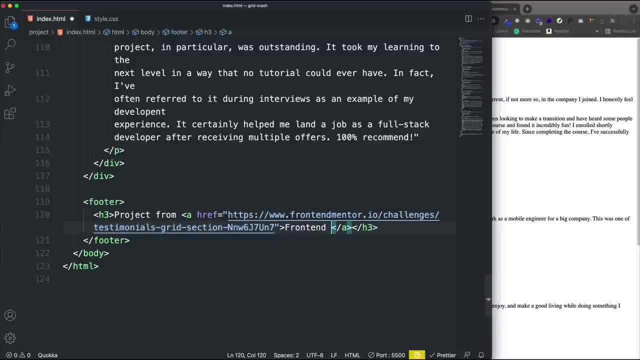 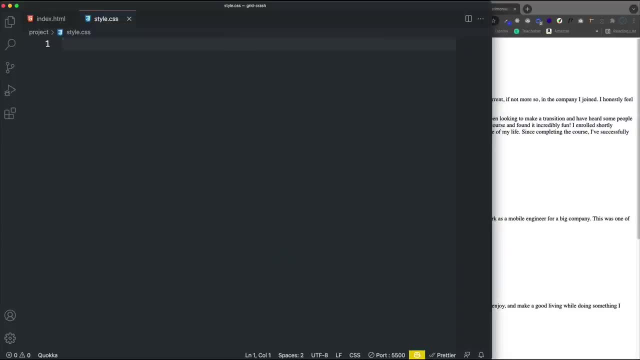 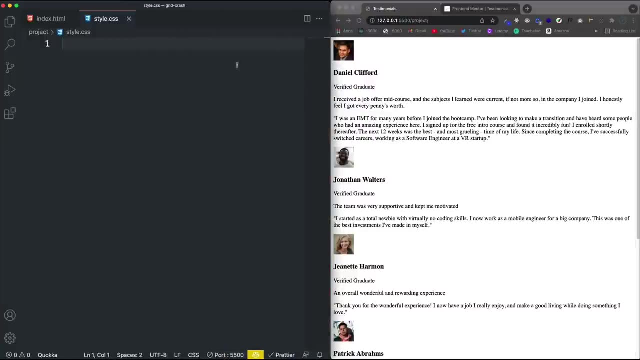 And in here we'll just say Front End Mentor. All right, cool. So now we go into our styling And we can make this a little smaller now, since CSSio doesn't usually take as much room, And I'm going to just paste in just a little bit of styling. 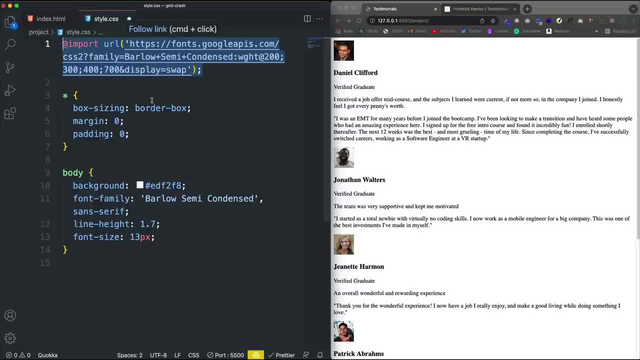 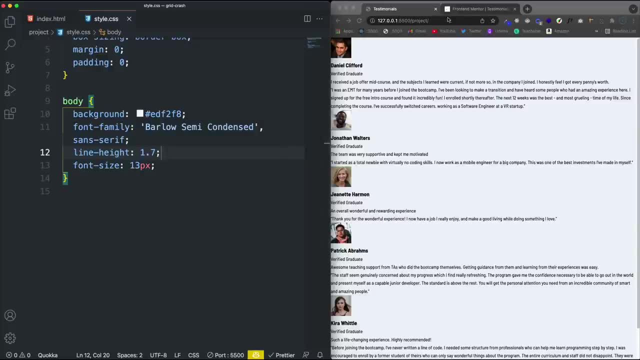 here We're importing the Barlow semi-condensed font and a reset And then just setting some background color and so on, And the text is pretty small. for this project There is a style guide when you download the resources from Front End Mentor, if you want to check that out. 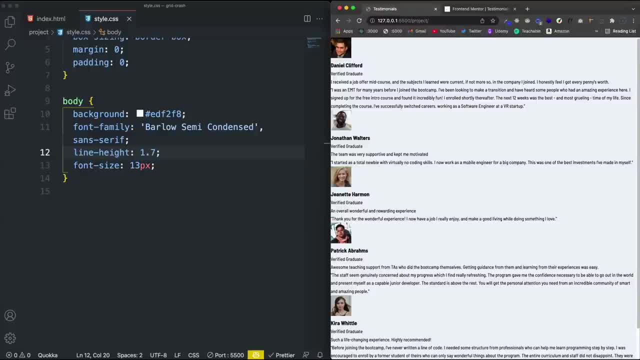 So I think first we should style everything but the grid just to get these cards. This is looking good- And then we can go ahead and add all the grid properties. So we'll start with the testimonials container. So let's at least add our max width. 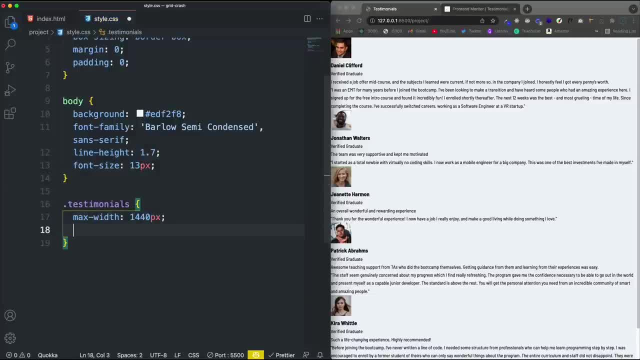 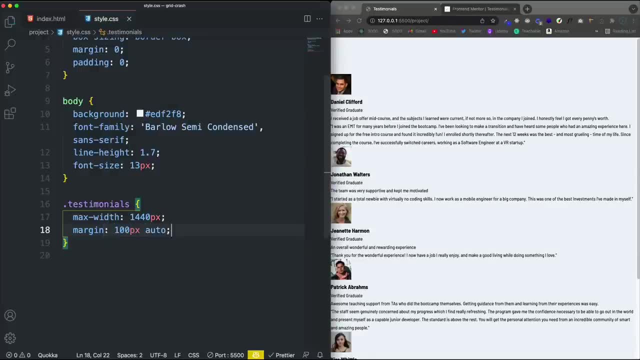 which is going to be 1,440 pixels going by the style guide. And then let's do margin. We'll say 100 pixels top and bottom and auto, And then this is where obviously we're going to have display grid and all that. 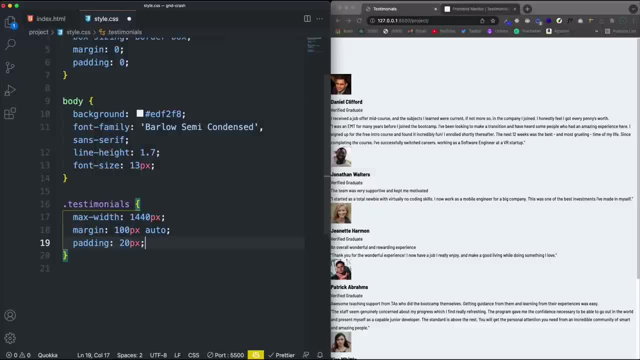 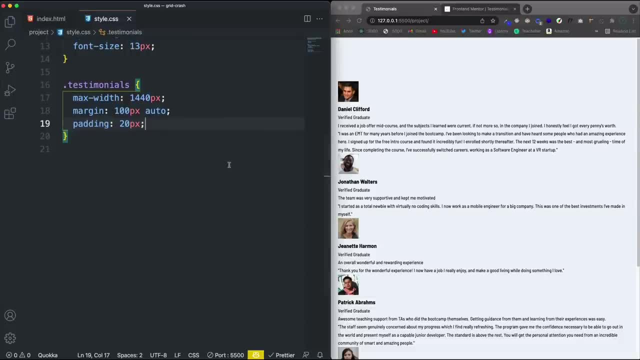 But we won't do that just yet And I know what we're doing for the next 10 minutes or so has nothing to do with the grid, But it's part of the project. So I like to do things from start to finish and not just paste things in. 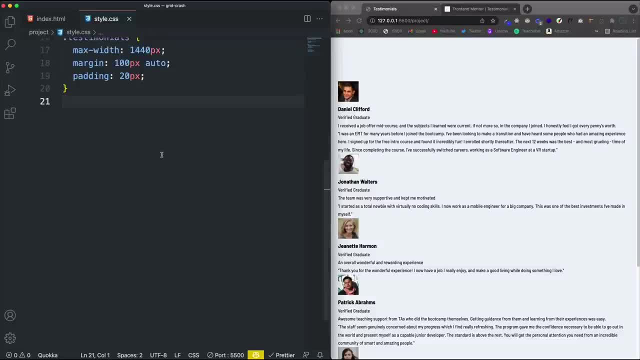 So you might learn some other stuff along the way. So let's grab the class of card, because we know that that's on all of these And we're going to add background. So the initial background color is going to be white, So we'll say white. 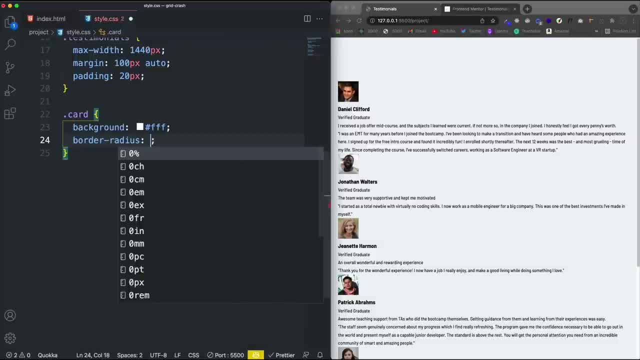 And then let's give it a border radius. We'll do 10 pixels- Whoops, 10 pixels. And then I'm going to add some padding- 30 pixels of padding- And we're going to have a box shadow. So I'm going to just paste that in. 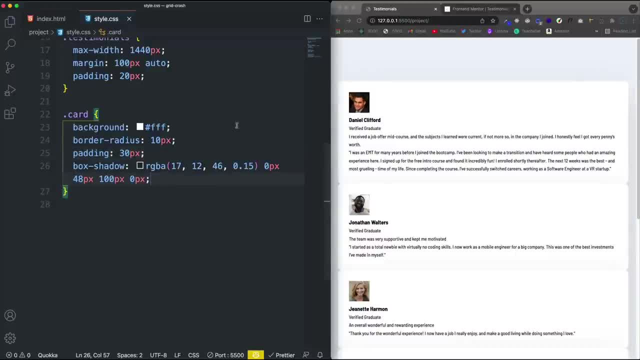 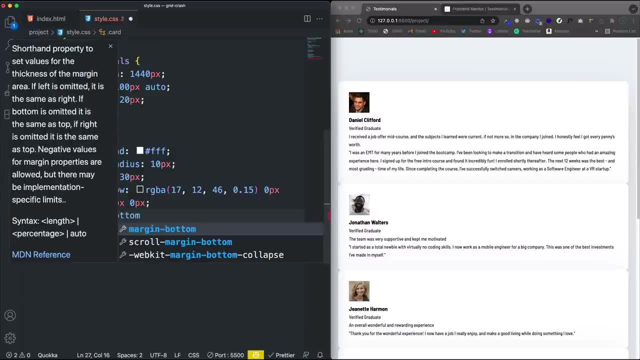 So I have to type that out. And if you want to change any of this stuff, obviously you can. And just for now I'm going to add a margin-bottom to the cards, just to separate them a bit, But we can get rid of that. 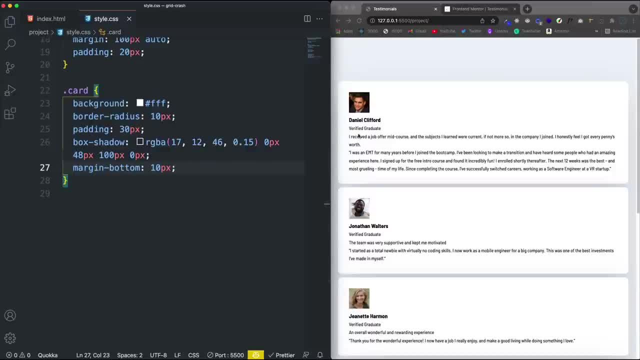 OK, Let's do that after. OK, So the header, which is the image, and then the div that has these two pieces of text in it. I want to use flexbox on that to align, And that's what I was talking about when we started the video. 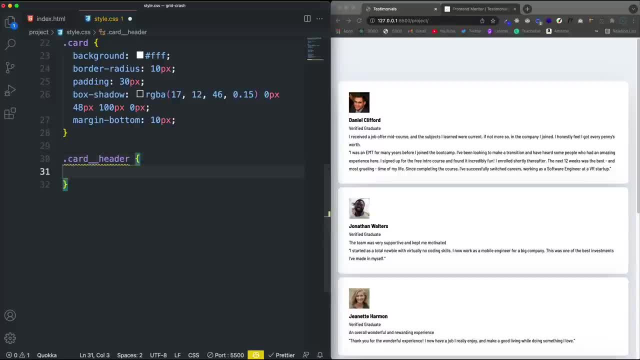 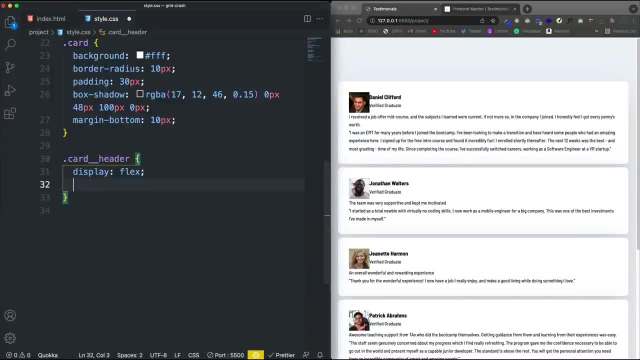 and I said where I use the grid and where I use flexbox. So I'm going to display that as flex And it's going to put the text right next to the image into a row. Let's use align items Center to align vertically. 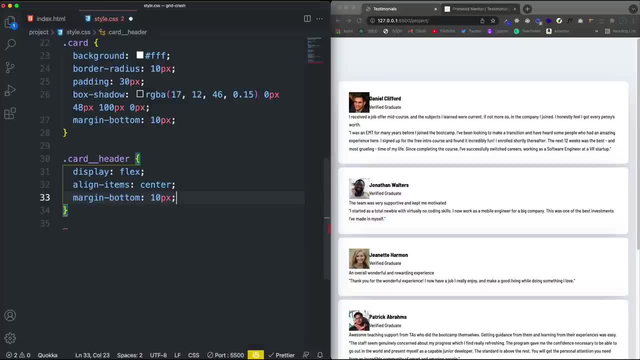 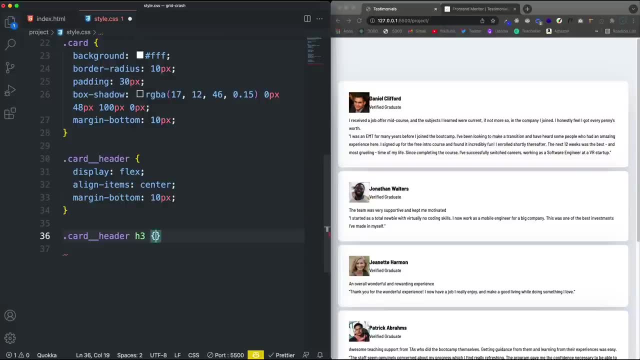 And let's add margin-bottom 10 pixels. And then let's grab the card header H3, which is the name, And we'll go ahead and just set that font size to 15 pixels. And let's see, We'll just grab this and just grab that and bring that down. 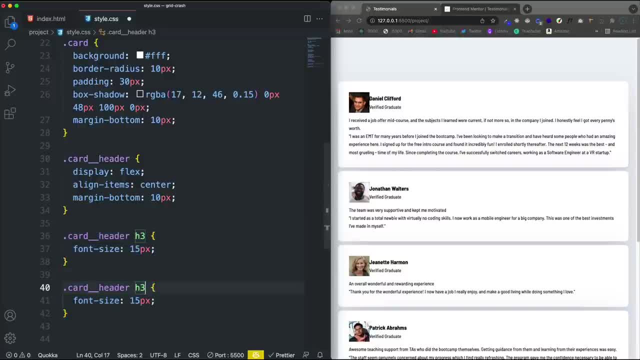 And I want to do the paragraph OK. So I'm going to go ahead and just set that in the card header, which is that verified graduate And that's going to be a little lighter. So we're going to do opacity and set that to 50%. 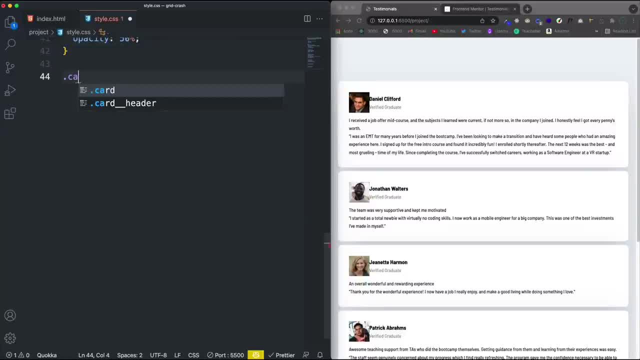 OK, And then for the image that has a class of card, double underscore, IMG, And we're going to set the width- let's say width of that, to 40 pixels, And then We're going to set the height to be 40 pixels. 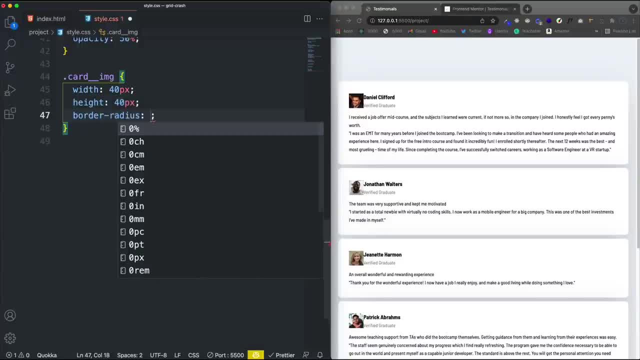 And let's make it rounded. So set the border radius to, let's do 50%, OK. And then we want like a light purple border, So say two pixels solid And the color for that is going to be 996ED9.. 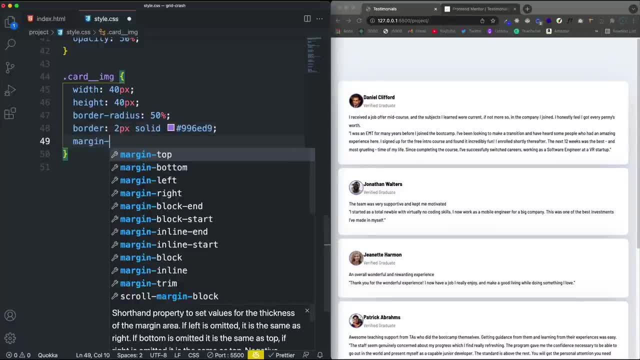 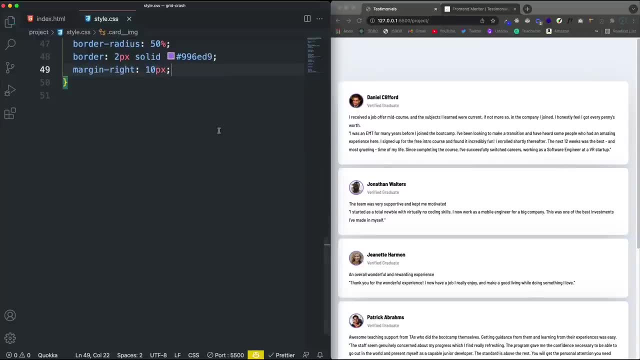 All right. So now we have the border, And then let's just add some margin right to push the text over. So we'll do 10%, 10 pixels. All right, So that's our header. Now for the text we have lead. 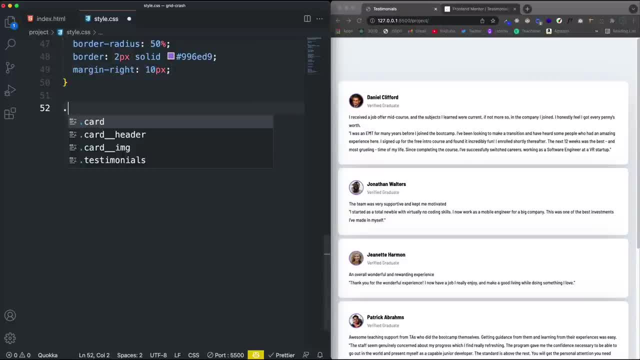 This is the lead And then this is the quote. So let's grab the- we'll say card- double underscore lead And for that we're going to do font, say font size of we'll use rem units here, 1.5 rem. 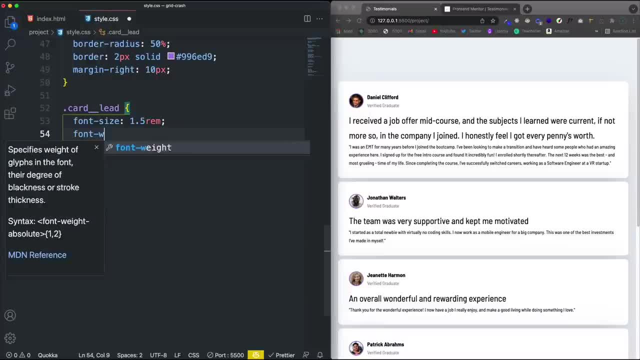 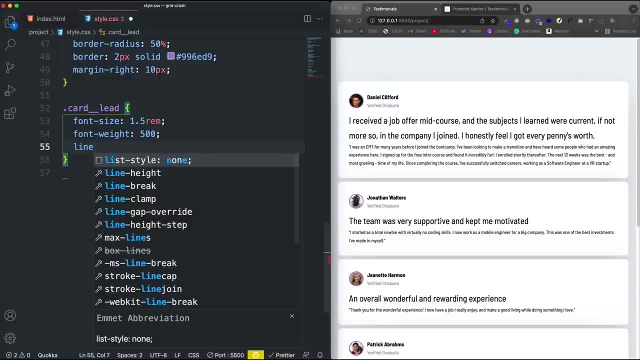 because it's going to be quite large, And then the font dash weight is going to be 500. And let's change, let's add the line height for that, which will be 1.3.. And then the margin actually no. 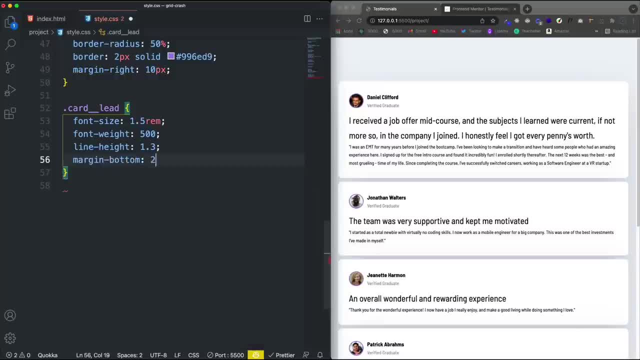 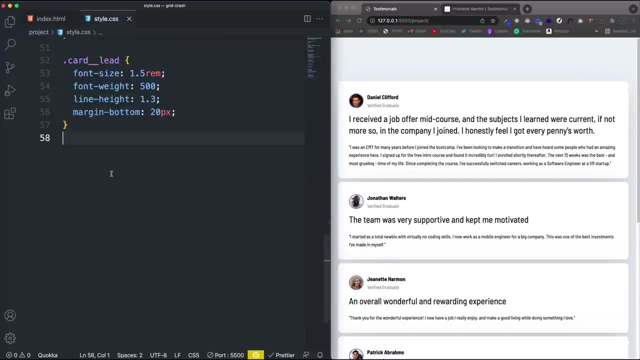 Yeah, let's do margin bottom 20 pixels. OK, And then for the quote I'll just copy this. So remember we have the card underscore quote And the font size for that. It's going to be 15 pixels, so really small. 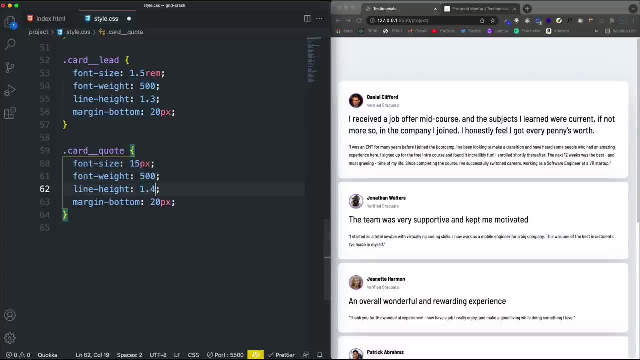 And then font weight's the same Line height, we'll do 1.4.. And then we're also going to make this lighter with opacity 70%. That's actually in the style guide as well. Now we want to, because these look pretty good now. 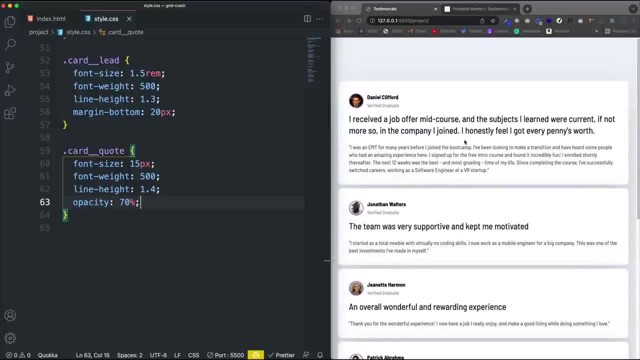 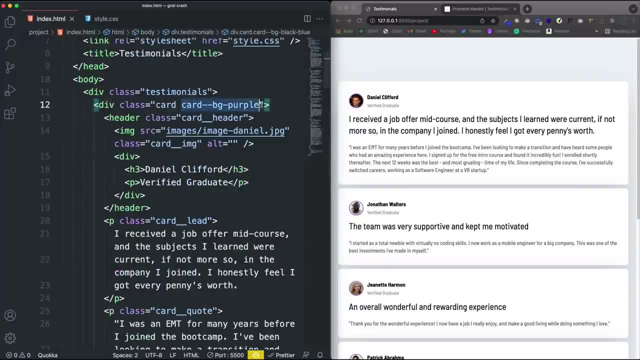 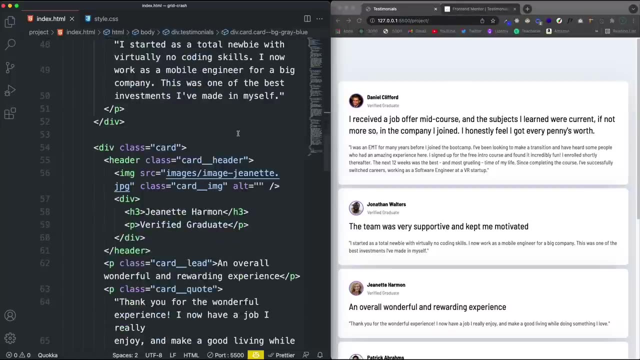 so we want to work on the different colors, so the different styles or variations. So we have the purple, Remember? the first one Is this card BG purple. And then we also have two others: This one here, card BG gray blue and card BG black blue. 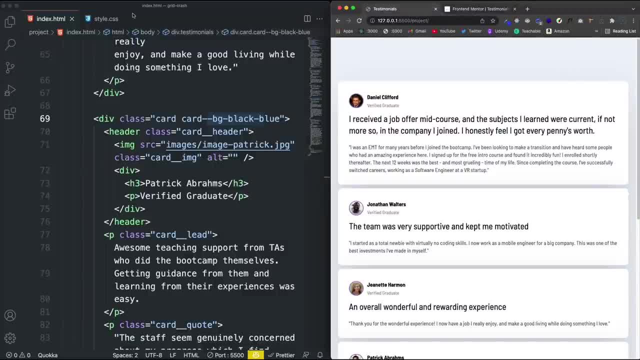 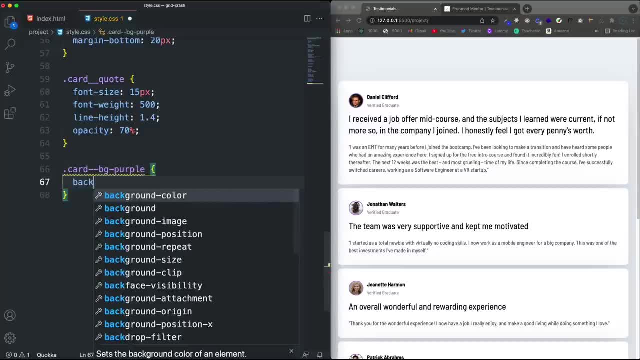 So here this is the gray blue, That's the black blue and the purple, So let's take care of those. So say BG purple And for this set the background, And the background is going to be HSL, So that's taken from the style guide as well. 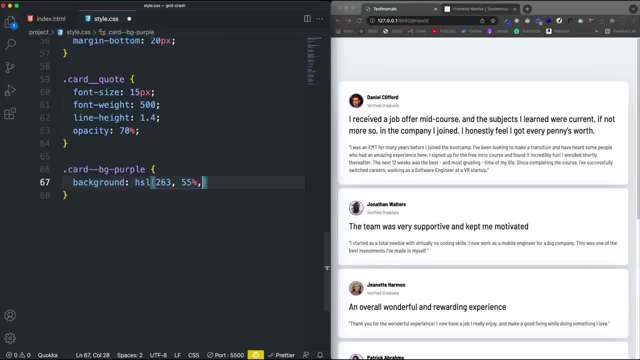 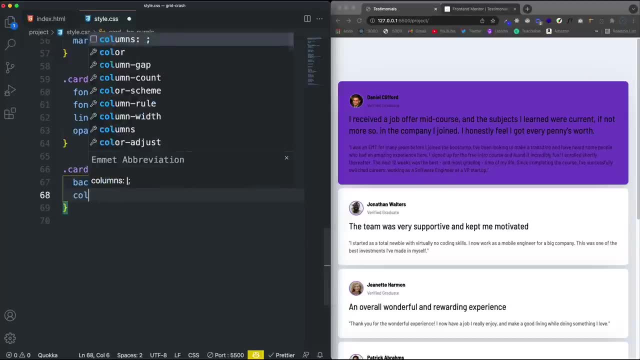 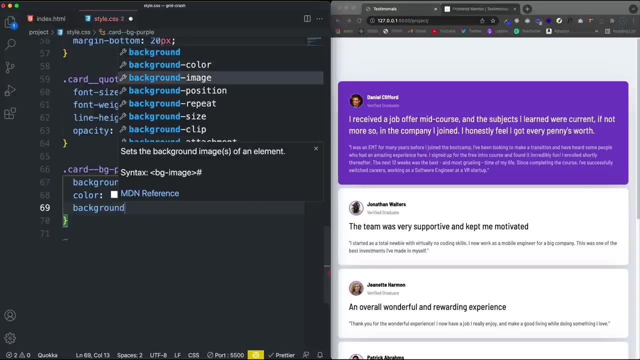 from Front End Mentor. Let's do 263,, 55% And then 52. Is it 50?? Yeah, 52%. So that's our background, And then, of course, we want to lighten the text, And then this one actually has a background image of the quotes. 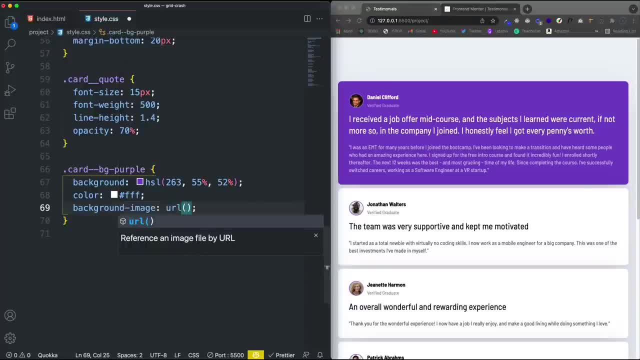 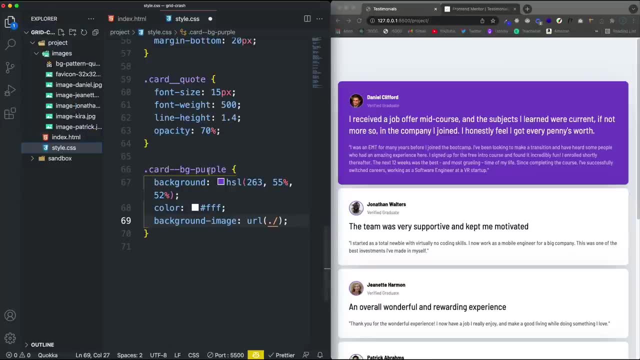 So let's say URL And we want to go. let's see, just dot slash, Is it? Where is it? Yeah, so I'm in style CSS, so we just want to go into images. Let's see Images. 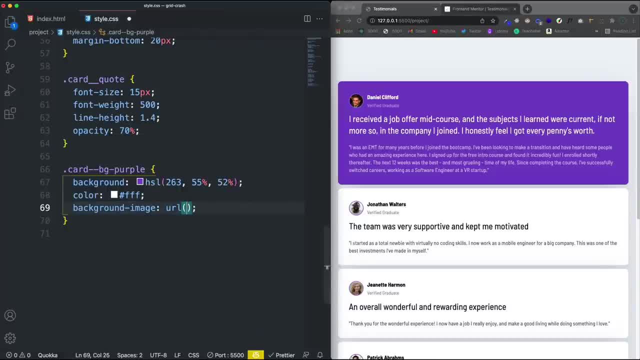 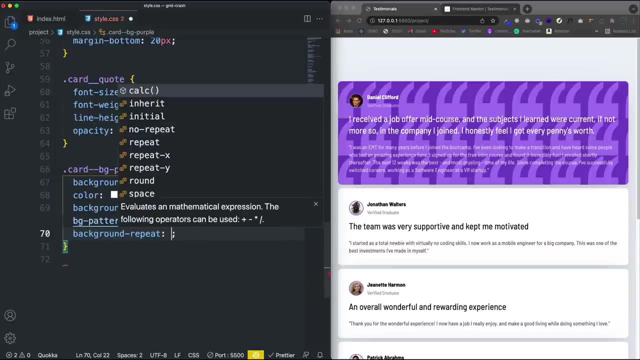 If you used a CSS folder, then you're going to want to do dot, dot slash. Let's do dot slash, images slash. And yeah, we want that. OK, so that doesn't look good. Let's do a background repeat and set that to no repeat. 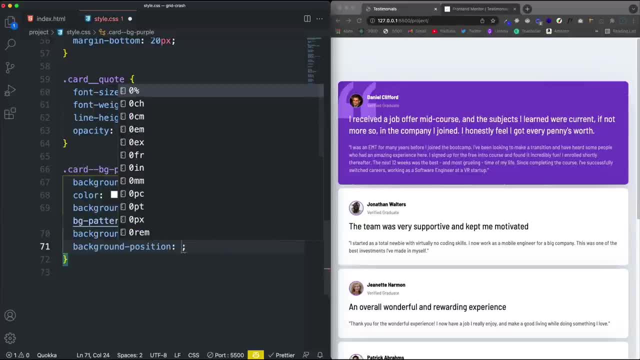 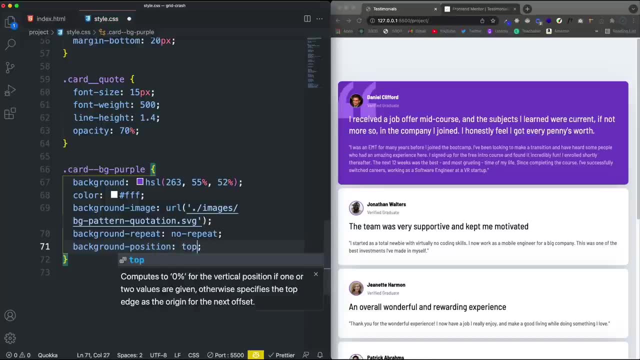 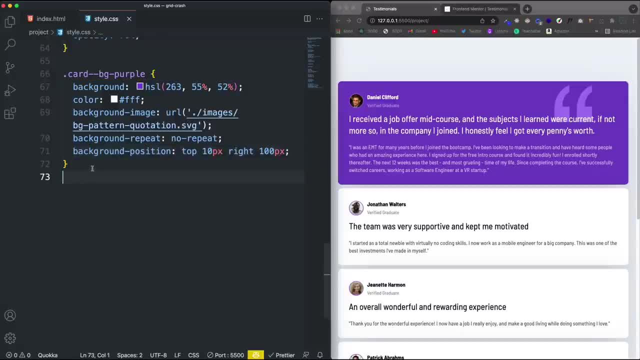 Yeah, that looks good. All right, now the other ones here. so let's just grab that And then we don't need the image for the other ones. So the color for this is going to be BG black. Let's do BG gray. 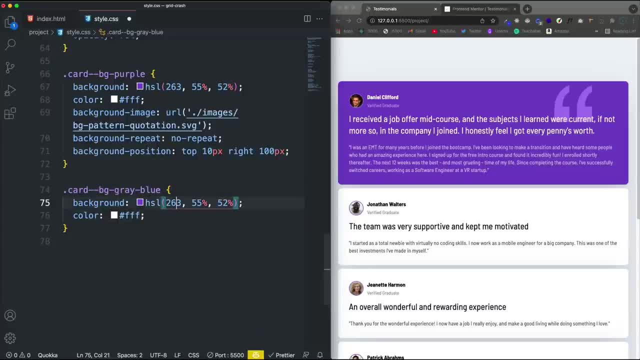 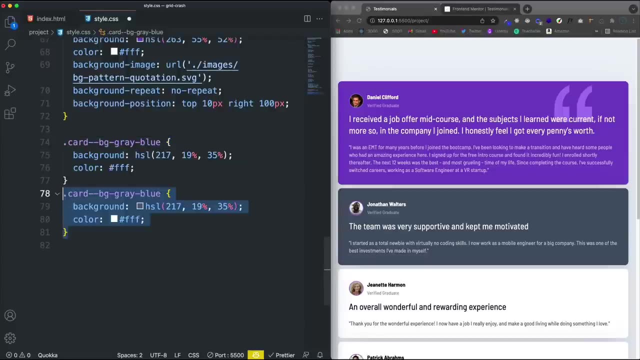 Yeah, gray blue, And the HSL value for that And the value for that is going to be 217.. 19% And then 35%, All right, and then we'll just grab that and bring that down And this one's going to be called BG- black blue. 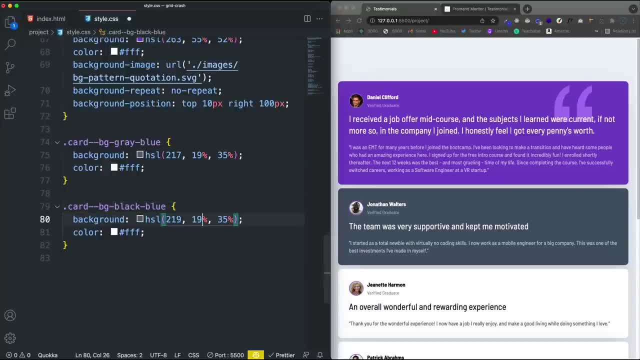 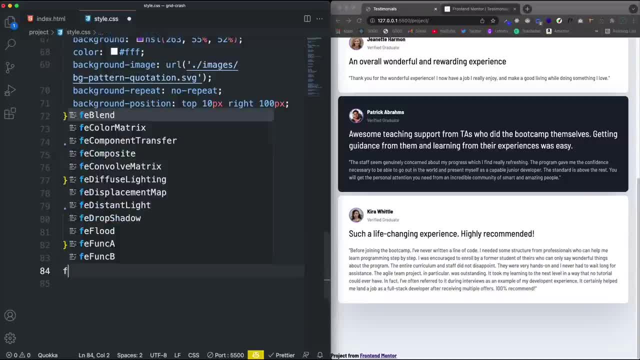 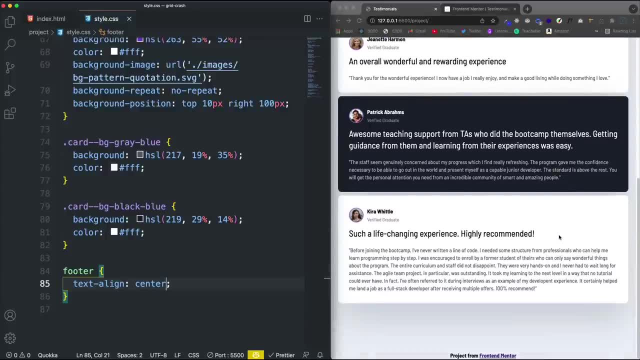 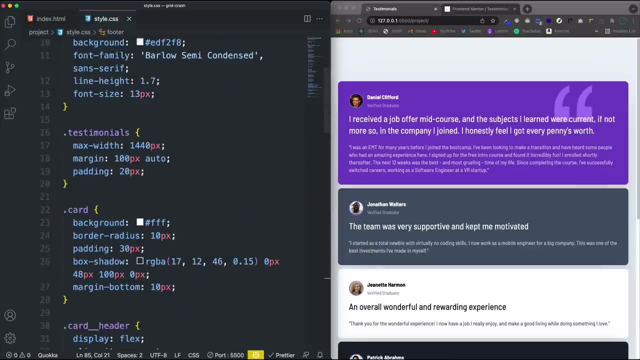 Oh, the footer down here. I do want to just center that. So I'm just going to say footer And let's text align that to the center. All right, so now for the grid. So we know that we have the testimonials up here. 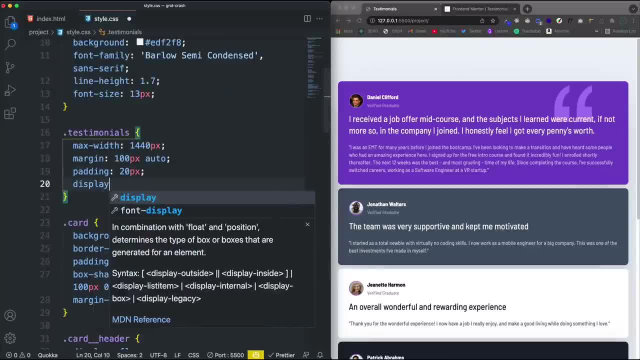 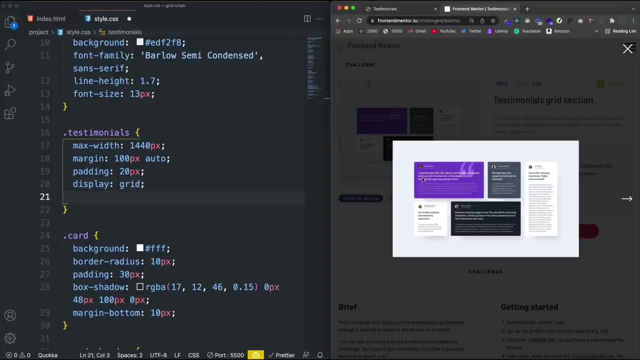 That's going to be our grid container, So let's go ahead and display grid And then we know we're going to need four across And you see only three items. But remember, this one is spanning. It's spanning across two lines, right? 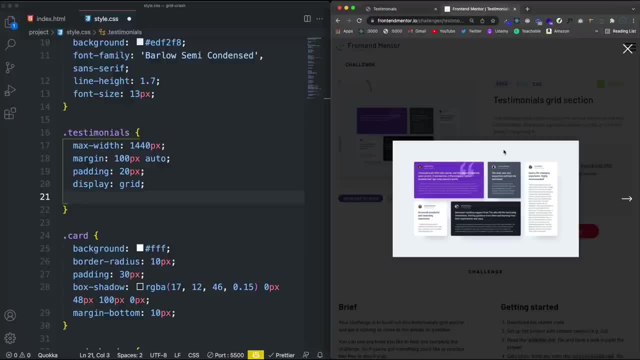 So it's going to be one, two, three, four, five, But it's going to be five lines, But the tracks it'll have four tracks. So let's do grid, Grid, dash, template columns, And we're going to repeat and say: repeat four times one FR. 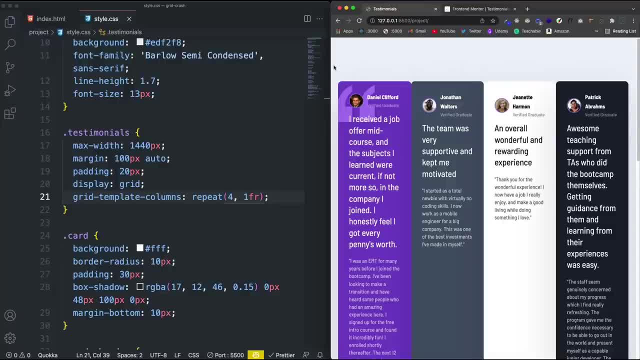 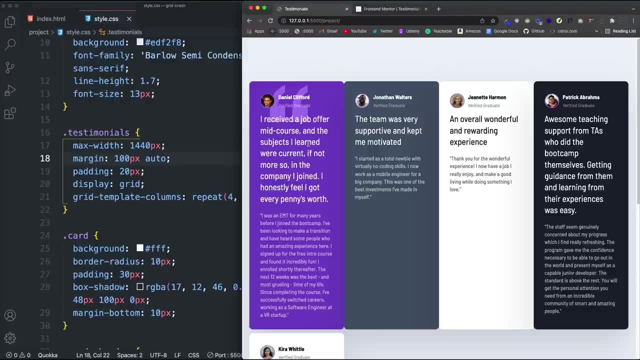 So let's take a look at that. All right, so we have four going across. We'll make this a little wider here. Now this one we want to span from. actually, let's open up the grid tools. So I'm going to just click that. 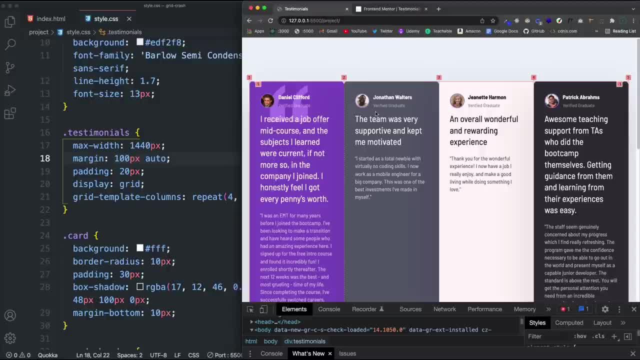 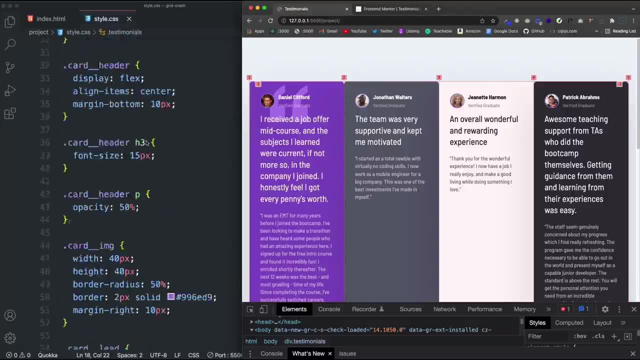 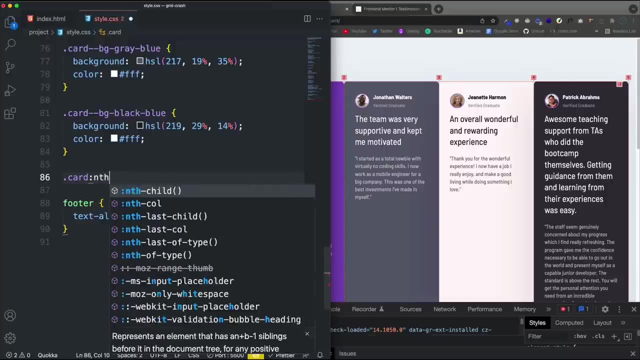 All right. so now we can kind of see what's going on a little better. So we want this one to go from one to three. So what we can do is go down here to the bottom and let's say dot card, And we want nth of type. 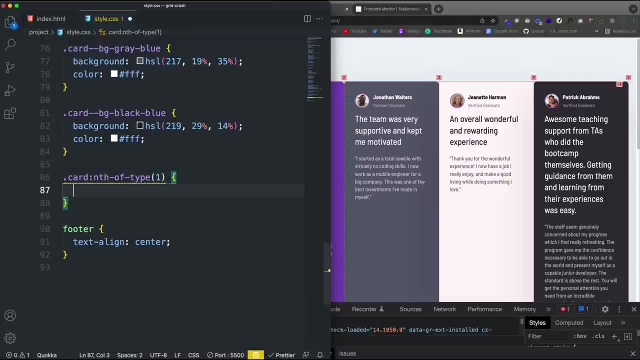 And we want the first one. So if you want to pause the video and try to do this yourself, I would recommend that. Of course you don't have to, but I would suggest it. But let's do column grid- column. 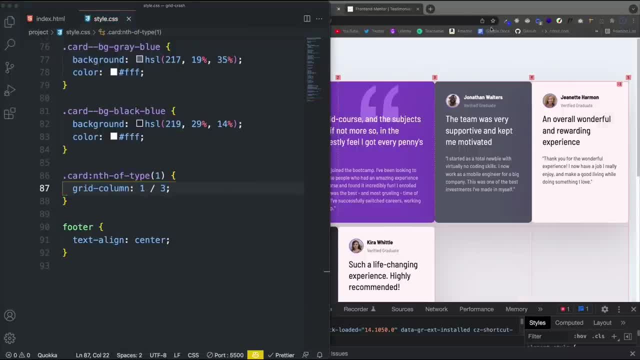 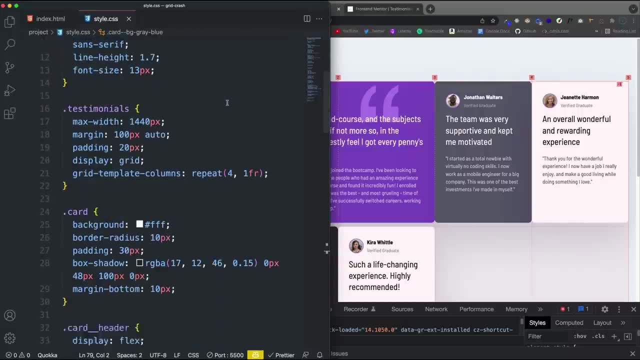 So one, two, three, All right, cool. So now that goes from one to three. Now I do want to add gap as well. So let's go up top here and where we have our display grid, We're going to add gap. 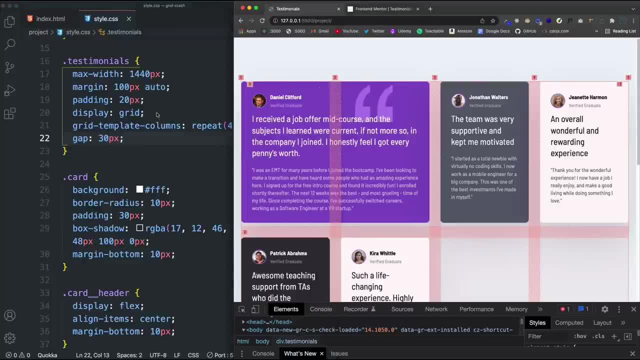 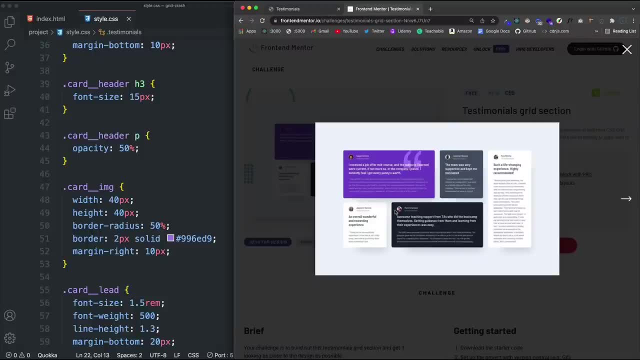 And let's do 30 pixels to split those up, And then I want to do Okay. So the fourth one, Patrick, we want to go from here. So Patrick will have grid column. This is going to be two, right. 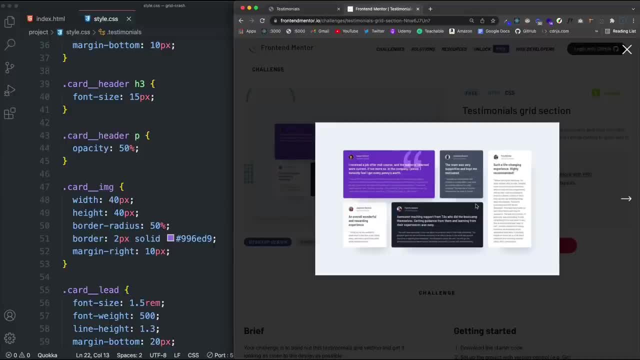 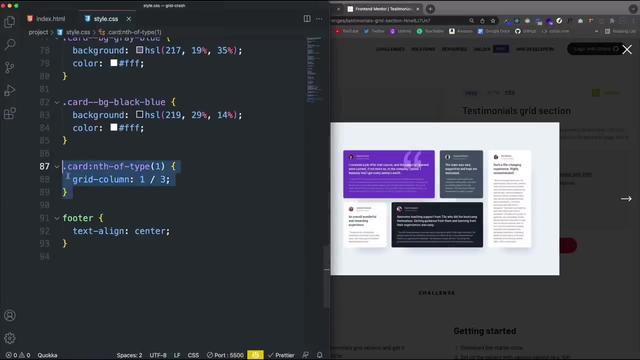 So one, two and then three and then four. So we want him to go from two to four as far as the column goes, And we want him to go from two to three as far as the row goes. Okay, So let's just grab that. 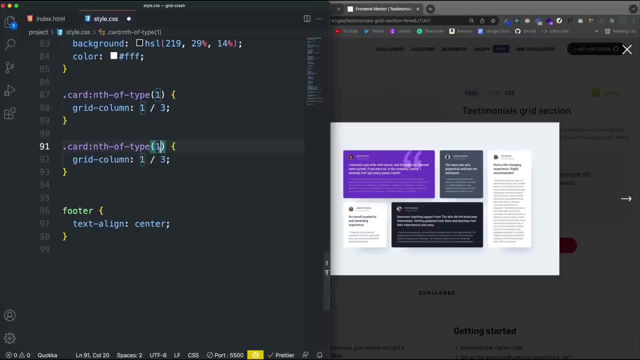 And Okay, And that's going to be four. That's the Patrick, the dark background here. So, like I said, grid column is going to be two. We want it to go two to four and then grid row We want to be from two. 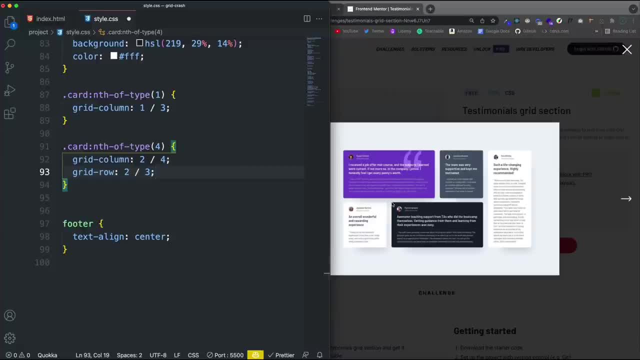 So it's going to be two to three, like that. All right, So he's going from two to three as far as the row goes. Now, since it's it's just the next one, like two to three. we can, we can do this, but 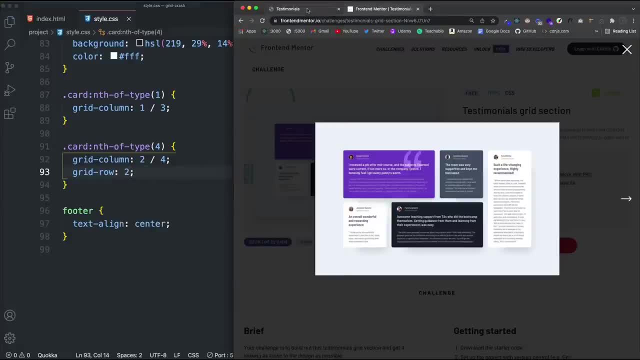 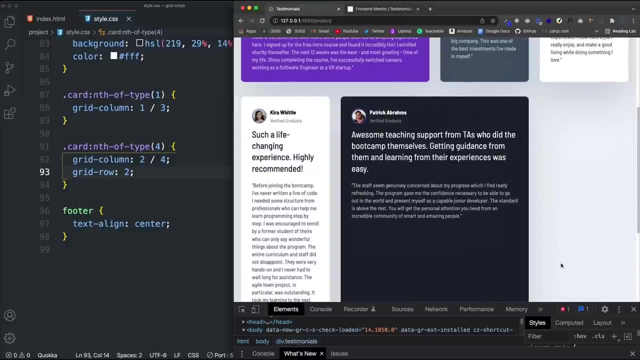 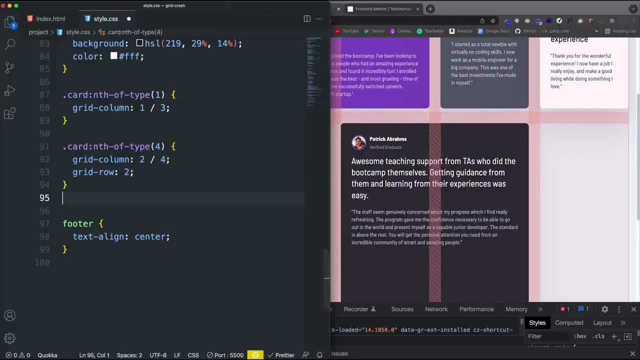 we can also just say grid, row Two, All right, So now, yeah, we have Patrick in the right place, And then the last thing we want is for Jeanette to go all the way down. Okay, So let's grab this, and Jeanette is five. item five: 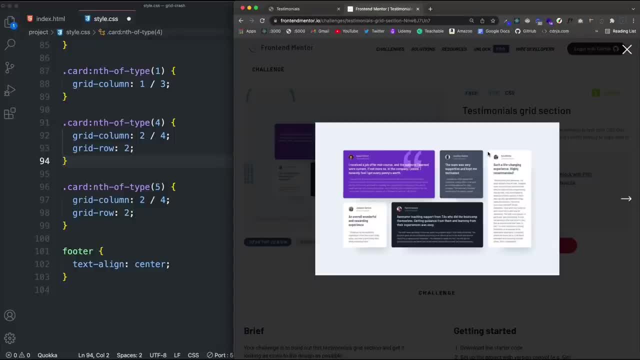 So grid column is going to go from four, four to five, right? So this is one, two, three, Four, five. We want to go from four to five, So grid column, And since it's just four to five, we can just do four. 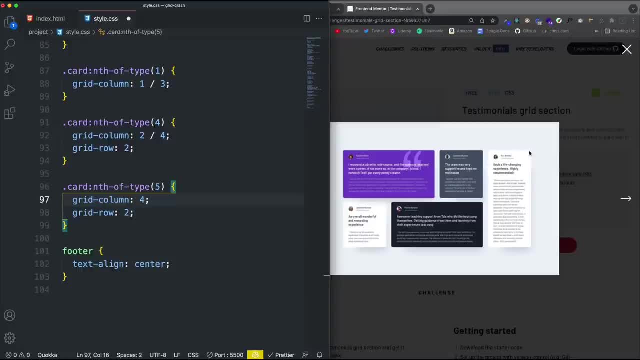 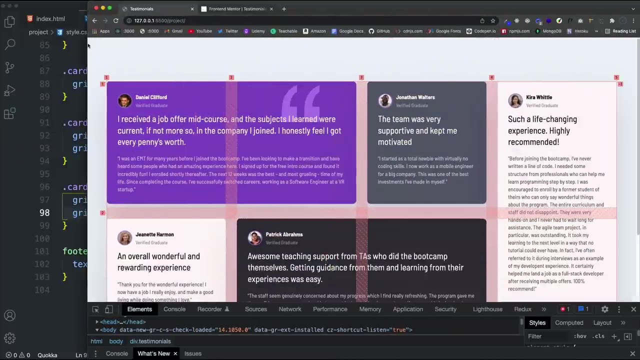 And then as far as the row goes, which is this way, we want her to go from one to three. So grid row is going to be one, three save that and there we go. please stretch this out a little bit, It should look. 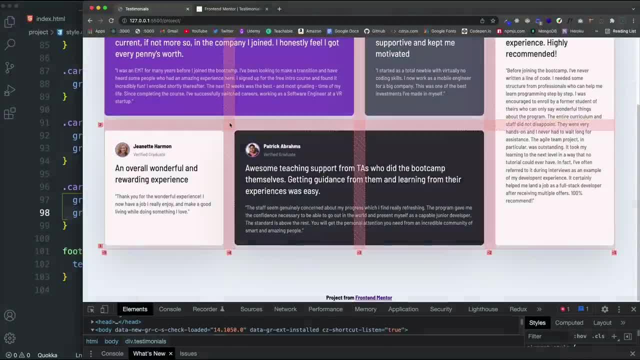 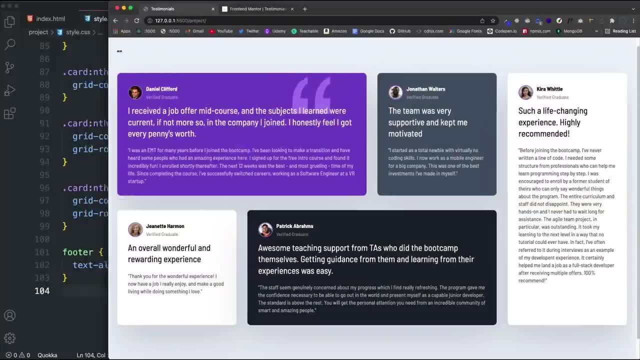 Okay, It should look similar to that- Awesome. Now, the last thing I want this to do is stack on small screens, because if we make this really small, then you know that obviously doesn't look good. So let's, let's do that. 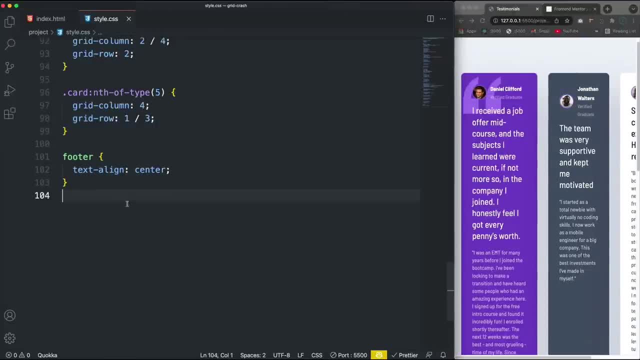 Let's add a media query So say, uh, I'll just do seven, 68.. So at media max with seven, 68 pixels, Okay, Okay. And then for testimonials, which is the container, we'll set the grid template columns, just to. 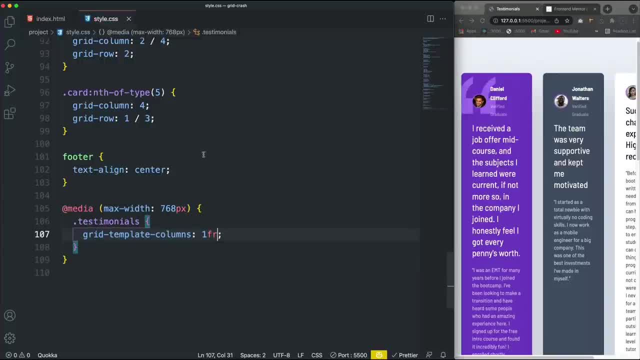 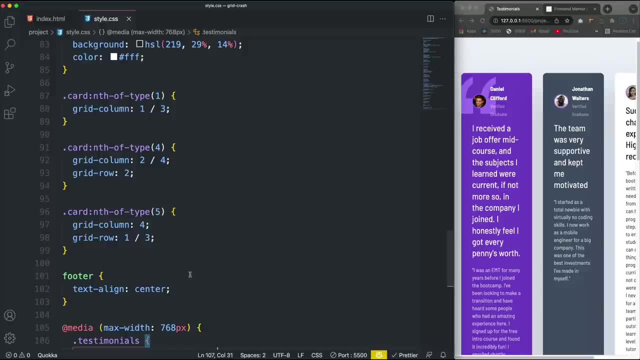 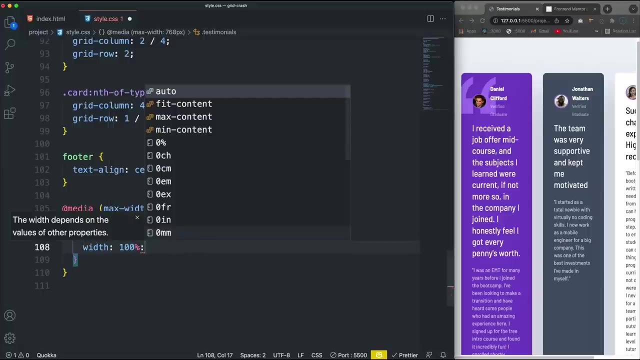 one fr. Now, that's not going to be enough, because we have the spans going on. So, basically, when you, when you want to stack them and you're doing this kind of thing, you have to reset them. All right. So let's go, um, let's set this to with 100%. 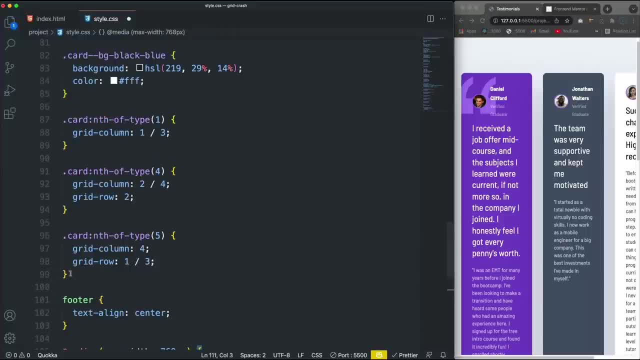 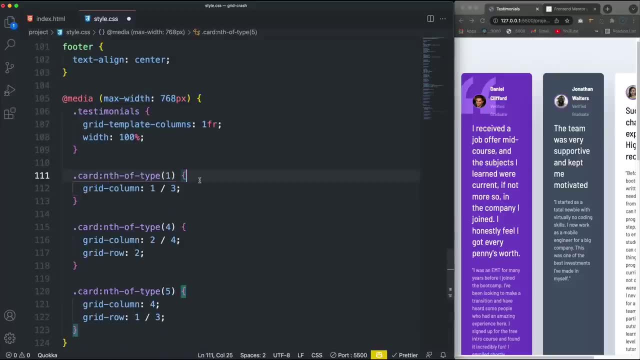 All right, All right, And I'm just going to copy these three and then we just need to reset and let it know where we want these to go on smaller screens. So for the first one, that's pretty easy. We just want it to be at one. 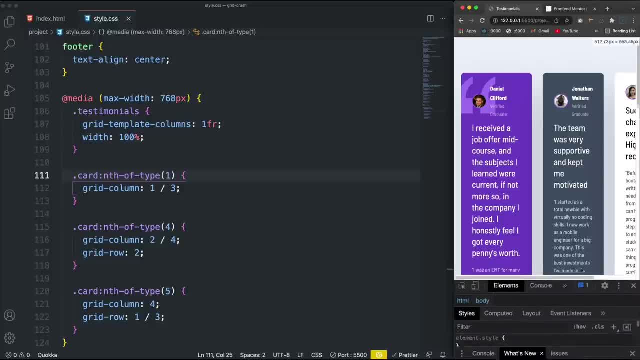 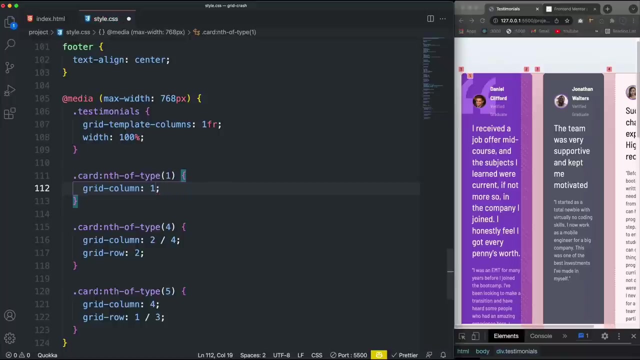 I should probably show the numbers here. for some reason They just disappear sometimes. All right, So we want this one to just As far as the column goes. So this way just one to two instead of one to three. So here we could do one slash two, or we can just do one. 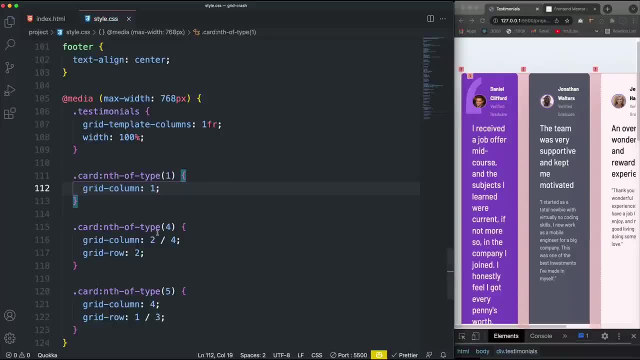 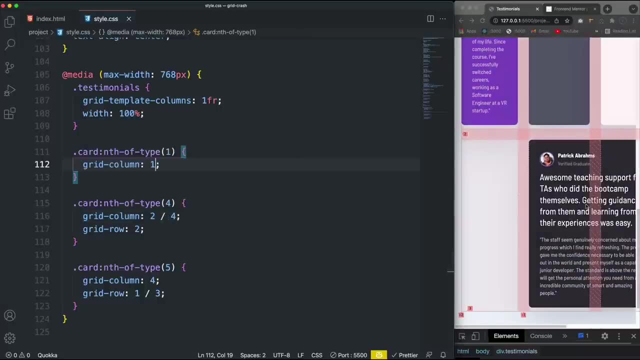 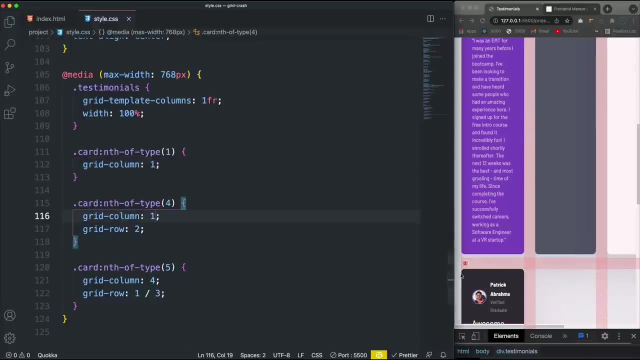 Okay, So now, yeah, you can see that goes to one, to two. Now for four, which is Patrick, who is way down here. we want, as far as the column goes, to be one. Okay, So column is going to be one. 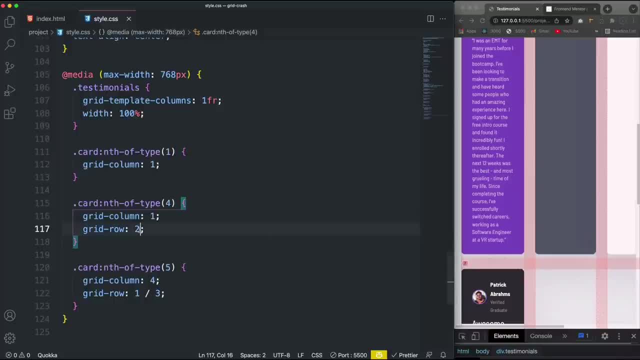 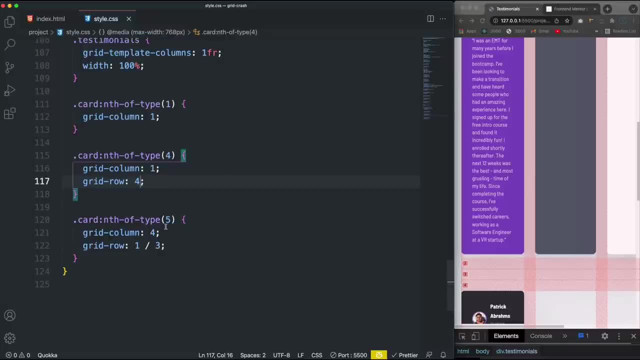 And then for the row: Okay, The fourth one. So let's set the row going from four to five, right, Or just four? And then for the fifth, one grid column again is going to be one, because it's just one column. 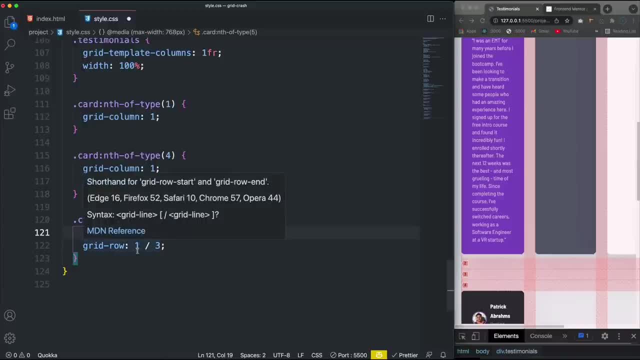 So they're all going to be one to two, And then, instead of going from one to three, as far as the row goes, she's the fifth one, So she's going to go from fifth to six, or just five. Okay, So now, yeah, we have Daniel. 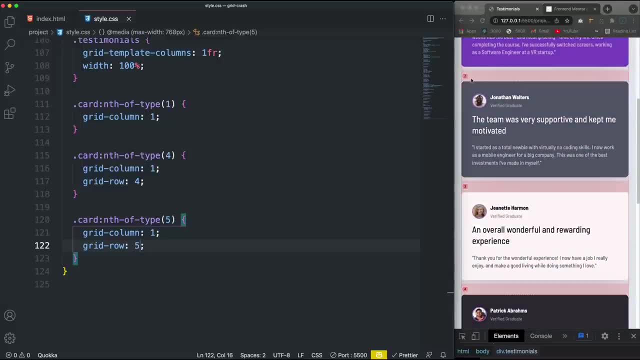 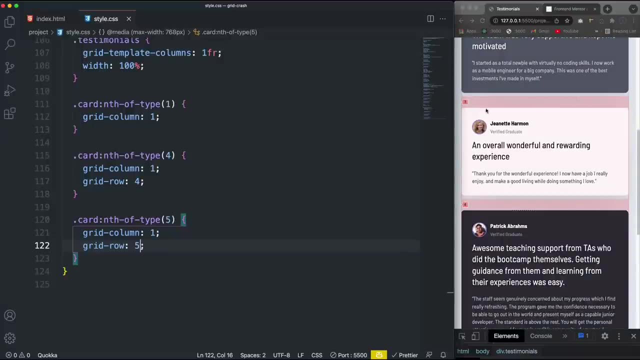 So he's going one to two, one to two, Jonathan's going two to three, one to two, Jeanette is one to two, three to four, Patrick is one to two, four to five and Kira is one to two. 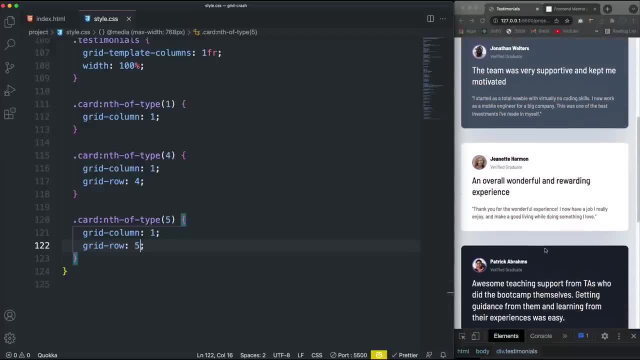 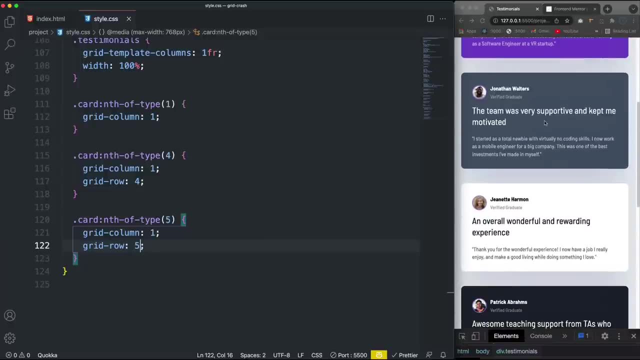 five to six, All right. So hopefully that makes sense And it can be a little frustrating to you know, figure out for for media queries, to figure out where you need to reset them so that they're in the right spot, You know. 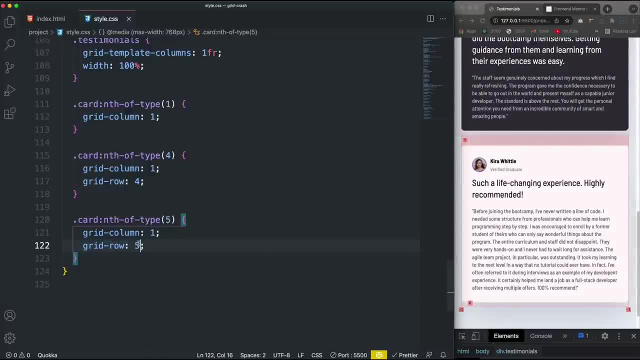 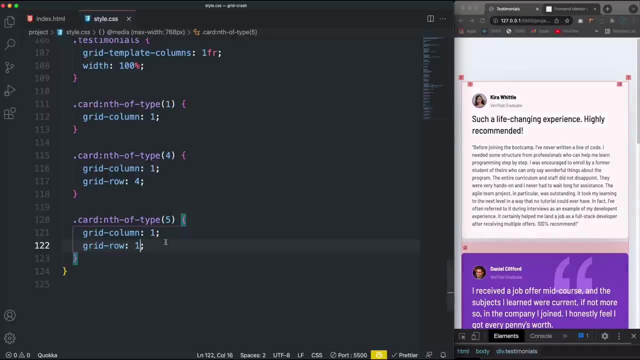 Unless it doesn't matter the you know where they fall, because you could set five, which is Kira to like one, and now she's at the top, All right, Which is actually kind of cool that you can switch around the order as well and not touch. 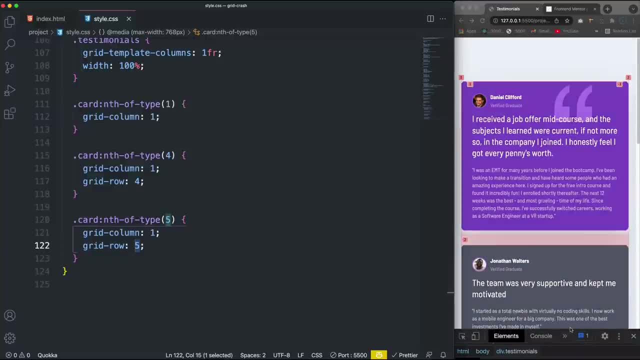 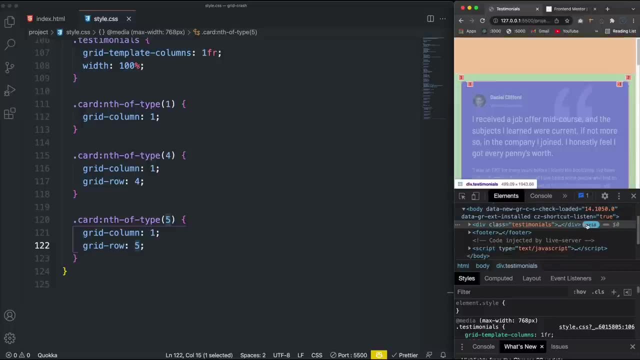 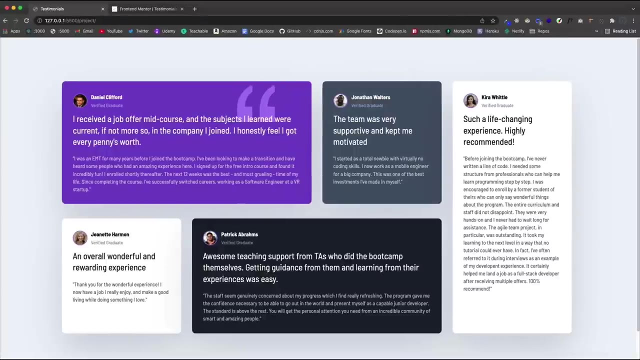 the HTML. But uh, but, yeah. so I think that that looks pretty good. Let's shut this grid, uh, grid thing off, All right, And yeah. So once we get to 768, we get our layout Cool. 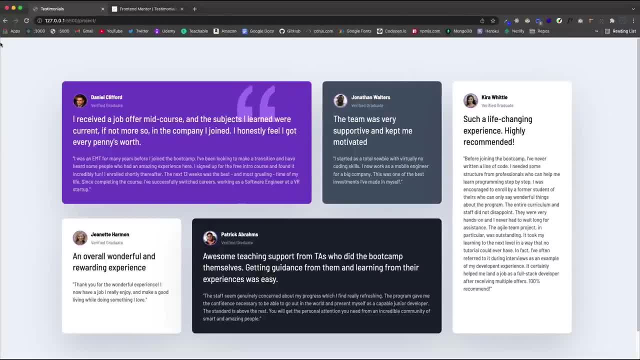 So I I really hope you guys enjoyed this and learn something from it and have some- you know, some- foundational knowledge in CSS grid. It's probably going to take more than just this one video for you to be comfortable with it, So I would suggest looking for some more uh project based tutorials where where you can. 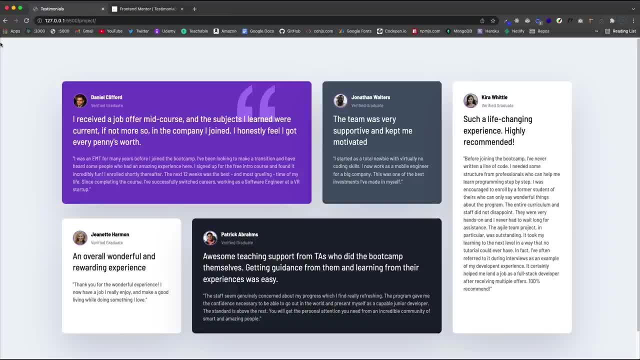 use the grid, All right? Thanks for watching, guys. I really appreciate it, Especially if you watch the whole video. thank you so much And I will see you next time.